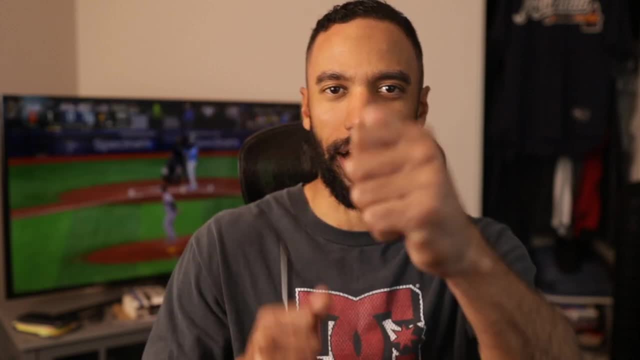 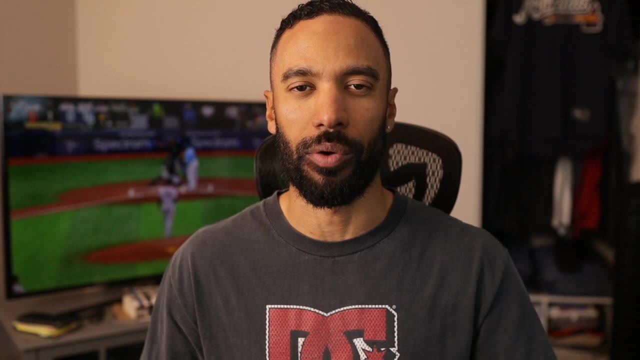 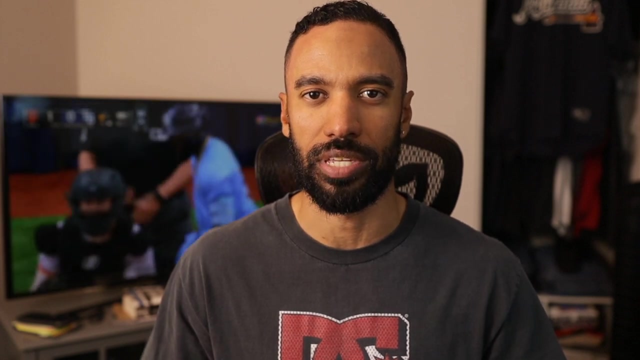 Well, hello and welcome to YouTube, to Mr Robinson's Q&A Power Hour straight out of the shower, where I am going to take my students' questions that they asked on right triangles and trigonometry, something where we've concluded this unit. If you've been following my video series, The Big Idea is Math Integrated Math 2 textbook. this would be stuff from chapter nine, So I'm going to take their questions and I'm going to attempt to answer them the best that I can. 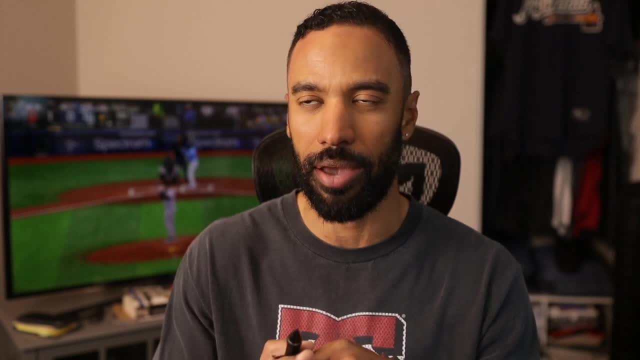 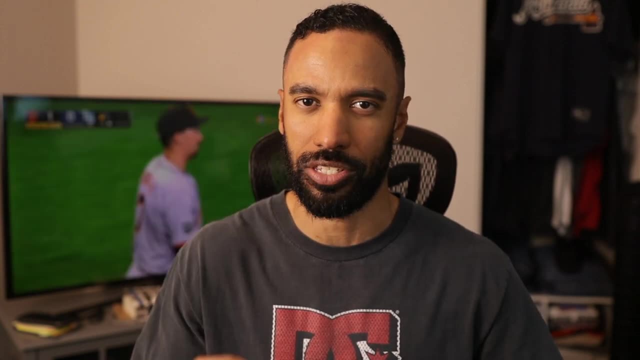 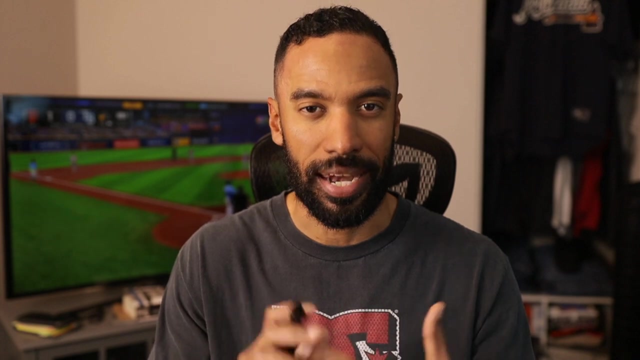 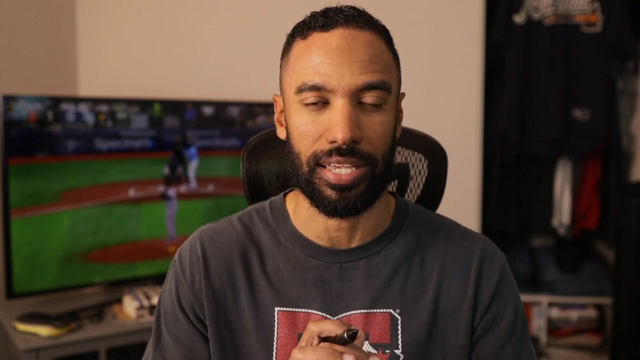 Nineteen questions were asked and at a time I was thinking of taking and consolidating them into like 10 questions as a whole, just like a lump sum of like whatever they were asking AskChatGPT to do it and make 10 questions out of it. But 19 isn't very many in comparison to what it could be, So I'll try and keep it within an hour as well. I haven't really read the questions. I imagine a lot of them are going to be asking trig related things, because that was the last three sections of that particular chapter. 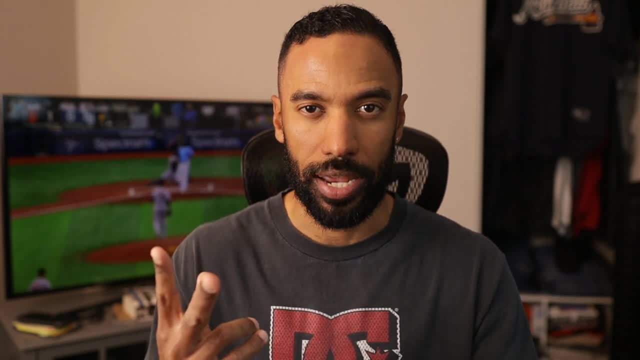 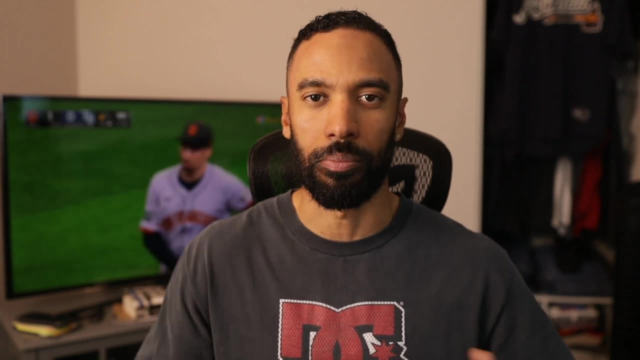 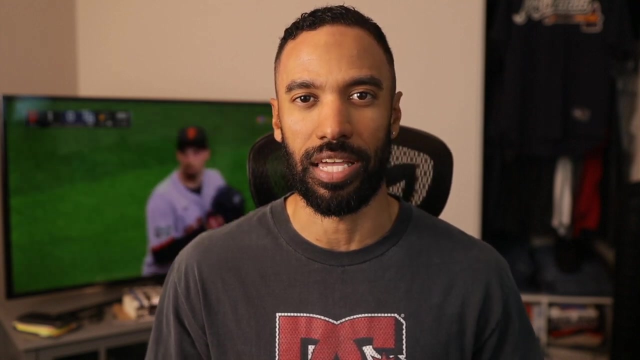 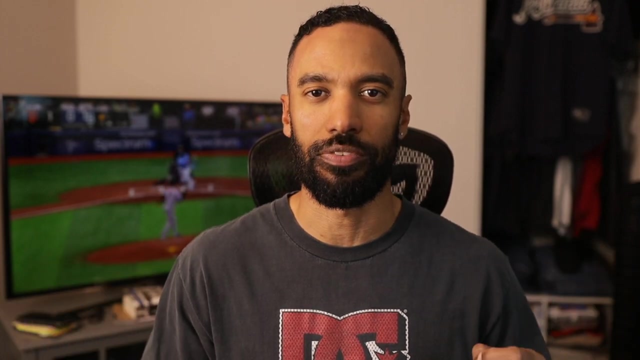 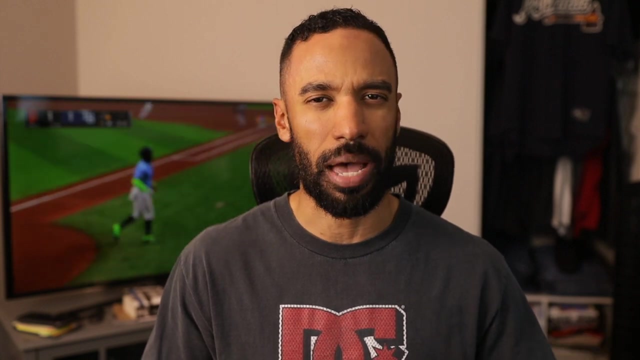 But if you want to know what else there was, there was Pythagorean 3.. Theorem: special right triangles: the 36, 90, 45, 45, 90 triangles and right triangle similarity, where you have an altitude drawn in a right triangle and then boom, three similar right triangles are made. I don't know what kinds of questions they're going to ask with that. If they do, I kind of hope that they ask some and they found a way to ask them so I can answer them for them. Anyway, check the description section down below if you want to find timestamps to each question that is asked So you figure out what kind of question you'd want to get answered. There may be repetition in questions and if there are, I'll just say I answered that before. 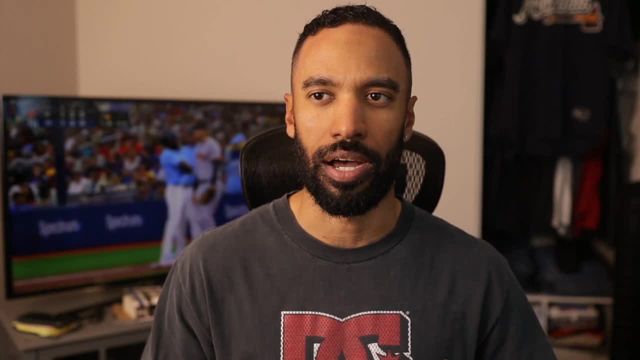 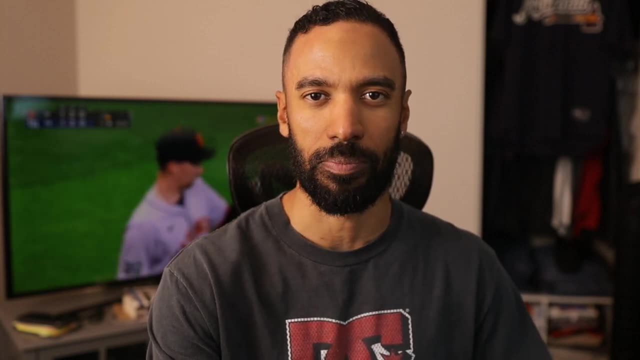 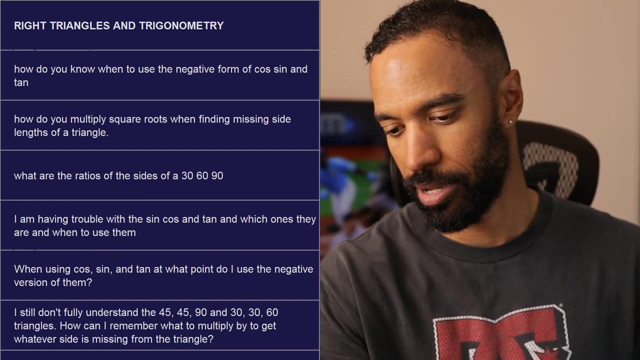 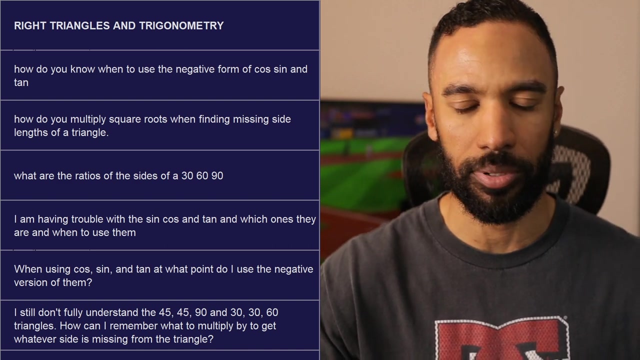 Kind of. Or? I answered something similar. Go find the one above, just to kind of save time and to not be repetitive, But let's go ahead and see what they came to ask me in this set here. Okay, so here we go. The first question asked- let me dim my screen a little bit- is: how do you know when to use the negative form of cosine, sine and tangent? So what I believe they're actually asking is about inverse sine, inverse cosine and inverse tangent. 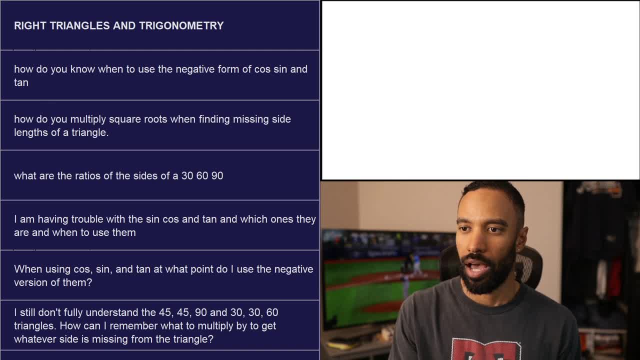 Because it has that negative appearance in them. They're talking- I believe that because I can't think of anything else that they'd be asking about- But this, where there's a negative right there, sine to the negative first power, right, Something like that, Let's just say of x, just for now, This kind of appearance, Okay, So this one, or cosine, or tangent, How do you know when to use it? Well, there are kind of two answers to it. 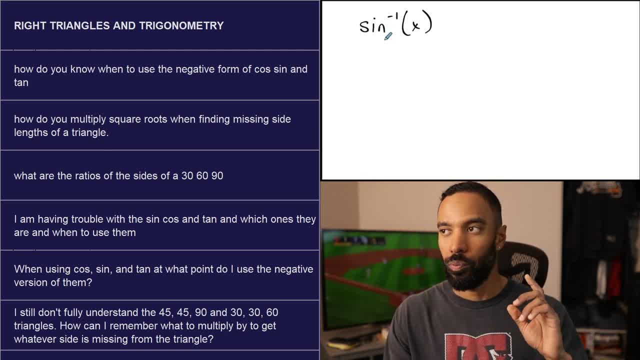 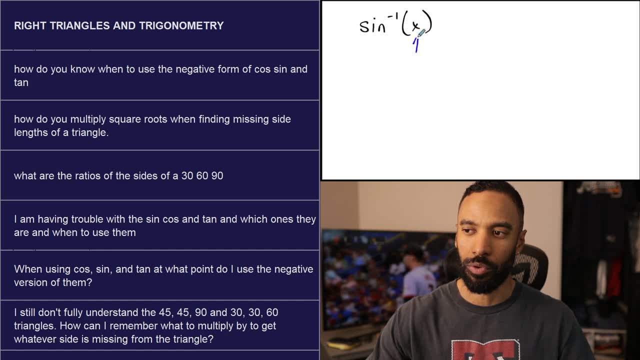 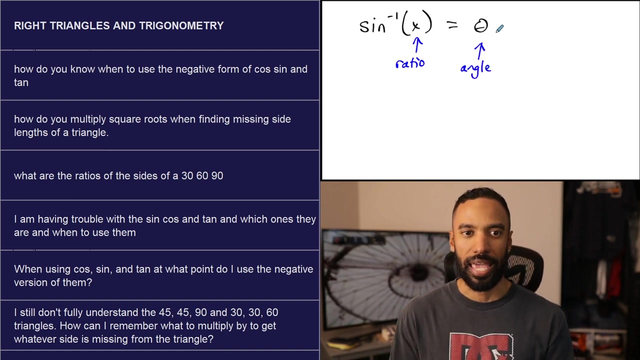 Number one. well, they're both the same answer, But we use it to get the angle measure of a value. This x, right here, is a ratio of the opposite over hypotenuse, whatever it is in your triangle. The result is some theta. that is an angle measure. We use it to get that angle measure. Now, when you say how do you know when to use it, you use it when you need to find an angle measure given a ratio. 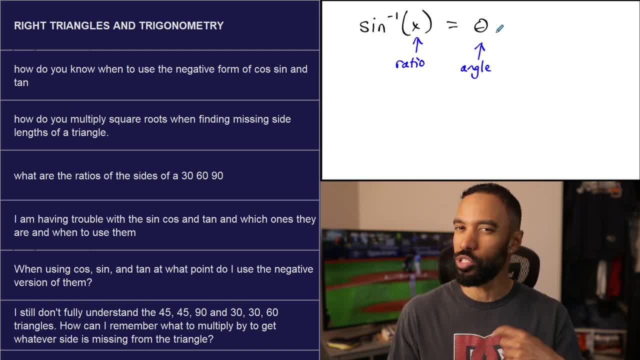 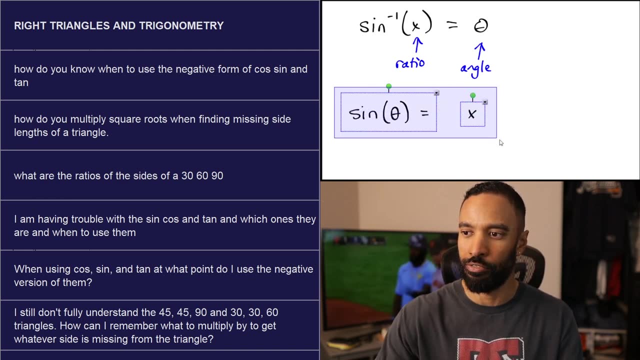 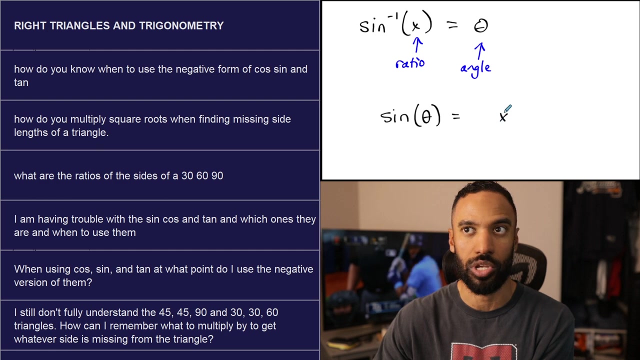 But in your particular case, you will know also when to use it, because you will have something that's set up as, say, the sign of an angle and it equals a ratio. And then let me get that spaced out a little bit more. And then your next step is: I need to solve for that theta. I need to get this theta by itself, because you'll have a ratio right, You'll have some number here. You're not solving for a number, The number is already solved for, But this is a variable still and you've got to find that. 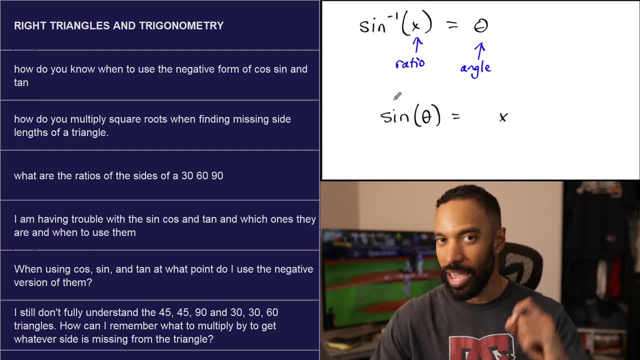 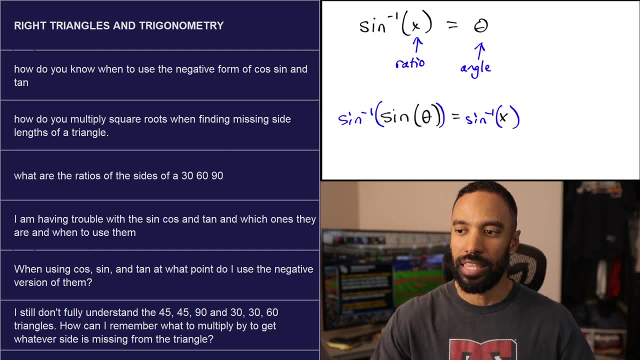 The way to get this by itself is to get rid of sine, And the way to get sine by itself is by using inverse sine of this side, And therefore you have to use it on this side. here The inverse sine of the sine of something is what cancels it out, And I've tried to stress very heavily in my class, probably in videos as well- in that, you know, some people suggest: oh, divide both sides by sine, which means very little because, number one, we're not multiplying by anything. 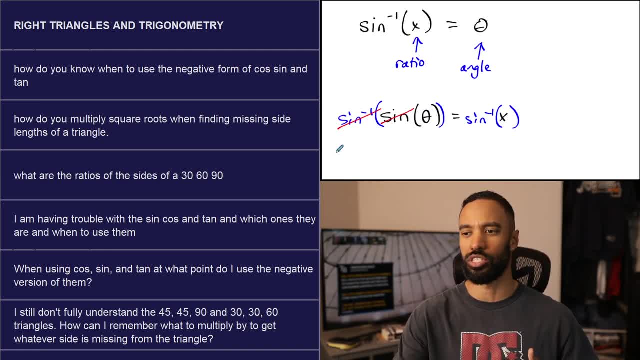 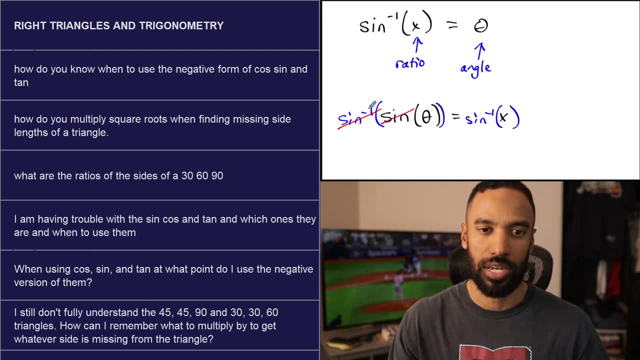 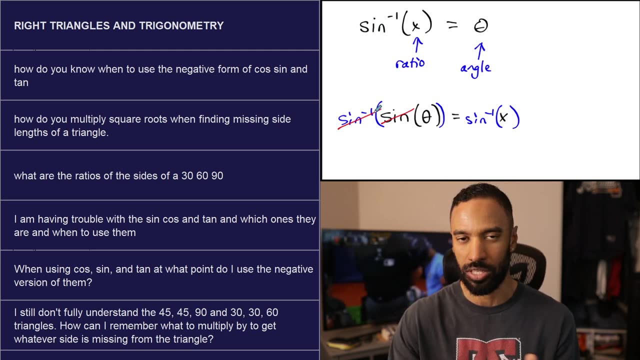 Number two: sine's not a number, It's a function, And you know all those things involved. But this particular function has an inverse called inverse sine, and that's what it looks like. So how do you know when to use the negative form of cosine, sine and tangent? I'd use sine very specifically here, but it doesn't matter, It can be interchangeable. If this says tangent, use, inverse tangent, things like that, You do it to find an angle measure And you know. therefore, now theta is now the inverse sine of something of that thing. right, And I wrote that up here as well, To give one quick example of that, we have some theta right here. 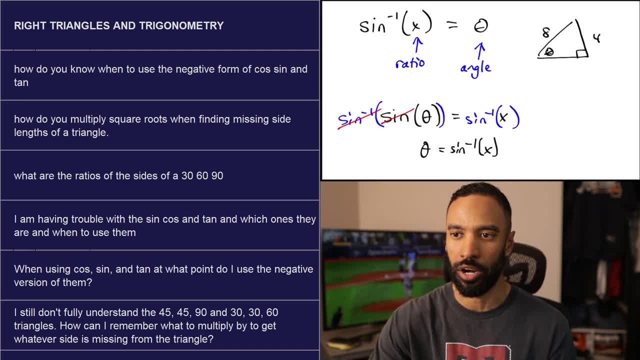 And this length is four and this length is eight. Actually, I don't want to use something that I know the answer to This one's five and this one's eight. right, So we can say: all right, I'm going to set up an equation that says the sine of my angle equals opposite over hypotenuse, five over eight. Now I take the inverse sine of both sides, which cancels out the sine on the left side and gets theta all by itself, And then you now have the inverse sine on this side, And the inverse sine of five eighths is some number. Actually, maybe I should have used the four eighths, because I'd know what that number would be. It would be 30 degrees. Why don't you? 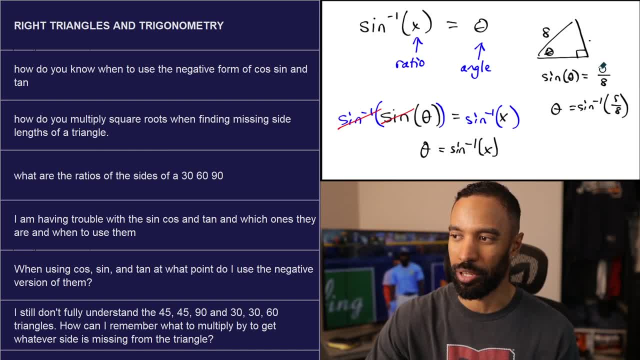 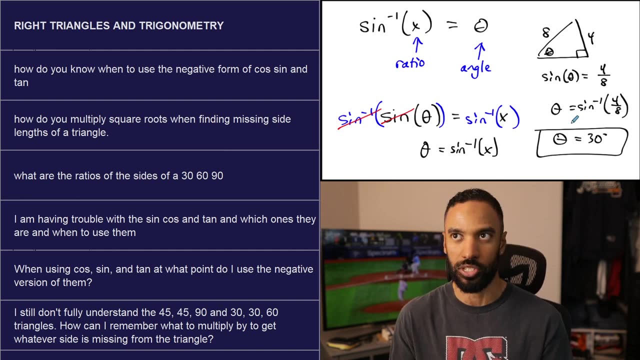 try that if you want to. So let me bring the four back. This is clearly unplanned. Yeah, if you had a four right here, four over eight, I happen to know that this one will be exactly 30.. You can use your calculator and check that one out. But yeah, you use it to find an angle measure right? That's the point. It's not the negative form, And I think that's the other thing I want to address. It's not the negative form of it, It's the inverse of them. You use it to invert what you have. It's like saying: how do you know when to use division? Well, it's the inverse of multiplication. So you use it when your variable 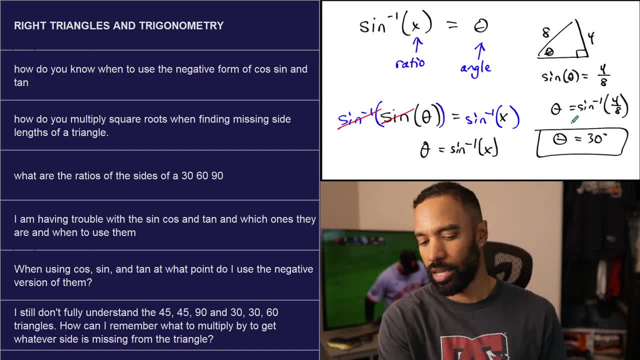 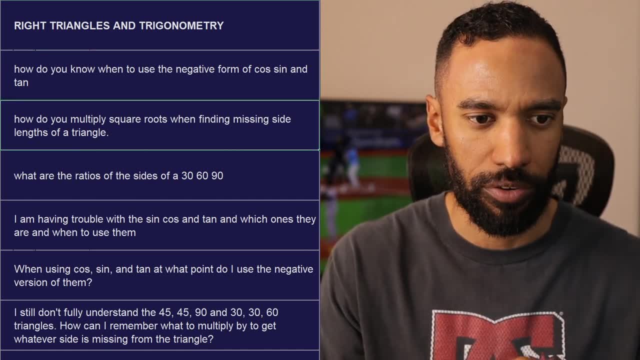 is being multiplied by something that you want to get rid of- Stuff like that. All right, there's that question. Hopefully that is answered. well, Let's go to the next one that asks: how do you multiply square roots when finding missing side lengths of a triangle? Let me start up a new thing here. 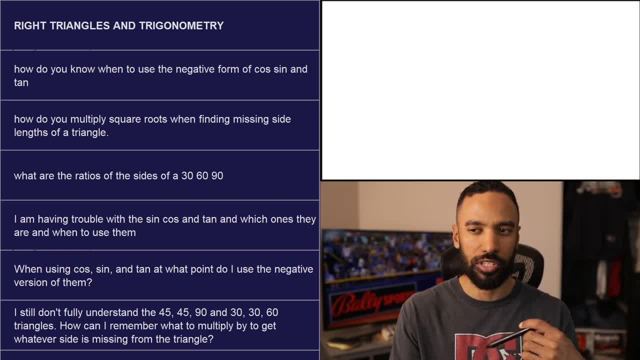 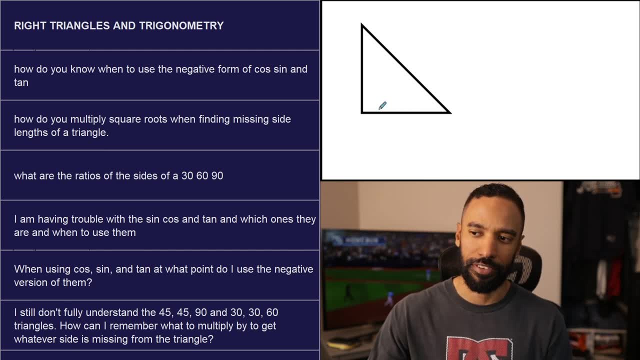 Square roots meaning. so I think we're talking about the special right triangles. So let me get an actual right triangle here drawn, So like in a 45,, 45,, 90 case. you know, here their ratio relationship is 1 to 1 to root 2.. So that means that whatever this length is right, 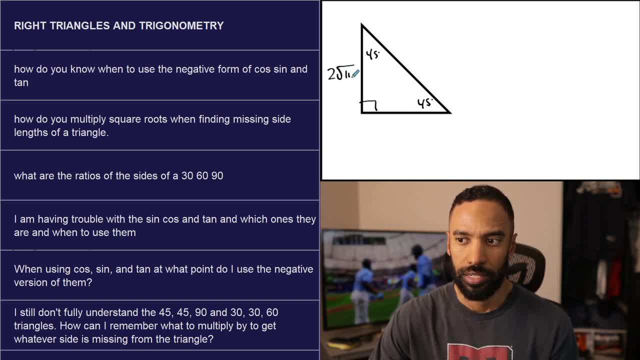 here. let's say it was 2 root 10, that I wanted to find out what this x was right here. So this x is going to be root 2 times larger than whatever this guy is. So x is 2 root 10 times root 2.. 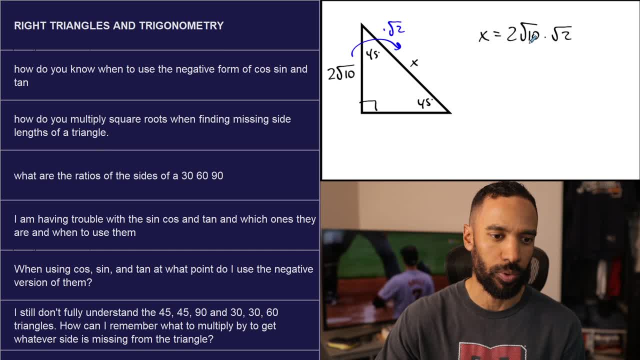 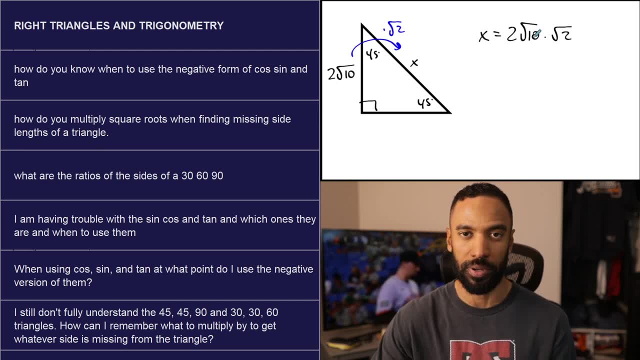 Now the question asked is: how do you multiply square roots when finding missing side lengths? So I mean, this isn't new for us, the 45,, 45,, 90 is, but not this actual simplifying radicals concept: Square roots multiply with square roots. The idea of the property is: and this works both. 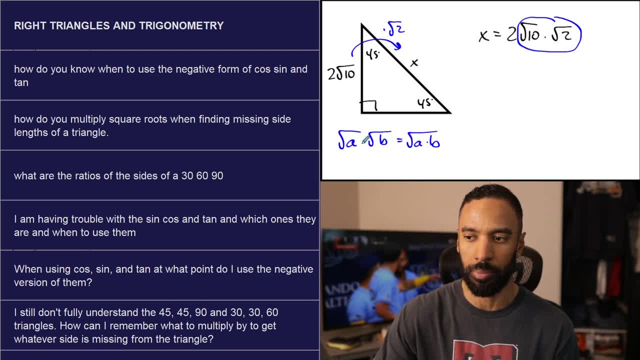 ways- this also works to simplify radicals, which we'll get into in this very problem- that you can merge these two under the same square, what I call square root hat, Or if they were cube roots, then they can go under the same cube root hat together. 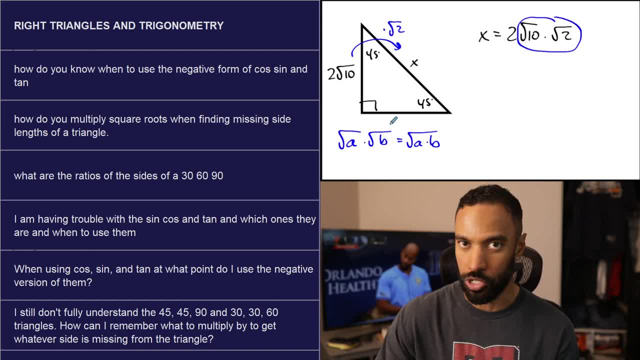 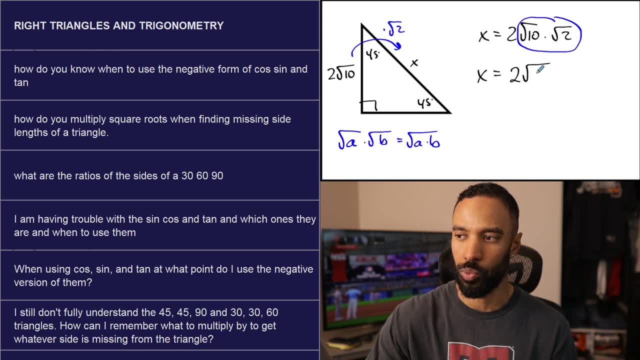 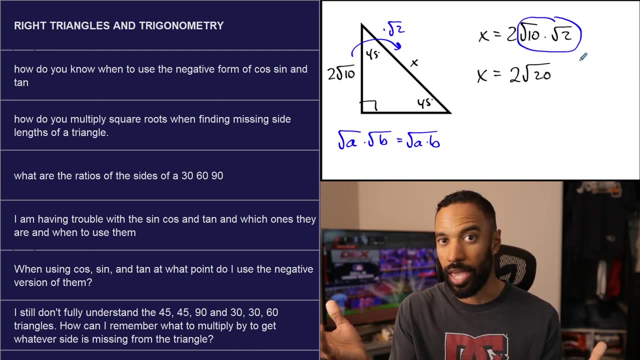 things like that. This is a property that's true for multiplication and division of radicals, of irrational values. So root 10 times root 2 can multiply together and you'll get root 20 as an example. Now that is how you multiply them. So you only multiply them together if they are square roots together. 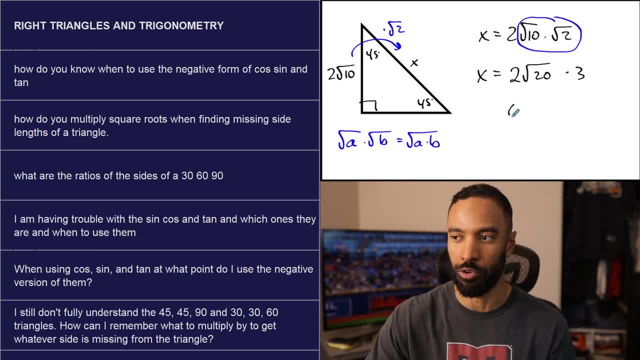 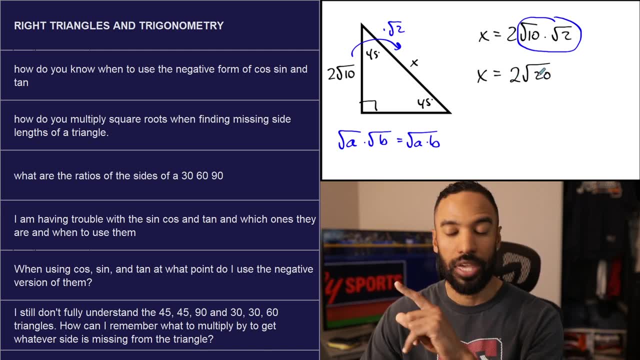 I hope that makes sense. And then if there was like a times 3 right here, then it would be 6 root 20, whatever like that. Only the rationals multiply with rationals, irrationals with irrationals, things like that. Now this would still have to simplify as a radical, because it 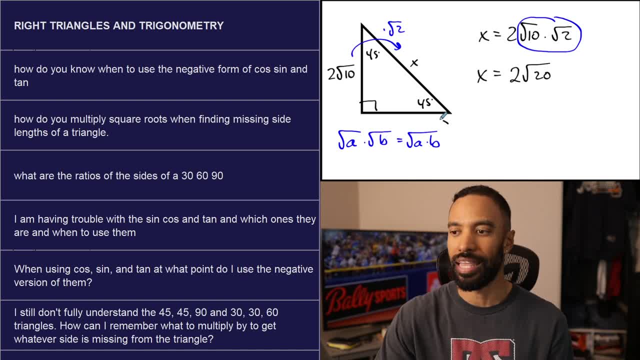 contains a perfect square factor, which brings me to my next point- that this works this way as well. 20 is a product of two numbers, not just 2 and 10, but also 4 and 5.. And I bring up 4 and 5. 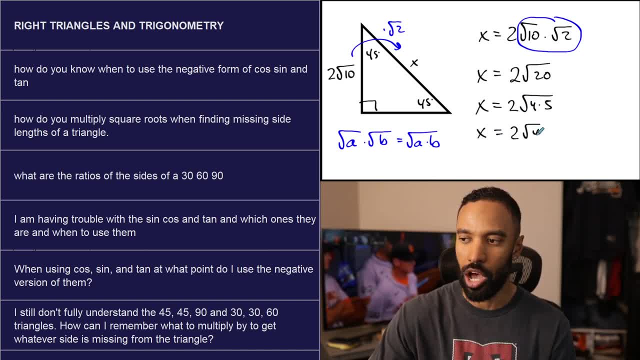 because 4 is a perfect square and that I can get it in its own square root. Own square root 5 gets in its own square root and I can therefore take the square root of 4 and get 2.. And this 2. 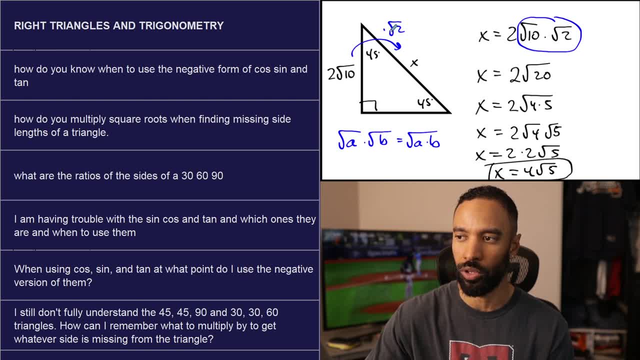 multiplies by this 2, and you get 4 root 5.. Obviously, I'm going longer in the problem than perhaps need be, But that is the idea that you can multiply by 4 and 5. And that's the idea that you 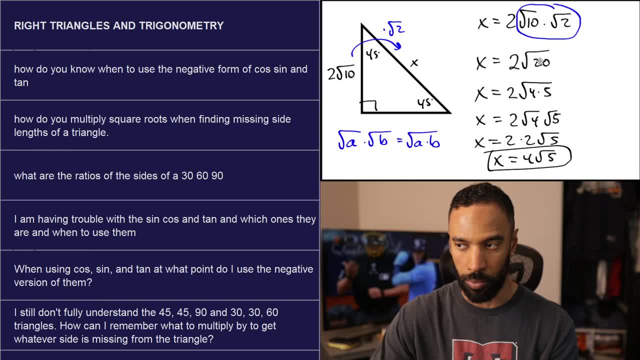 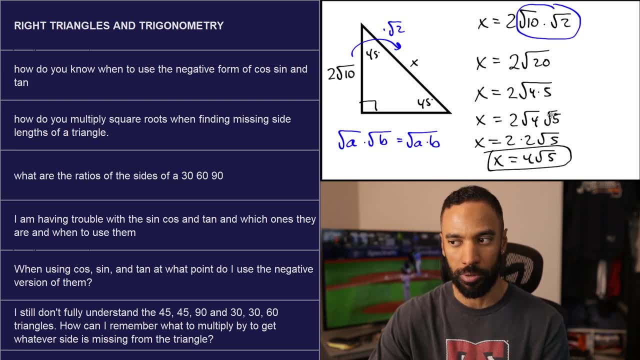 multiply things together, fuse the square roots together to become a single square root of something, And likewise, when you simplify a radical, you factor out any perfect squares because they can go in their own separate square roots as a product. in the same way, 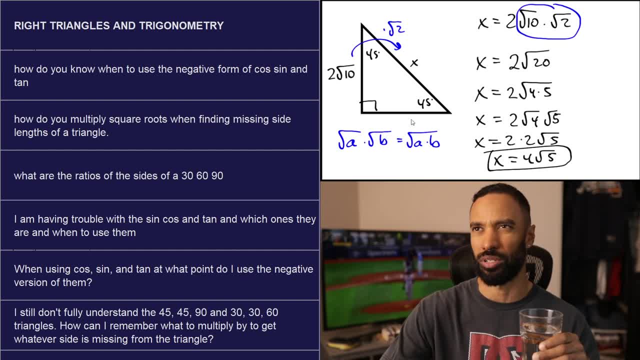 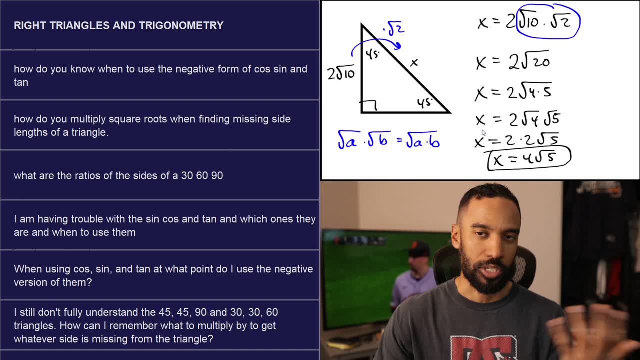 This is interchangeable, It goes both ways. We've been using this since chapter, I think, 4.. If you've been in the integrated math 2 set, I'm not saying you can't ask the question, I'm just saying that it's not new. for that All we now have to know is what are 30,. 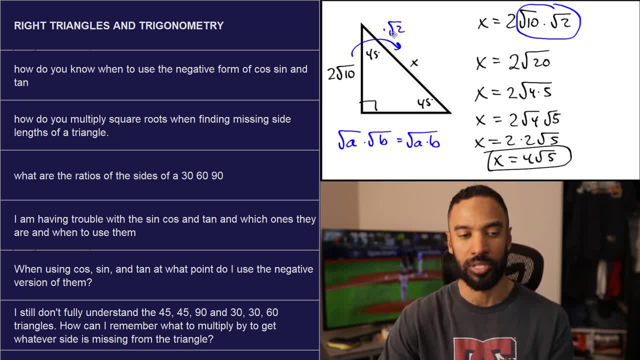 60, 90 ratio relationship is. What are 45, 45, 90 ratio relationship is Now? you didn't ask about dividing. You didn't ask about dividing and I'm not going to answer it in detail unless I see the. 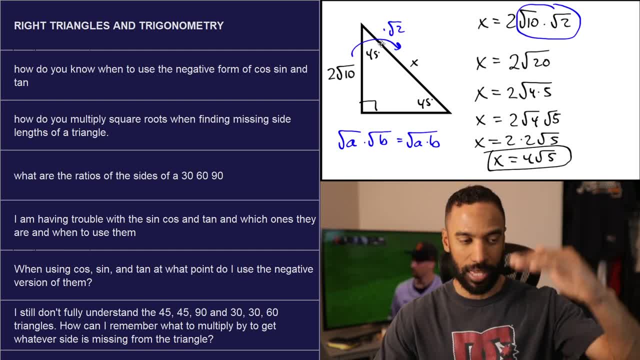 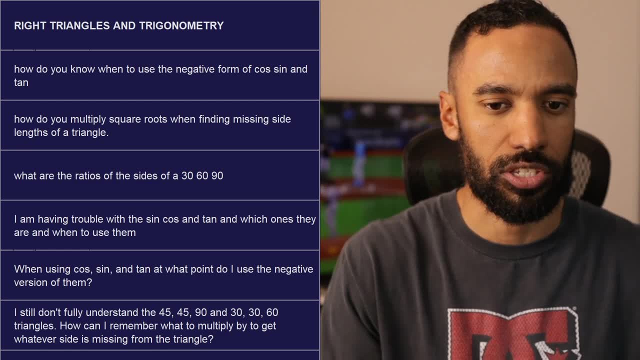 question, but it has to do with rationalizing the denominator. Yes, they can divide, but if you ultimately have a square root still on the bottom, you got to take care of it in some way. So we'll see if a question is asked about it or ask me in class, All right. Next question is: what are the 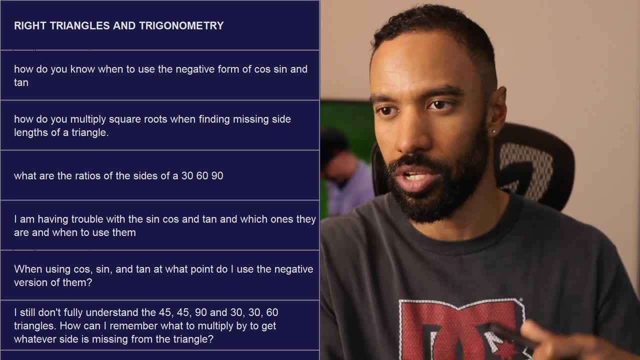 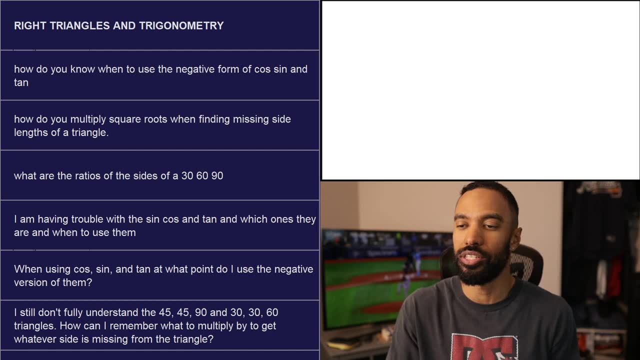 ratios of the sides of a 30,, 60,, 90? So I guess that this carries on So far. I mean, two or three haven't been asked about trig, so I didn't know to expect that. So the 30,, 60, 90 triangle, I just 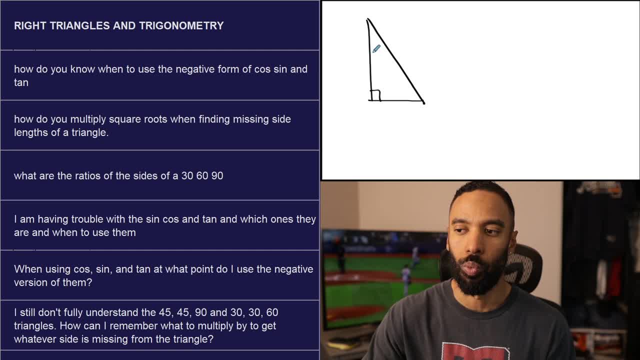 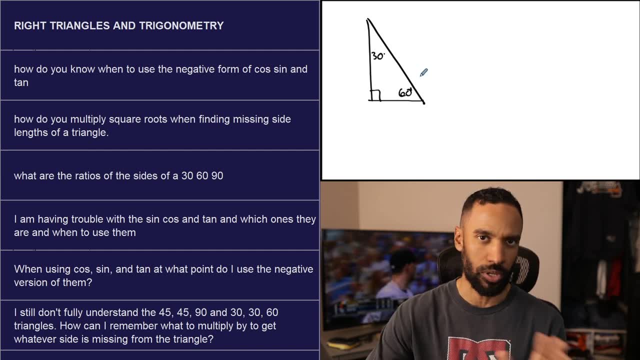 mentioned in the last one. the 45,, 45, 90 triangle is one to one to root two. Now, my students should have taken notes on this kind of stuff. They can obviously look it up at any time. I'm fine. 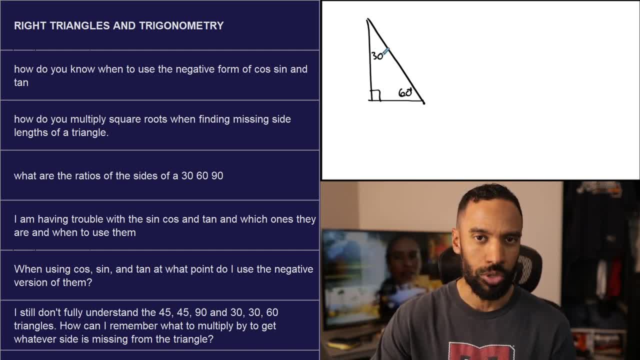 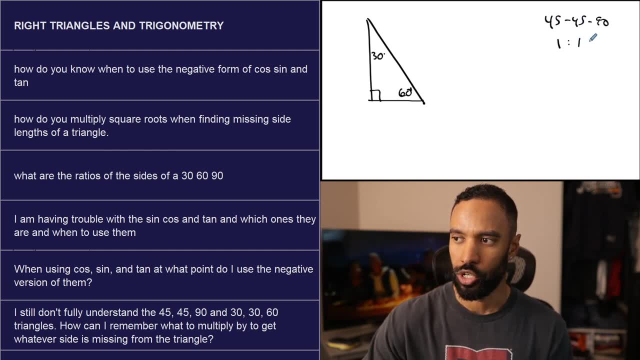 answering it though, but I just want to mention how you can remember this in some sort of way. First of all, the 45, 45, 90 has the one to one to root two ratio relationship. We know that one plus one is two. I'm not saying that that is something you'll mathematically have. 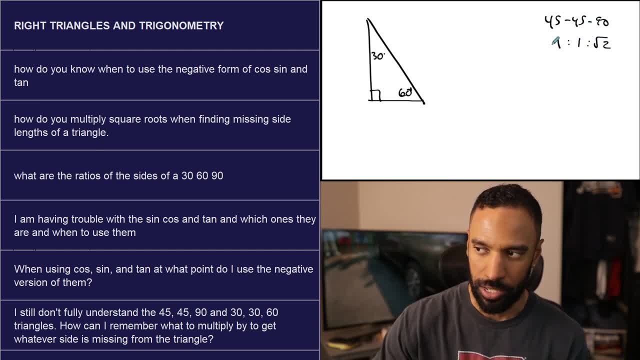 to deal with in this. I'm just saying that's a way to remember those numbers. I guess Also Pythagorean theorem: one squared plus one squared is root. two squared, The 30,, 60,, 90 is one to two. 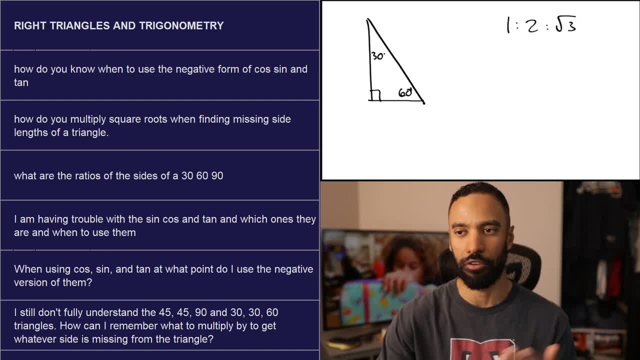 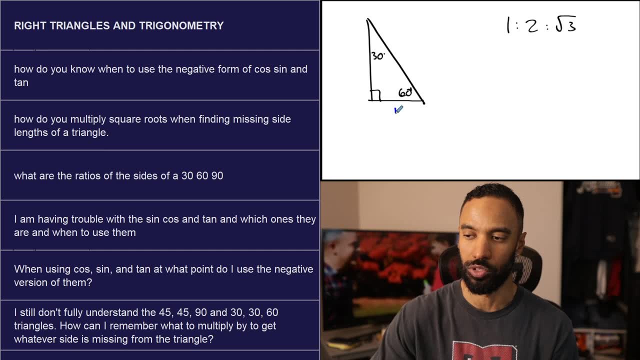 to root three. It's one to two to root three. but you got to be careful as far as where they go Opposite. the smallest angle should be the shortest side. One is smaller than either two with a square root of three, So this will be a one right here. Now that doesn't mean the number's one, It means 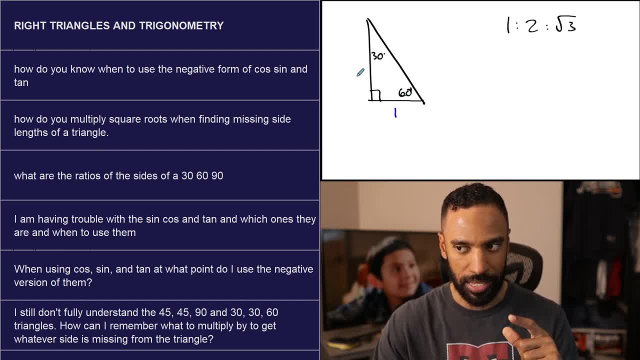 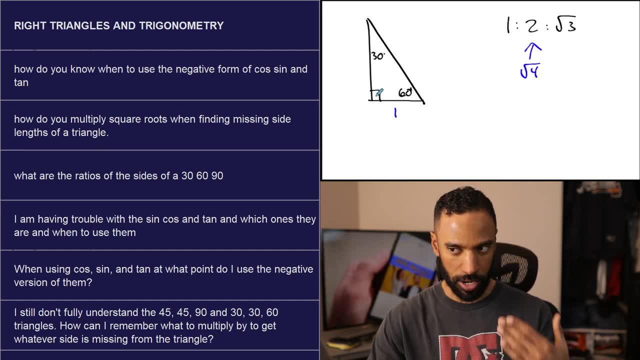 whatever this number is, we can multiply this by a certain amount to get this and this. Now, what number's bigger, two or the square root of three? Well, two is the square root of four, and opposite, the largest angle should be the longest side, So root four or two should go here. 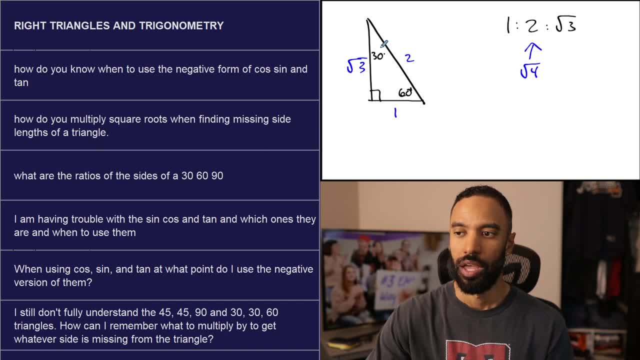 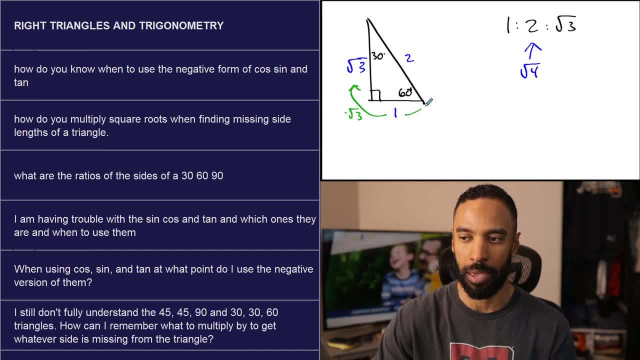 and the root three should go here opposite the 60. What this means to us is the short leg of the one. I can find the long leg by multiplying by square root of three, or I can find the hypotenuse by multiplying by two, And likewise I could get to the short leg by dividing by two or dividing. 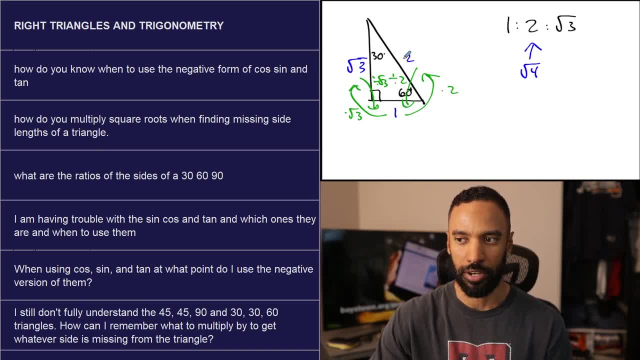 by two. So that's what we're going to do here. So we're going to get to the short leg by dividing by root three from these places, And I'd want to go from the long leg to the hypotenuse by going to the. 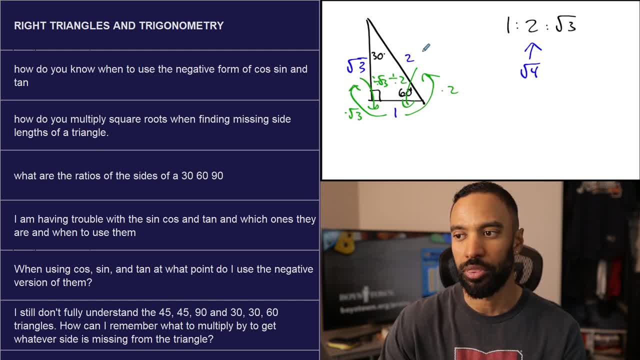 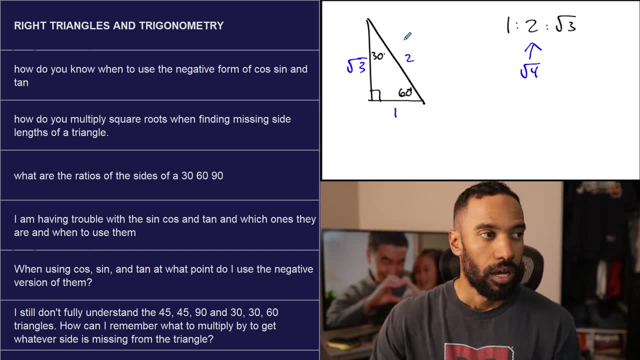 short leg first. So if you see it in my examples you'll know exactly what I mean. But those are the ratios. I won't dive into a proof right here, but it has to do with equilateral triangles. if you want to, I think I have a lecture video somewhere that dives into the proof stuff. So if you go to, 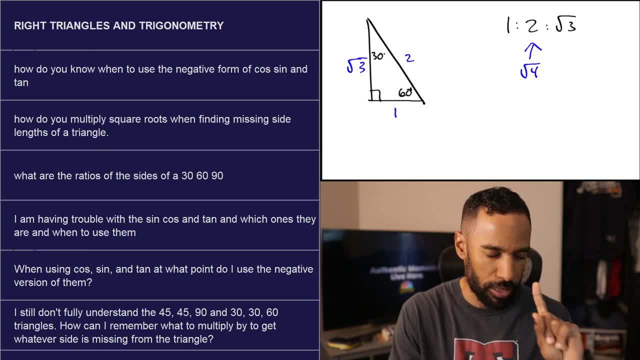 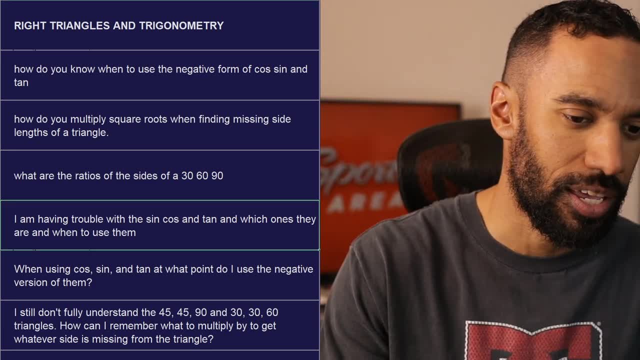 the 9.2 portion, find my lecture video, find the 36 and 90 triangle, you will see my proof on that exact thing. I hope that answers your question. Thank you for asking that. Next question is or statement. I'm having trouble with the sine, cosine and tangent and which ones they are, and 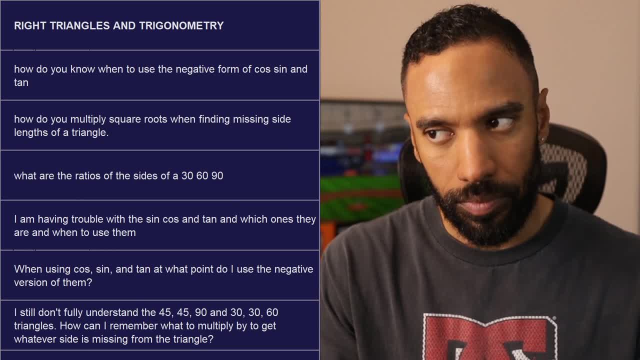 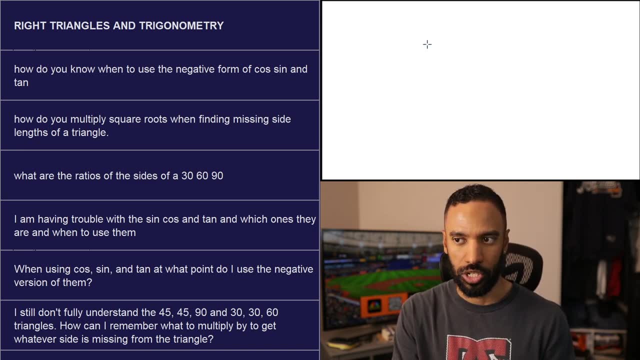 when to use them. There could be a bigger talk to be had. I'll try and condense it into something significantly smaller. Sine, cosine and tangent are each. there's no one that's better than the other. Like to just really hit home. no one's better than the other. No one's like well. 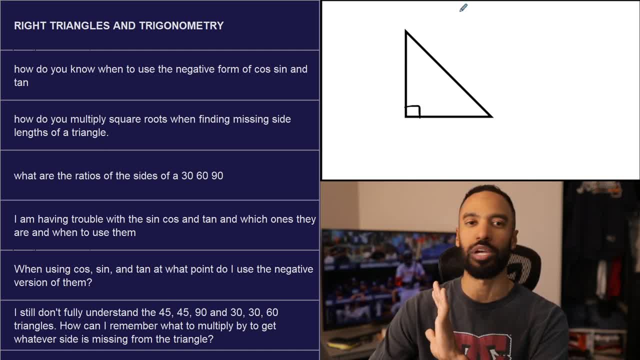 I really prefer this one. No, no, no, it's nothing like that. Everything's completely dependent on the angle to which you're referencing it from. So I'm going to go with the sine cosine and tangent. I'm going to look up the side of theta which are referencing. let's say it's this: 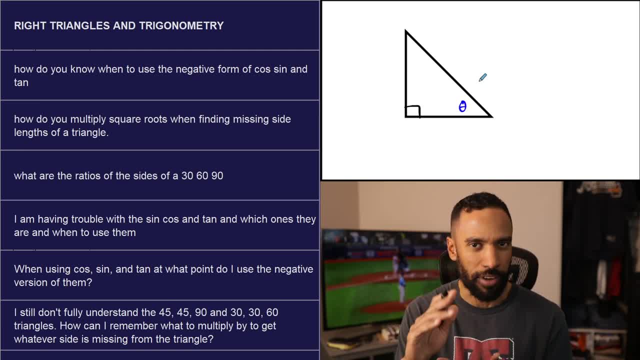 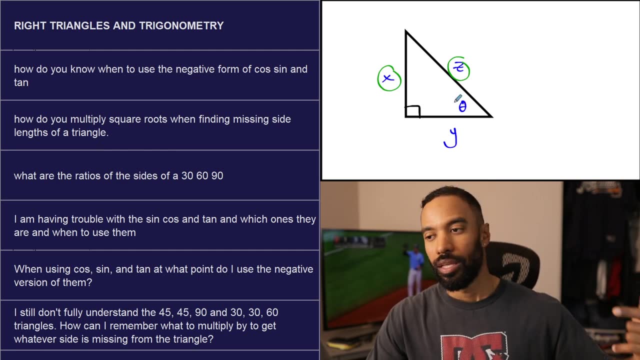 guy right here and which side lengths are known slash, labeled slash. you have to find If there's some sort of X, Y, Z right here, but X is the one that you need and Z is the value that you have in relation to theta. the side opposite is X and the hypotenuse is Z and therefore I will. 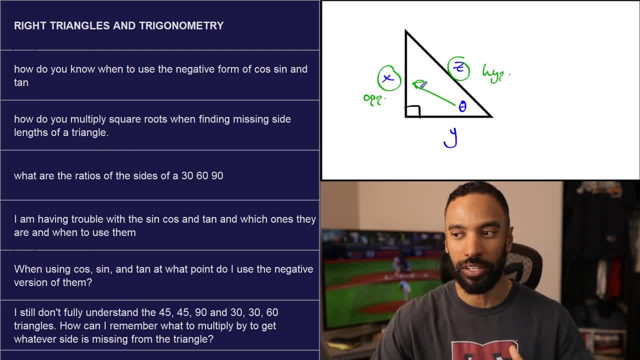 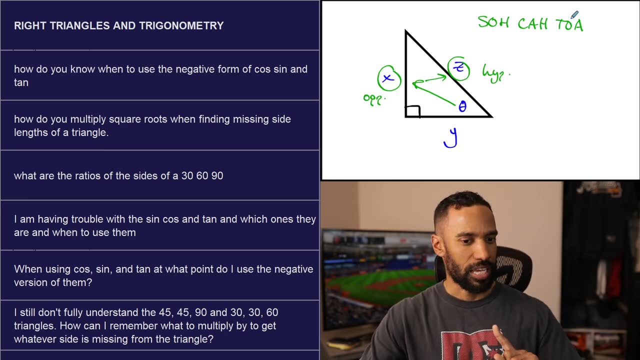 use sine. That function is specifically designed to understand that the opposite of hypotenuse ratio is what gets you this angle, the sine of the angle measure, because we remember that from SOHCAHTOA. So I'm having trouble with sine cosine tangent, which ones they are and when to use them. 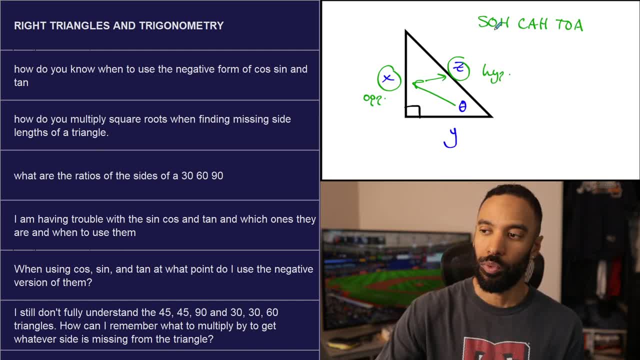 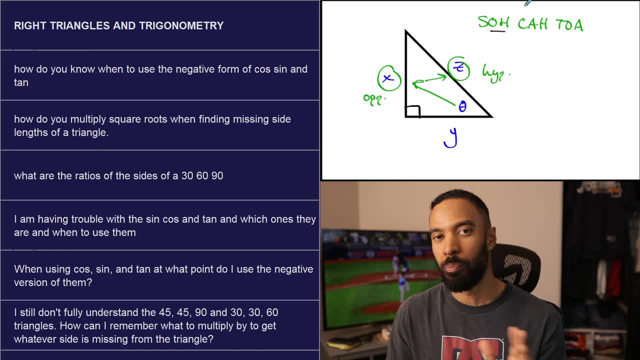 Remember how to spell SOHCAHTOA, That will get you a good head start. Sine uses opposite in hypotenuse. Now again, there's no one that's better than the other, or anything like that. Your calculator, as much as we're going to use it, your calculator is very aware that. 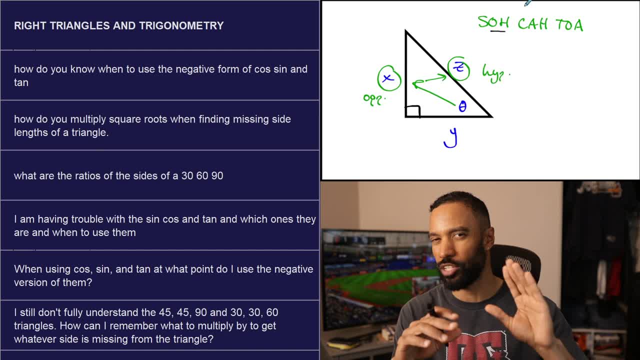 when you hit sine of an angle, it's dividing whatever that right triangle's opposite divided by its hypotenuse would be, because every right triangle with this angle measure is similar to one another- that this divided by this will always be constant. Remember when I said that if this was four and this was eight, if you heard earlier. 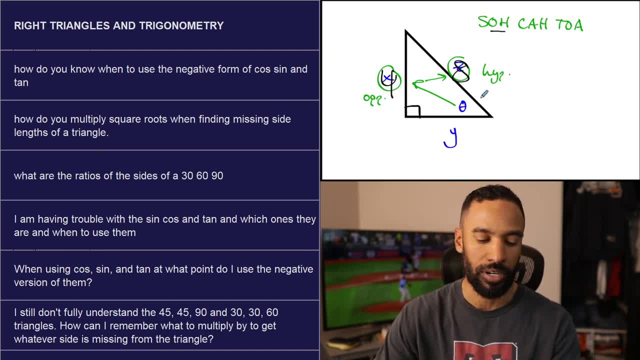 this would give you 30 degrees. It will always give you 30 degrees, Or you know, whatever the sine of 30 is always point five because, whatever this is, this is always twice that amount, like a 30,, 60, 90 triangle would. 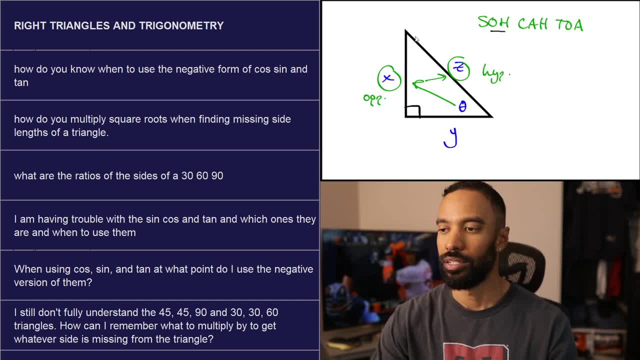 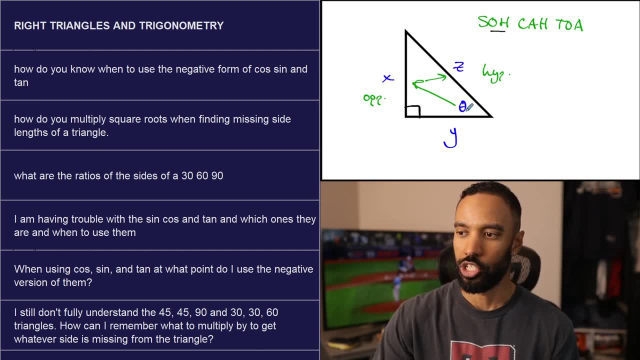 But that's what sine would always use. Now cosine. cosine would use opposite, excuse me, adjacent over hypotenuse. So the adjacent leg to theta is the Y variable. In this case this would be adjacent. And let's say you had that, or you were trying to find it, or you had the hypotenuse you're. 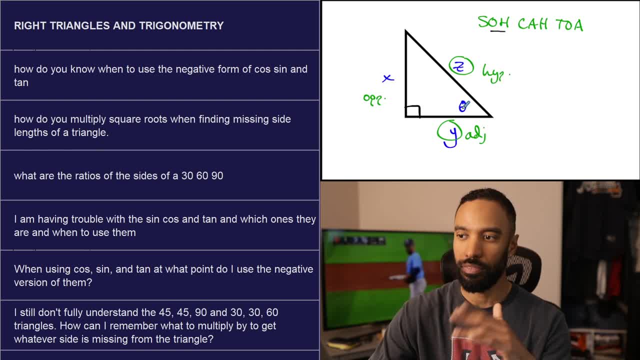 trying to find the hypotenuse, something like that. or you're trying to find the angle with these things labeled. Basically, if these were your three labels, you'd be using cosine because, relative to this angle, this is the adjacent leg, this hypotenuse. your calculator is very aware. 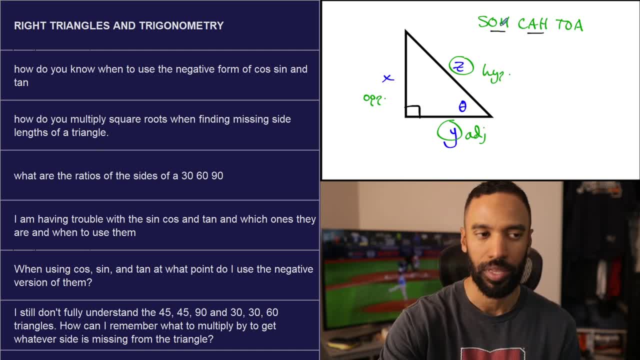 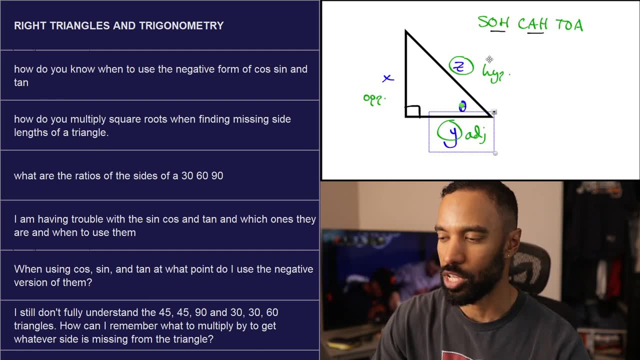 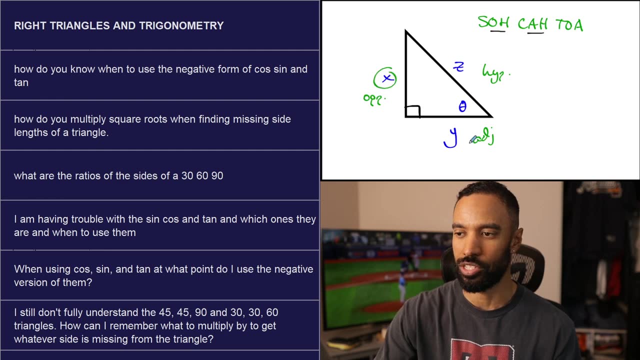 that those are the two things that divide when you use the function cosine. Tangent is opposite over adjacent. Whoopsie, I totally lost my stuff. There we go Tangent's opposite over adjacent. where ADJ opposite this angle is X, the adjacent is: 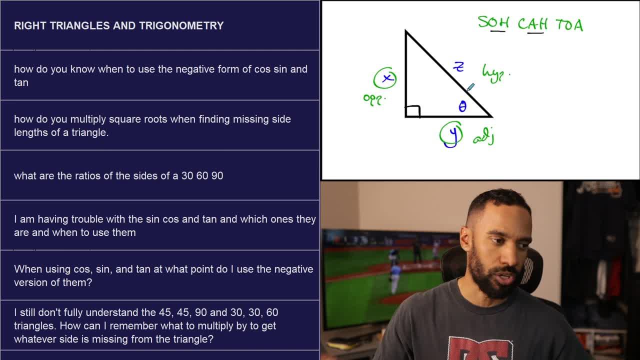 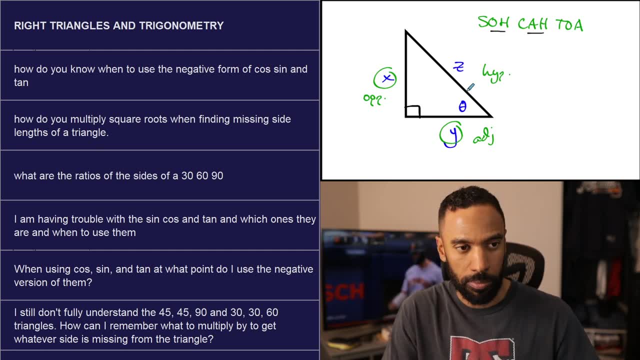 Y, it would divide those two. Get that ratio for you As far as what you need to solve for something. So I'm doing this very generically. I'm not using actual examples with this stuff outside of showing you where they are, but 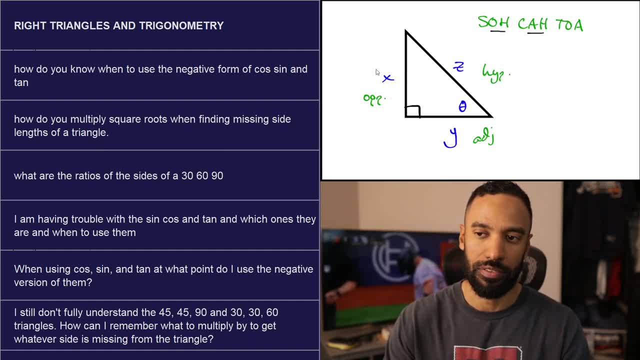 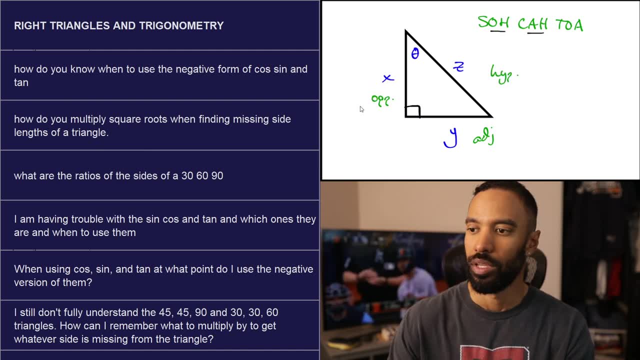 there's that Now. the other thing to keep in mind is everything is relative to the angle you're using. So this theta, if it was over here, this is no longer opposite. This is opposite is now on this side, like the Y, the adjacent is now the X. 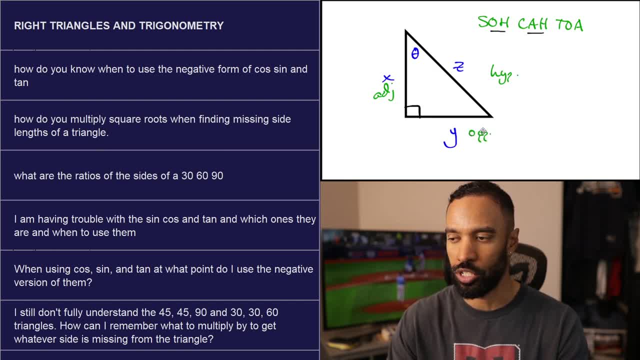 Hypotenuse is still hypotenuse, That won't change. But as far as opposite over adjacent or whatever, Theta now being here means we're going to use those and don't worry about the right angle one. We're always referring to the acute angles when we talk about it. 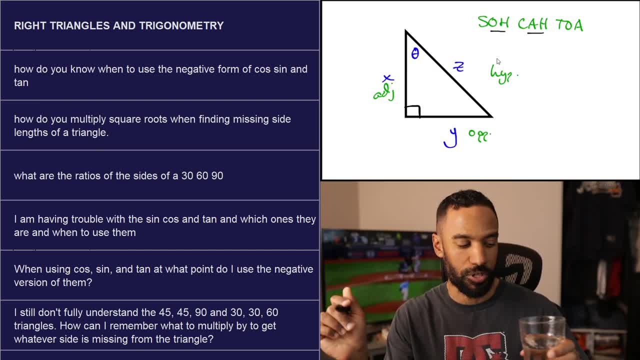 There's. there's a way to get sine cosine and tangent of 90 and your calculator will show you what they are. but you're not really talking about right triangles anymore. You're talking about unit circles, which means you're talking about IM3 or pre-calc. 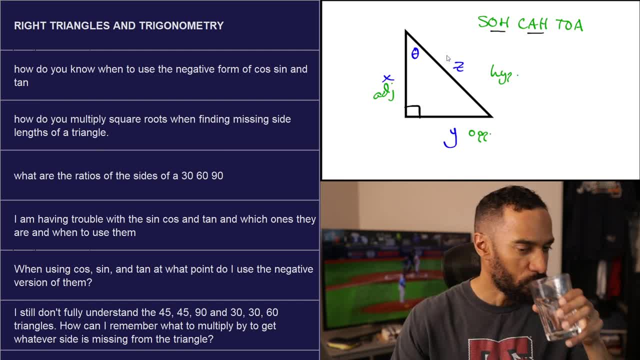 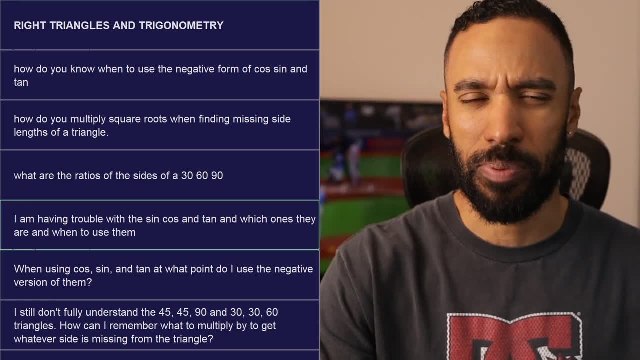 Only worry about the acute angles. OK, hopefully that answers your question there. Thank you for asking Next question. So yeah, I expect a lot of trade. but here we go. when using sine, cosine, sine and tangent, At what point do I use the negative version of them? 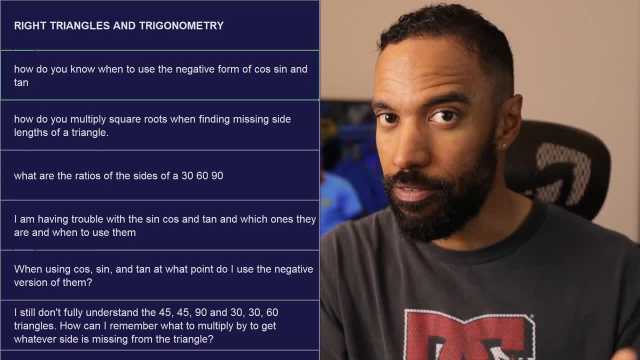 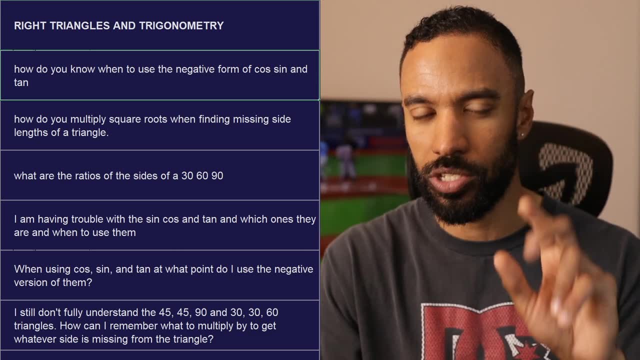 So I don't know if it was the same person asking with the first question up above. I'll just go ahead and mention I answered it up here, Uh, the one that I'll answer it very shortly here in two ways. Number one: there's no such, or it's not. there's no such thing when you're saying negative version. 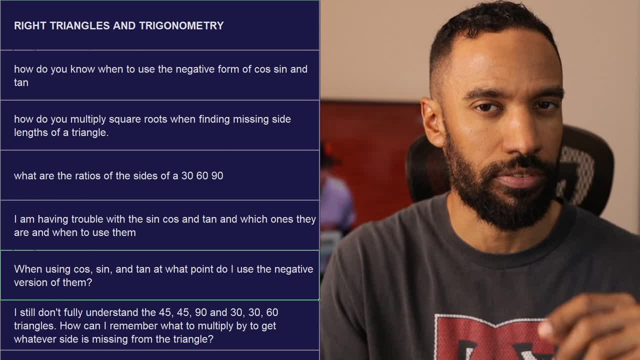 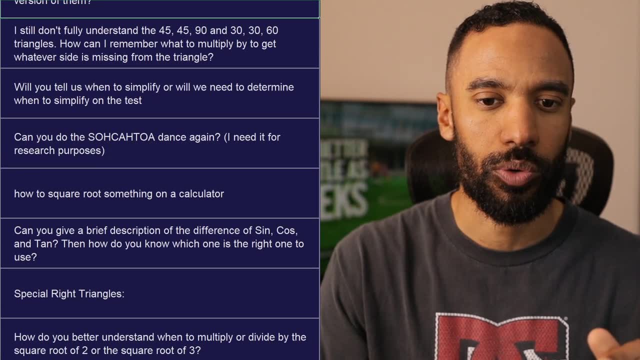 you mean inverse sine cosine tangent. Second thing is you use it to find angle measures. You use it on ratios to find angle measures. But I Answered it in detail up here. OK, all right. Next question asks: where am I? 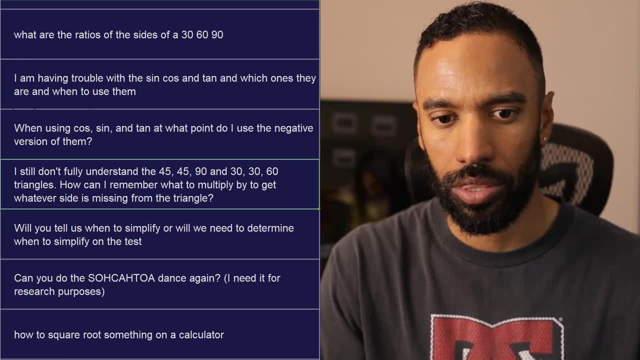 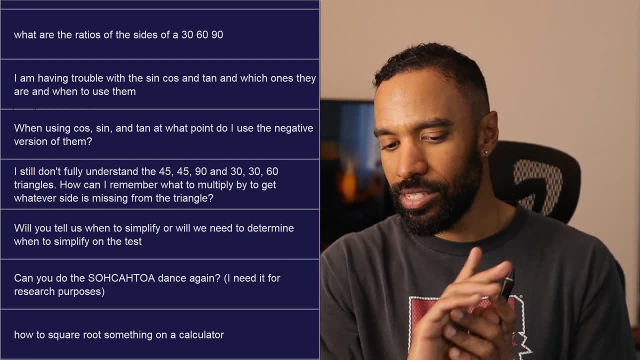 I still don't fully understand the 45,, 45,, 90 and 30.. Probably 30,, 60, 90 triangles. How can I remember what to multiply to get whatever side is missing from the triangle? Um, I'd say I'm I'm not big on memorization. 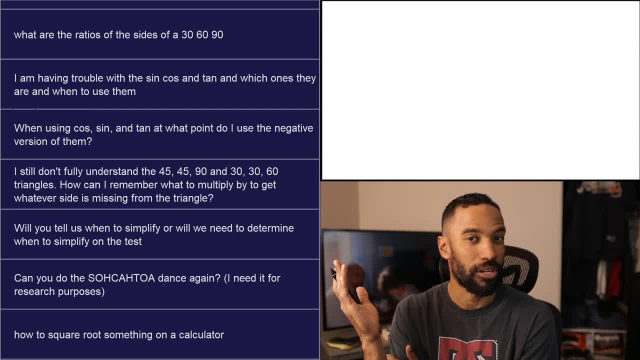 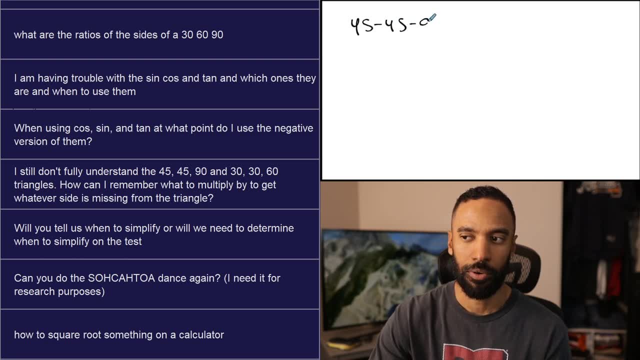 I'd say, at some point you kind of familiarize yourself with them, I'll say them again. I mean I'll, I'll say them over and over, right, That's a familiarity thing. The 45,, 45,, 90.. 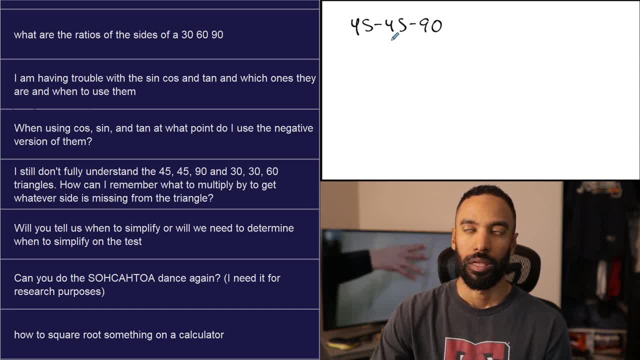 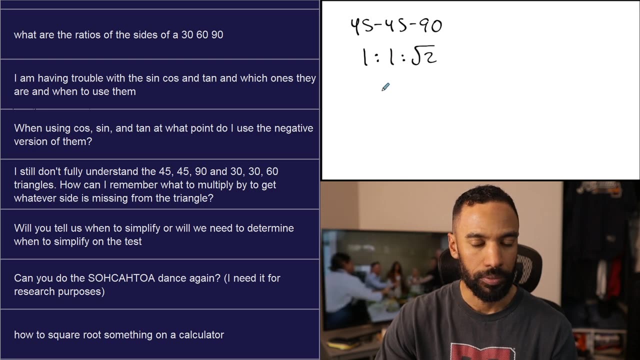 One's a lot easier to um come up with on your own, The the ratio is one to one to root two. We know that one is smaller than root two. Uh, the reason why this one's easier to kind of come up with on your own is a 45,- 45, 90 triangle is an isosceles triangle. 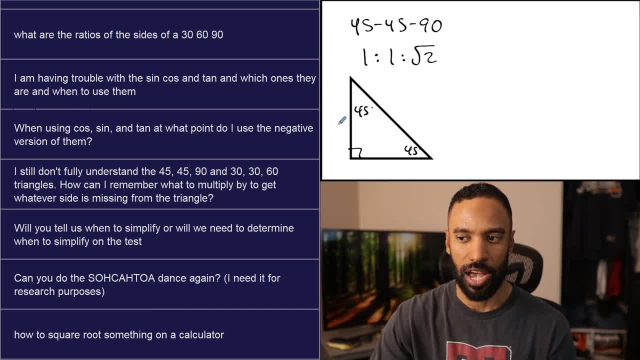 If these two angle measures are the same, then their sides opposite them are the same. They have a one to one ratio relationship. One to one isn't something that you first you heard for the first time in this chapter of this math class. hearing something as one to one means it is exactly pairing equal to it. 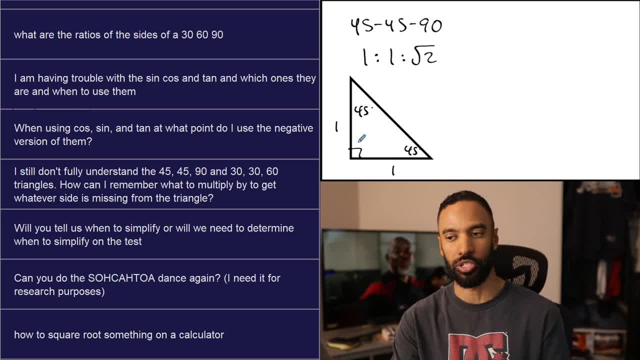 These are exactly the same length. I think we can all come up with that pretty straightforward. And when I did a proof in my own math class for this, in the lecture stuff which is also in that same lecture video I talked about, find my nine two- uh, the lecture video in my nine two. 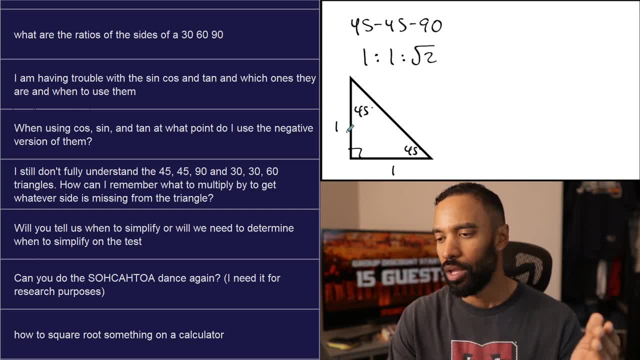 Uh, the lecture video in my nine two. Uh, the lecture video in my nine two. Thing, If you're in my Google classroom, um, or it's, it's titled there's, there's a YouTube video I have. 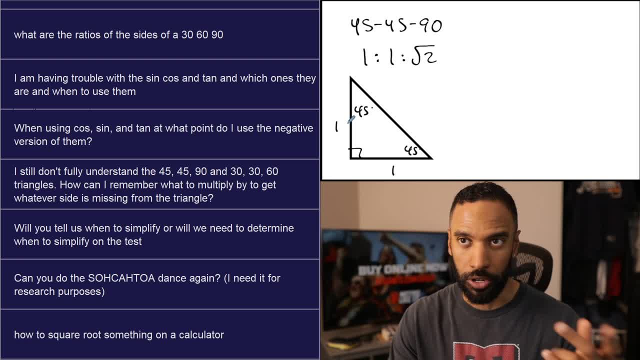 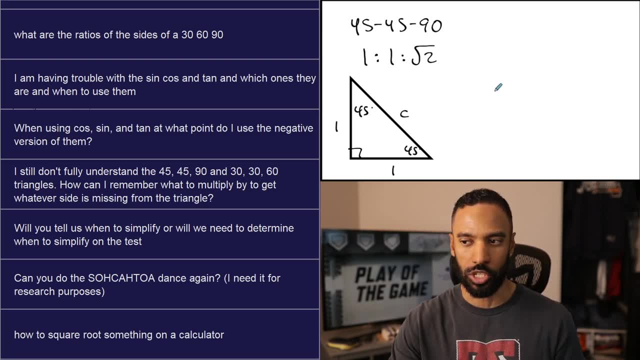 I should probably link it down below. She probably link my uh Pythagorean theorem stuff, right Triangle seven um special right triangles and trig stuff. Anyway, I can use Pythagorean theorem to find out what this length is, right here. 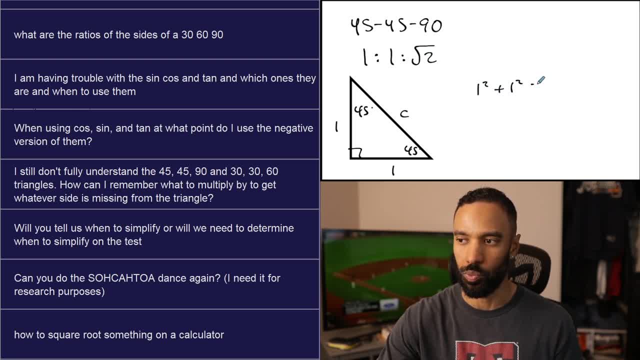 If I don't remember that, it's root two. let's just do one squared plus one squared and figure that out. One squared is one and take the square root of both sides, You get the square root of two. I mean, it's a very fast you know thing. 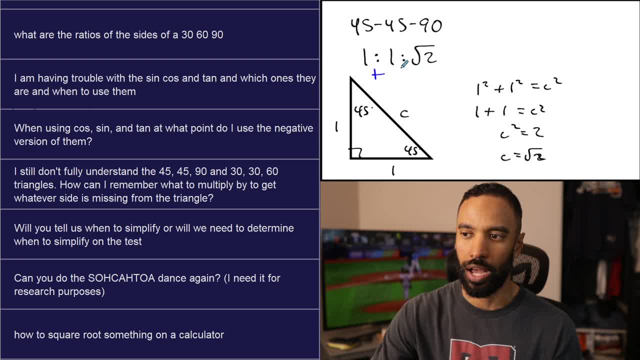 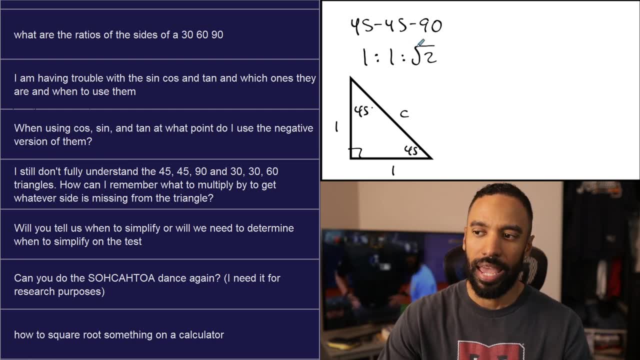 To get to. I mean, you know, one plus one is two. Obviously it's a root two. but one plus one is two is a nice way to remember that as well. Just saying it out loud it, it rolls off the tongue very well here. 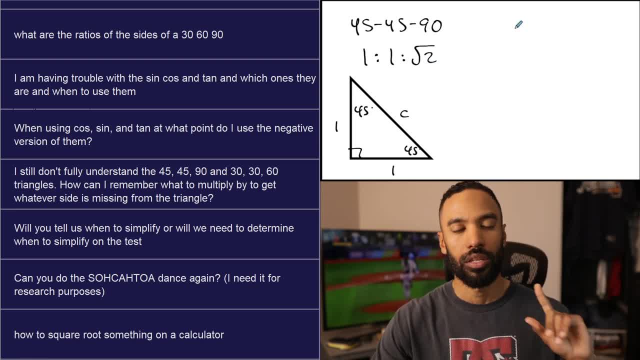 One to one to root two, one one and two there. Likewise, And I already talked about 36,, 90 triangle a little bit here, Someone asked about the ratios of the sides. Um, oh, let me uh before I talk about it. you said: 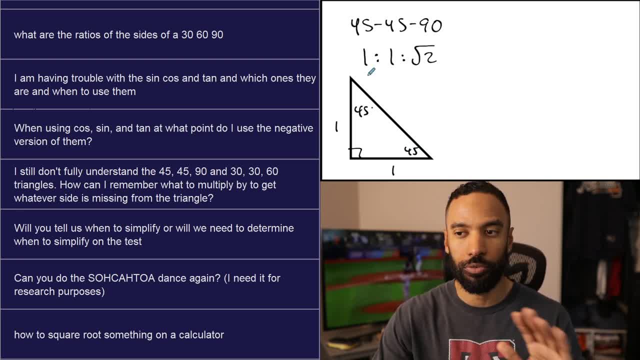 What to multiply to get whatever's missing. Hopefully you recognize this means that from a leg you find the hypotenuse by multiplying by root two and you go from the hypotenuse to a leg by dividing by the square root of two the whole one to root two ratio relationship means exactly that: that it's root two times larger than the leg. 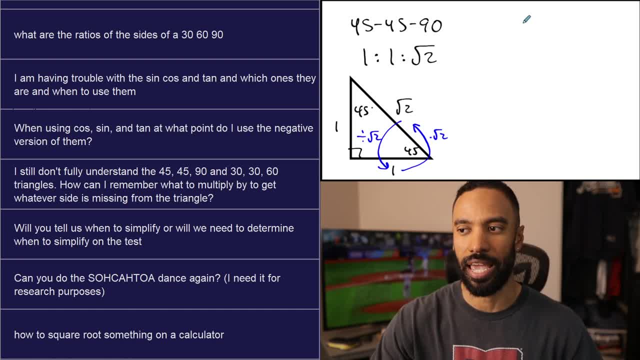 So you either multiply it by it or divide by it the 30,, 60,, 90.. And I again I've already brought it up, Uh and the other question, So maybe I'll go quicker here- but it's ratio relationship is one to two, to root three, being very careful of the fact that two is bigger than root three. 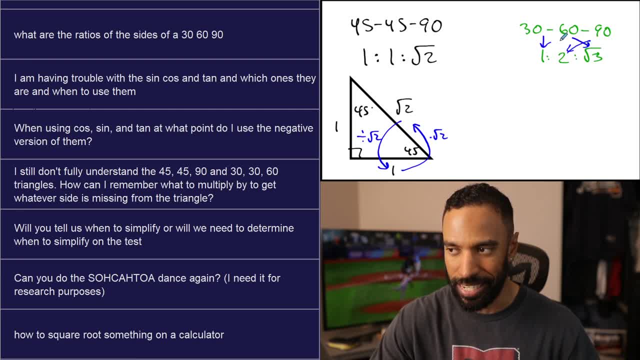 Therefore, two has to do with going opposite the 90 degree angle. but it's better to say one to two to root three than it is to say one to root three to two. You can tell it doesn't roll off the tongue as well, because we count one, two, three. we don't count one, three, two, and that root being the last number. kind of as nice as well. 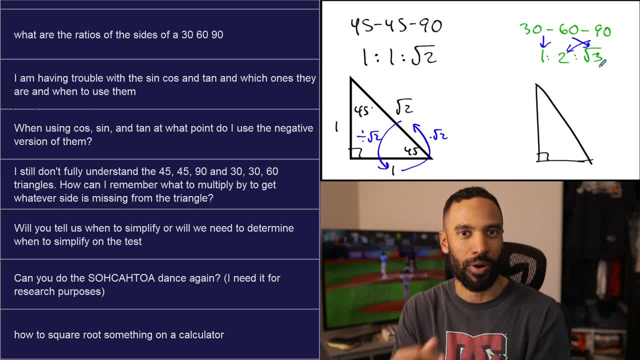 You know? yeah, I think those are things that we can just plant in, right, one plus one is two, and count one, two and three, and each of them have a little square root. at the end of it, There are little things to place and, honestly, there aren't too many things to like. memorize here, right? 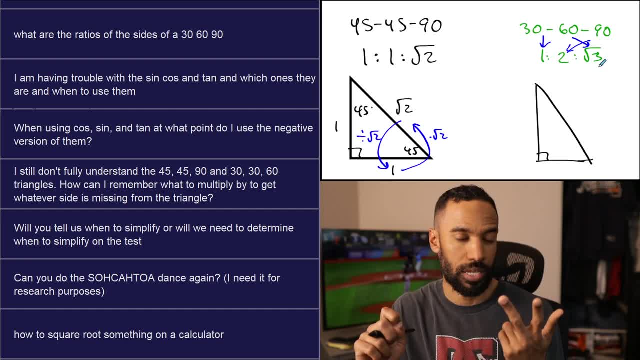 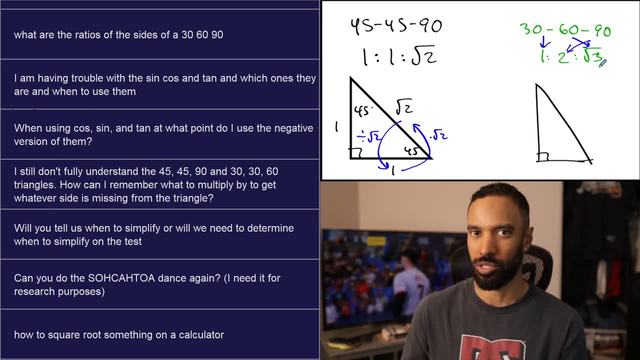 There's a squared plus B squared is C squared. There are these two sets of special right triangles and they're so Katoa and that's it. And I think we all know a squared plus B squared equals C squared. just from I am one, or from just alphabet based things. 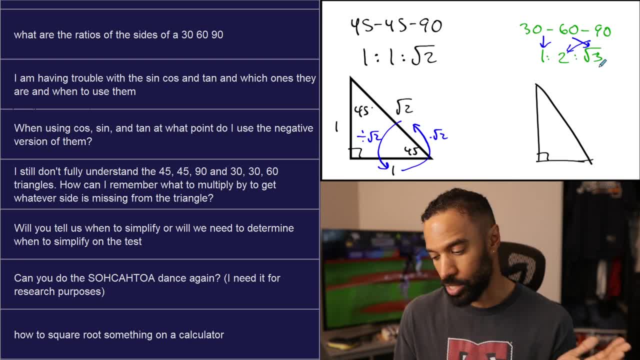 We've done them Before. so Katoa is a single spelling and from that everything will be generated. The other thing I'll mention: you know, when you get a quiz or a test, just draw these on immediately, Keep it in mind right before the test and do that. 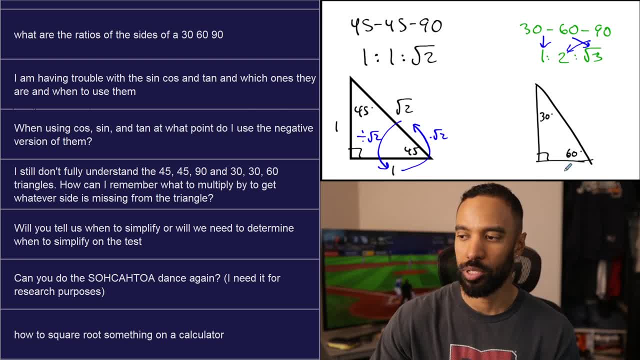 The question is: do you know how to compute with them afterward? Anyway, opposite the 30s one, opposite the 90 is two, and opposite the 60 is the root three. So from one to root three, you multiply by root three. 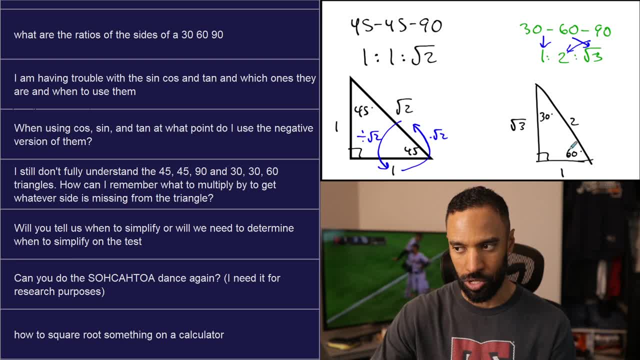 Here you divide by root three. Here you multiply by two, Here you divide by two, And I always go from either of those to the short leg, And I did talk Talk about those a little bit more up above. Maybe it'll be repetitive now if I 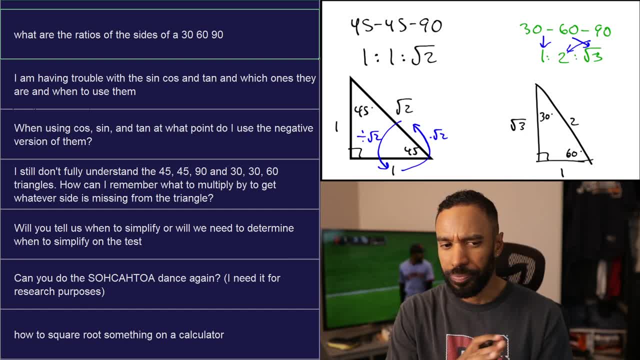 If you go back and listen to it, but hopefully I don't know if that answers your question, but that's, I hope I addressed it All right. The next question is: will you tell us when to simplify Or will we need to determine when to simplify in the test? 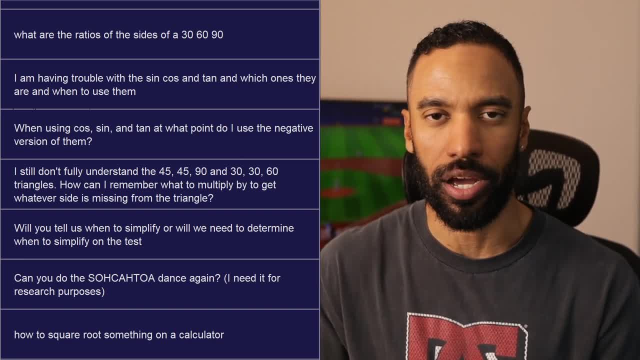 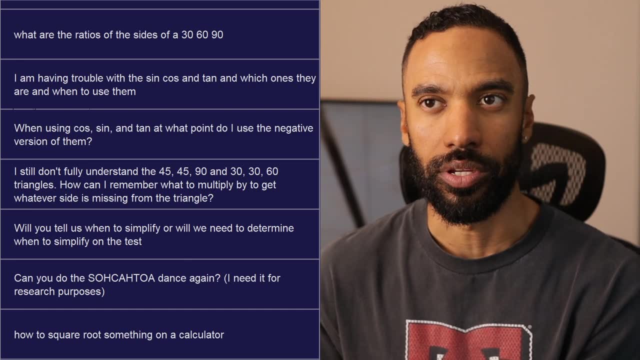 Oh, I mean, if I don't mention it, on a question you can ask me. The test is already written. I didn't write it, So I can either add Those instructions on or you can just ask me. for the most part, 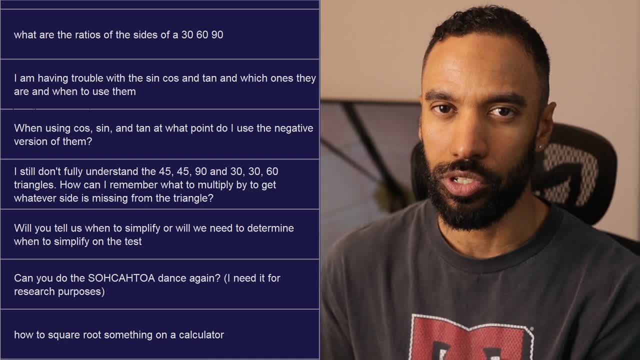 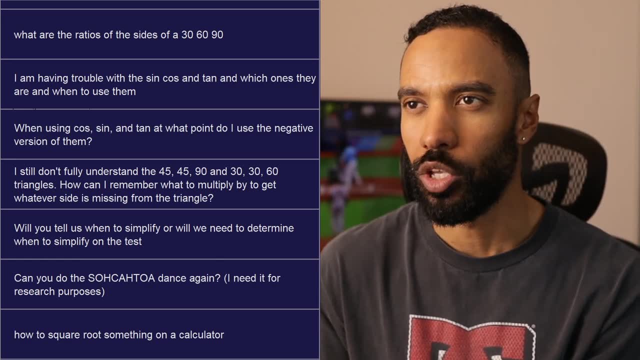 It's one of those things where if it's a special right triangle, you're simplified. If it's something from like 919293, you're simplifying. It's 949596 on trig, You're probably doing a rounding running to the nearest 10th or nearest whole number or whatever it is. 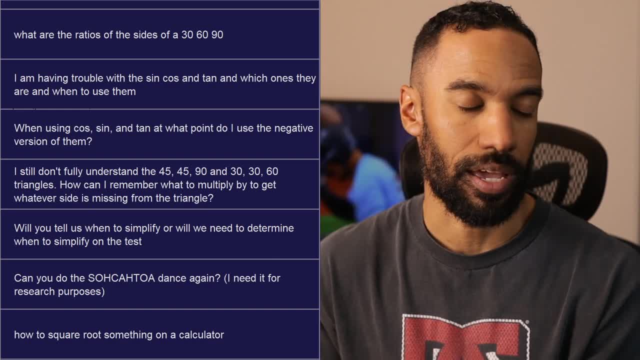 Because, yeah, I think it's pretty much it. You know, when we're taking the square root of something, it's like okay, if you're taking the square root of something and you can simplify it, you do that. The exception. 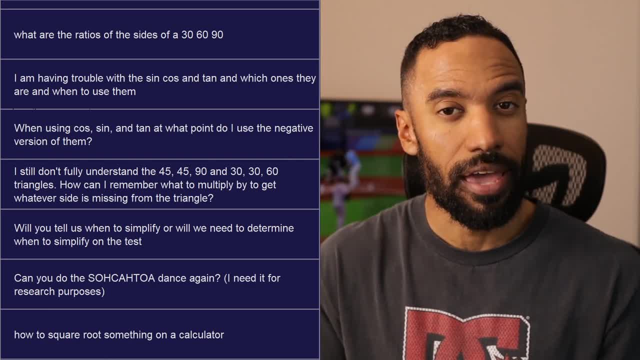 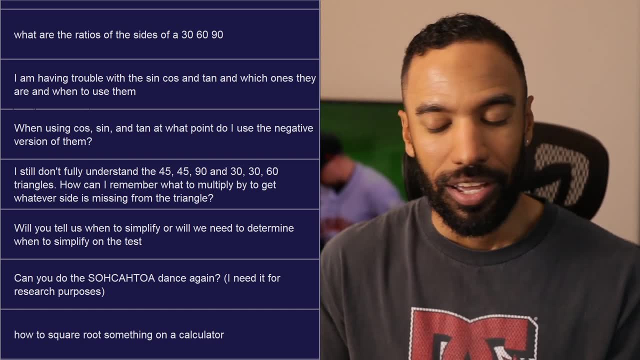 Is maybe a word problem. If you get the square root of 22, root 5 is an exact answer. But if we're talking about how many feet is the ladder, you know how long is the ladder? You'd probably say 4.5 feet. 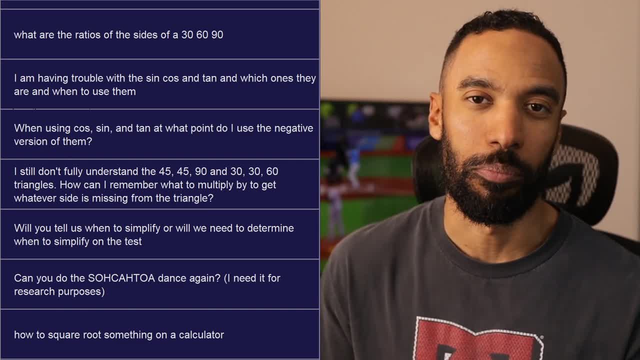 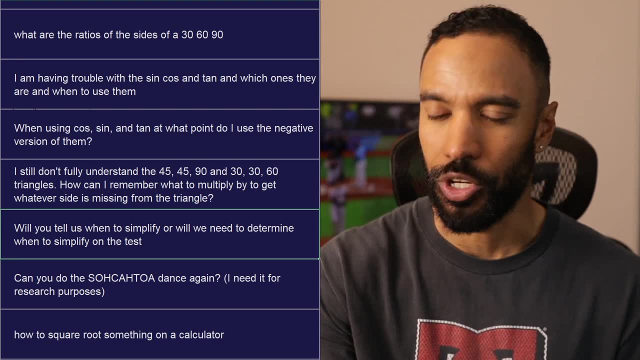 I guess that's a small ladder, but you'd say it was step ladder. We'd say 4.5 feet about, or something like that, instead of the square root of 20.. So yeah, I'll tell you. Sure, just ask. 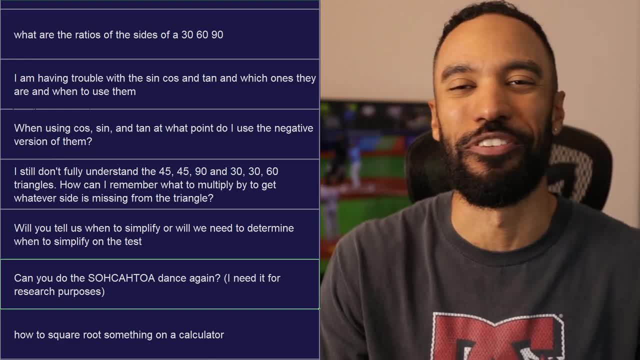 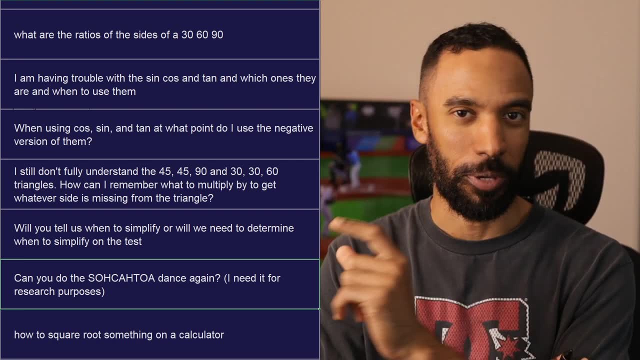 Otherwise I'll write it. All right, Can you do the Sokotoa dance again for research purposes? I'm not going to do it right now. There's no way I have to like film a thing, But, funny enough, I was thinking of actually filming it in my classes. 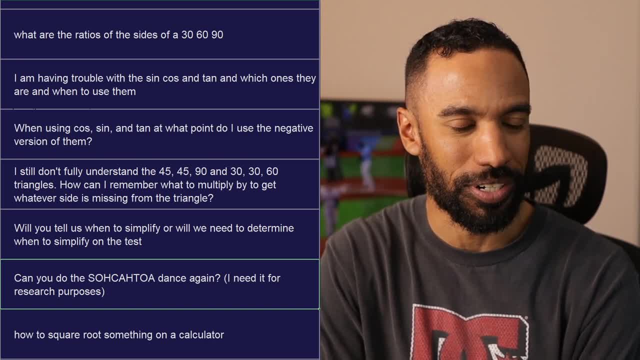 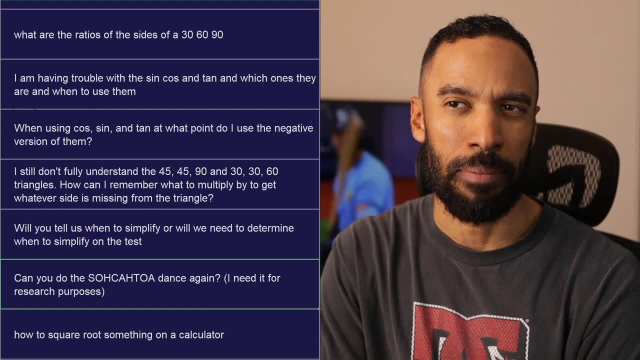 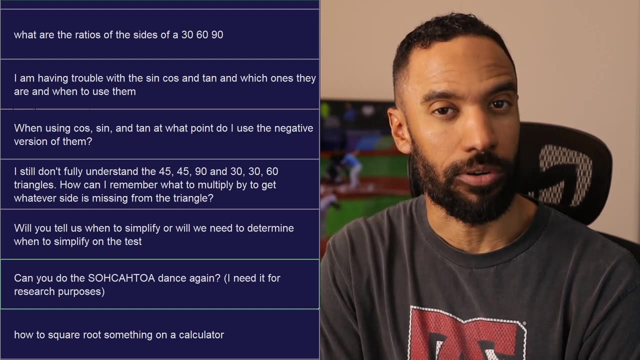 I just didn't have the camera prepped in a way to do it. Maybe next year I'll actually film it And all that stuff I made. I made up the dance portion of that story, By the way. it's a, it's a. it's a very popular folktale about King Fred and Queen Wilma. 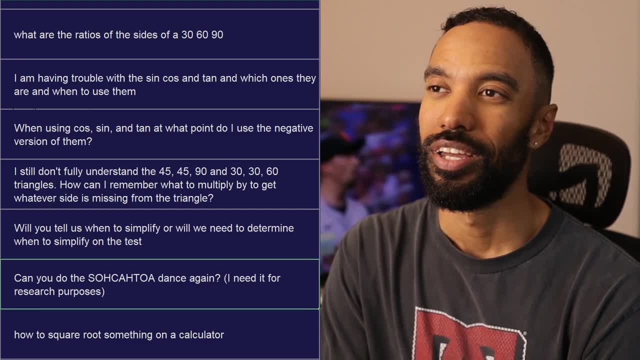 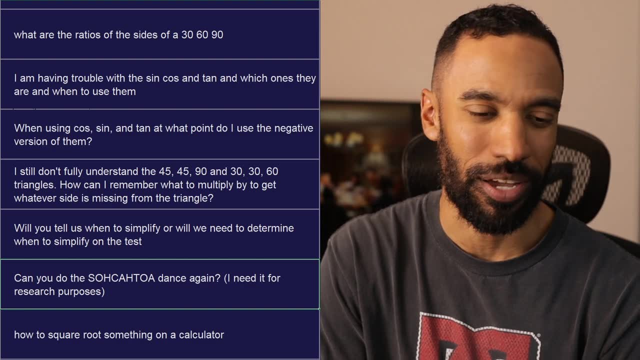 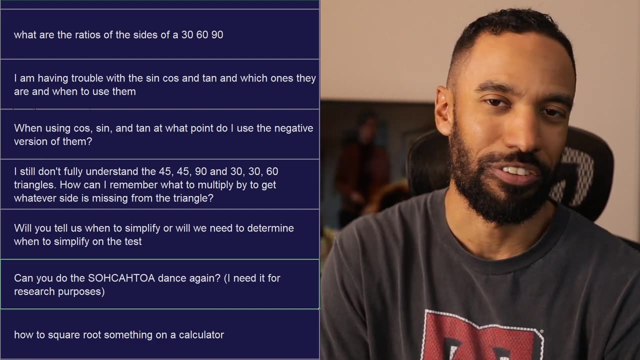 Of course King Klutz and Queen Sokotoa, But the the dance aspect of it is fully mine, Obviously using trig. but I own that portion proprietary until I film it myself And just look for it next year for research purposes. Absolutely. 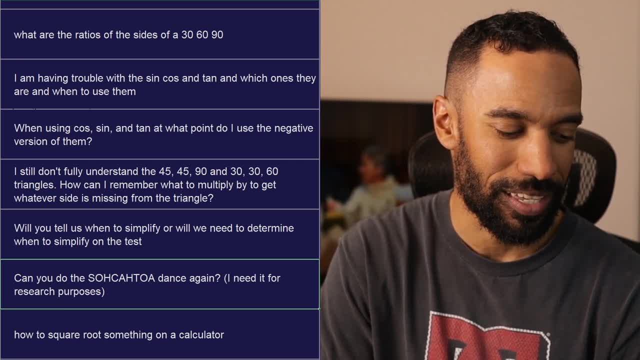 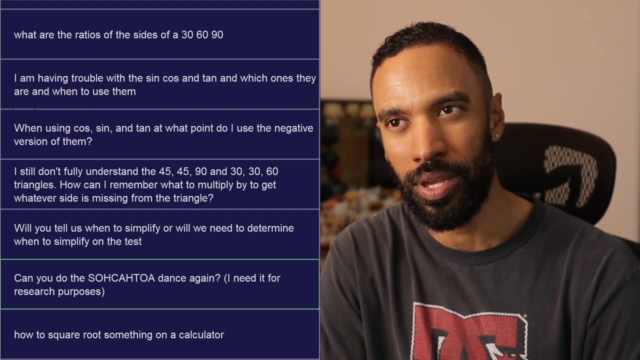 I yes, I did plan on recording it. The problem was there was brunch. Remember, we were on a block period and there was brunch time In between, So I had to step out and I had to go over a quiz and stuff first. 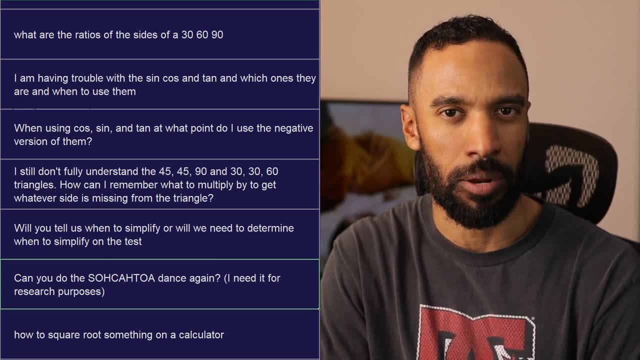 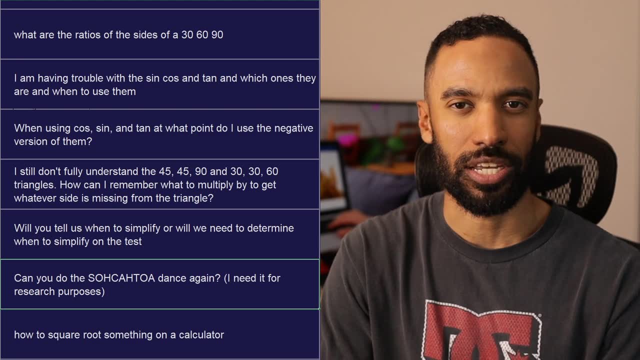 But basically I wanted the camera planted beforehand without you guys knowing about it, But I didn't want it to be recording for like 50 minutes. on overheating my camera And maybe I need to check the time or I need to check stuff for softball, or it starts overheating after a big recording or I run out of memory. 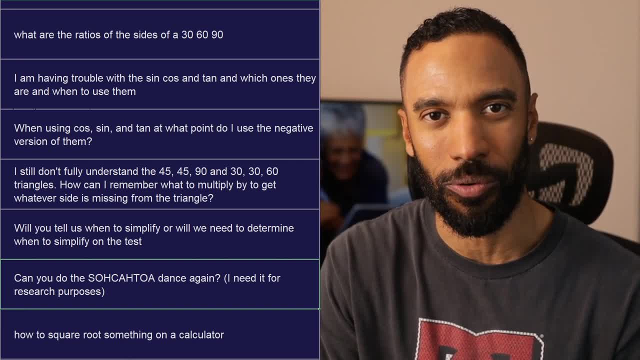 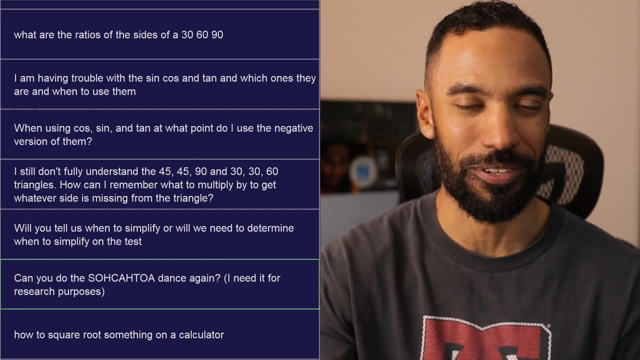 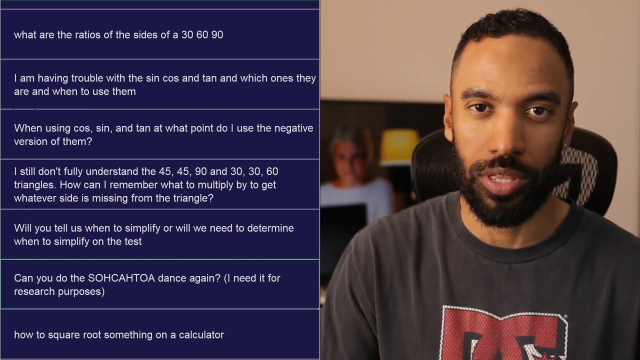 So there were logistical purposes for actually getting the recording in, But sorry, I don't know recording for you, Just the sine cosine tangent stuff. You're right, for research purposes. for research purposes, Honestly, try, try the dance. go up to the front of the room thing and make sure that you got your opposite hypotenuse. you know all that kind of stuff. 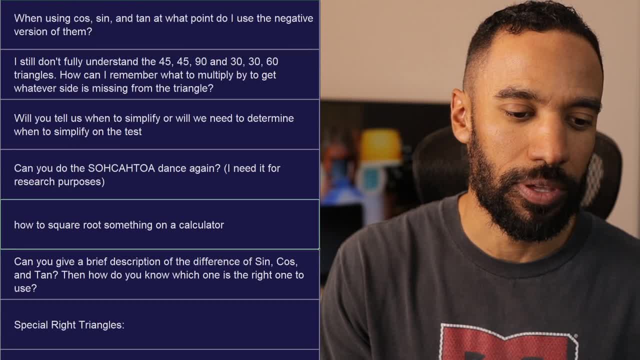 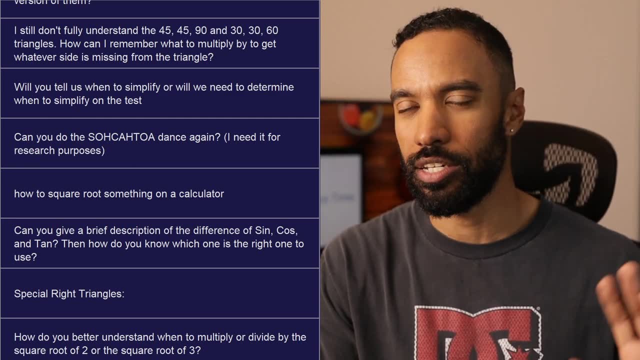 Make sure you know your Sokotoa for yourself. All right, how to square root something on a calculator. It depends on the calculator, Let me. let me pop up mine, The majority of them. if you're talking about just if you're talking about getting to simplify a radical, that's something you got to do on your own. 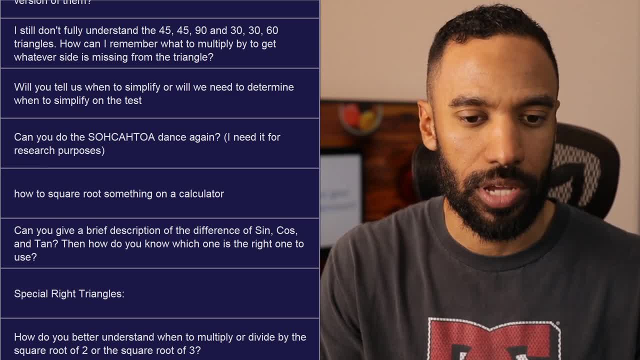 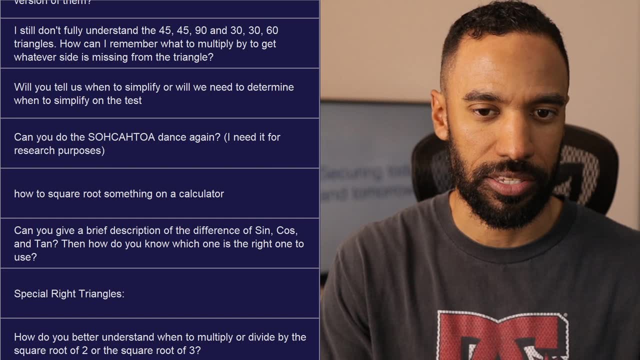 That's. that's something you're expected to be able to do on your own If you're talking. Talking about. I got to find out how to pop mine up most of them, and this calculator will be different than the ones we use in classes. 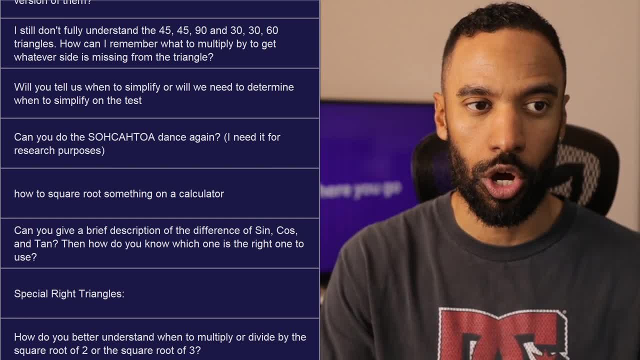 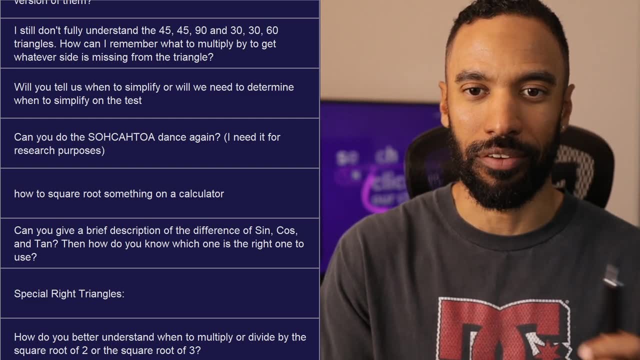 And if you have to ask, I guess in class you can. but my hope is you've been practicing long enough. We've been using calculators long enough, at least in my class, or I've been asking you to not use your phone as a calculator or whatever, that you should be expected to know how to use it kind of on your own by the time of a test. 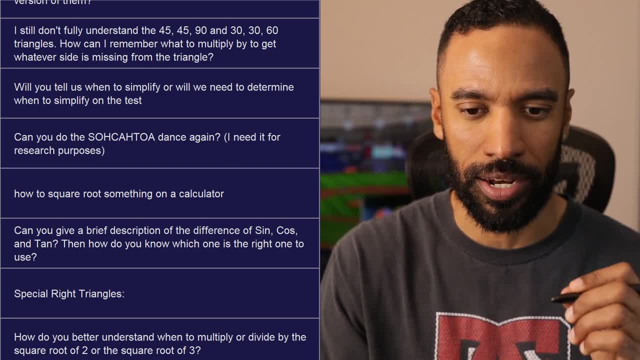 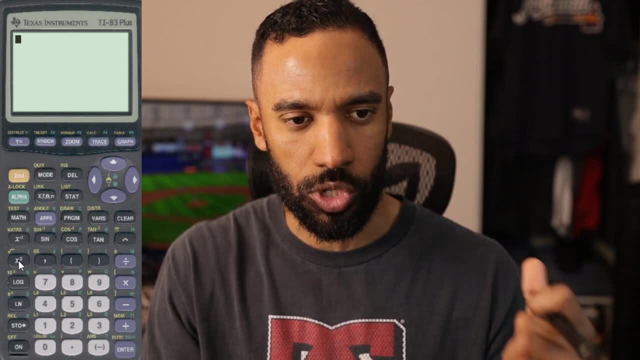 But if push comes to shove and you absolutely have to know to get something right, I guess I'll help you out. the graphing or my graphing calculator that I have here We kind of similar to what you do here. Normally there's a button where you square something. 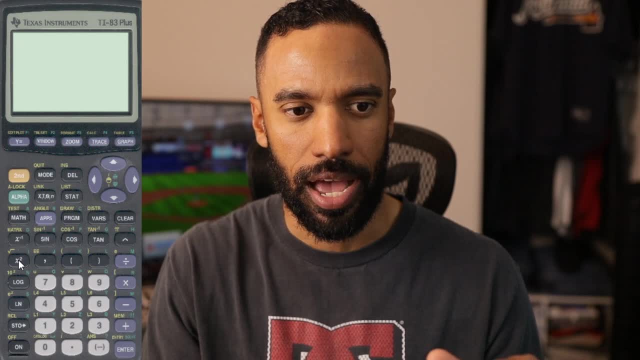 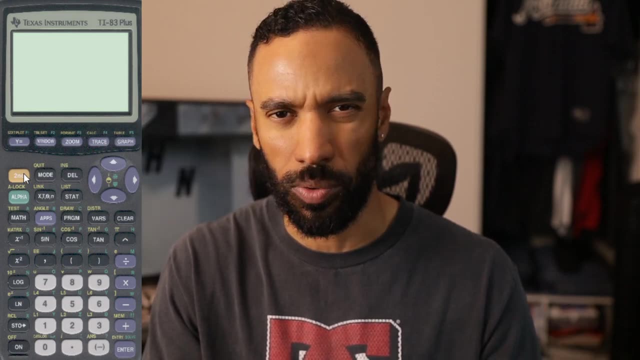 Like that, and then the functions right above it. I don't mean the next button, I mean the icon is above it right there, which means you have to access the second button. So on my calculators in my classroom I think it's a green button. 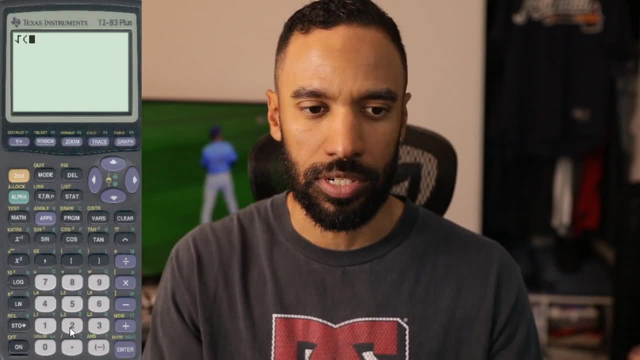 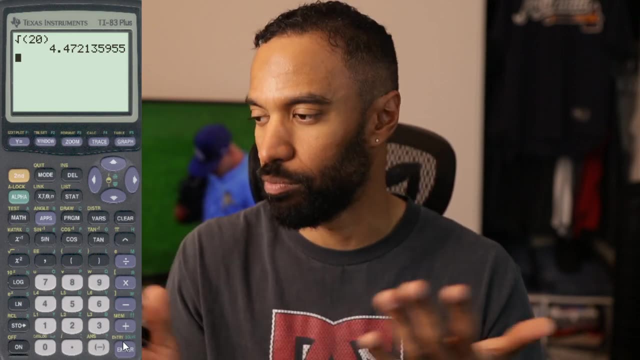 That's second, This one's yellow. you hit second and then you hit that thing and then you can take the square root. I talked about the square root of 20 before. I think it's around four and a half. Yeah, so if it runs to the nearest tenths- around 4.5, and there's a button, 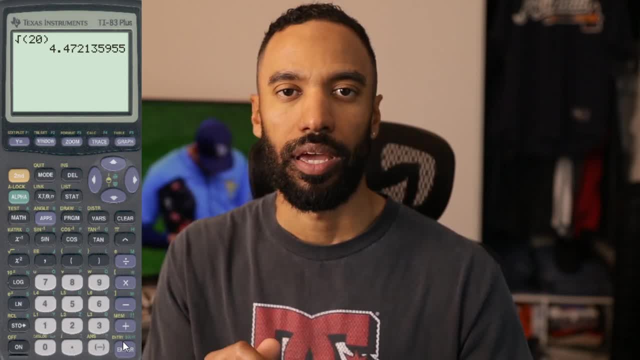 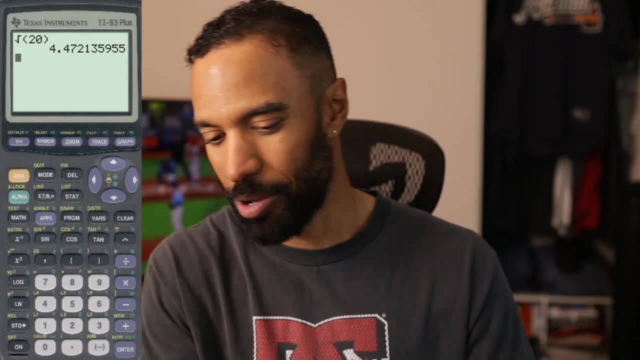 I want to make sure my calculators Are all in that mode. that gives you decimals and yeah, that's that's how you do it. Hope that addresses it. Good question Either way, Hope that was helpful. Okay, let's go to the next one. 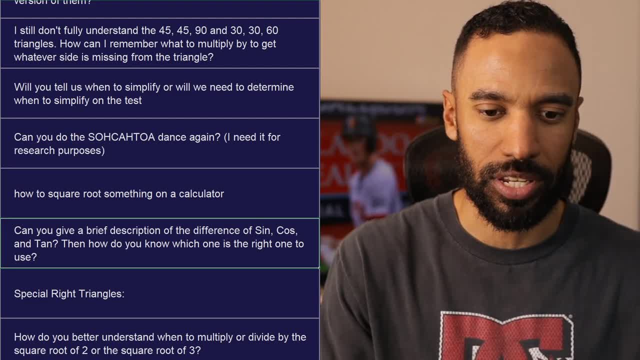 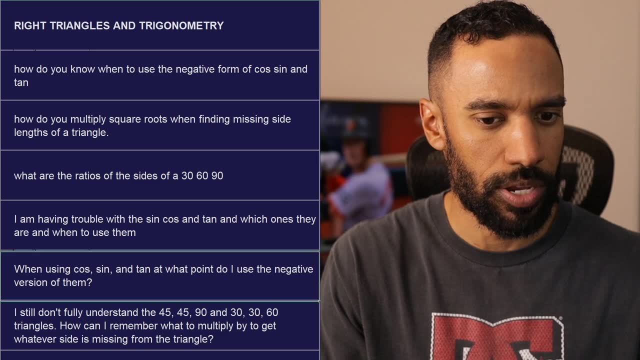 Can you give a brief description of the difference of sine, cosine and tangent than how you know which one's the right one to use? So I did answers before a little bit. If you go and check this question right here having trouble with sine. 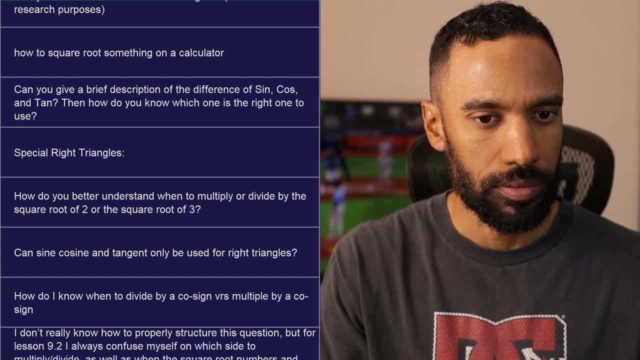 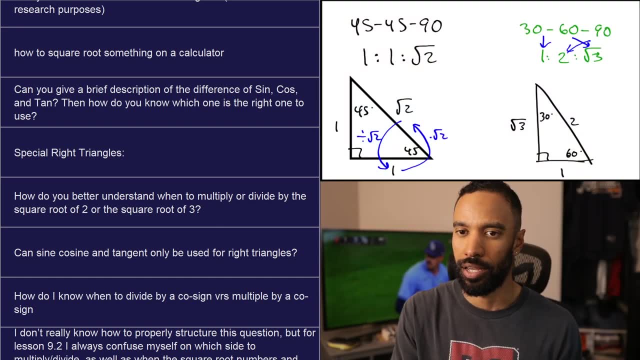 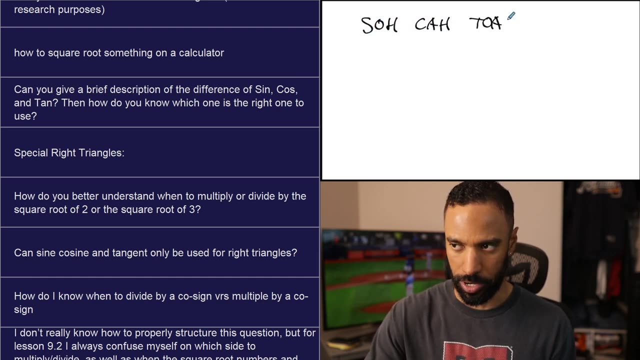 cosine tangent one. what I will Revisit, though, is first of all the way to spell Sokotoa. Let's go to that Sokotoa, because this answers that question Relative to the angle that you have one of the acute angles in your right triangle. 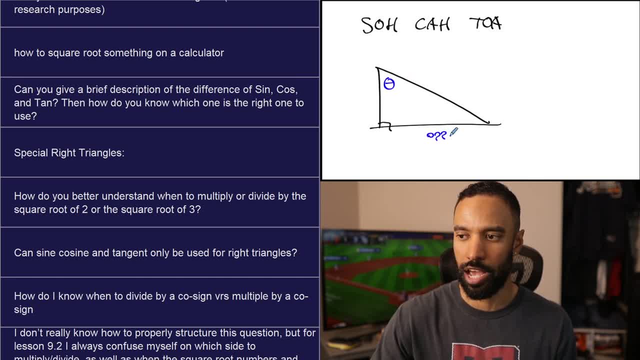 If it's this one right here, relative to this angle. here's the side opposite, Here's the leg adjacent to it And here's the hypotenuse of the right triangle sine uses opposite divided by hypotenuse. So and one thing I answered in that other question. 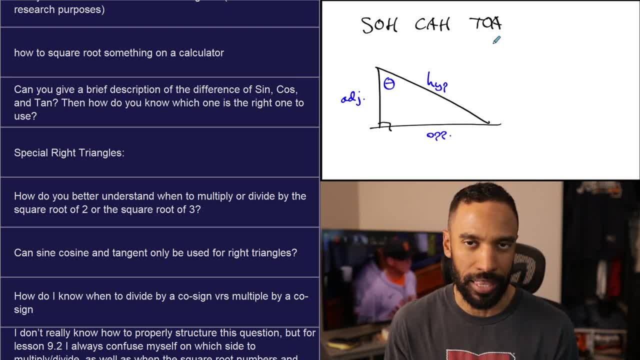 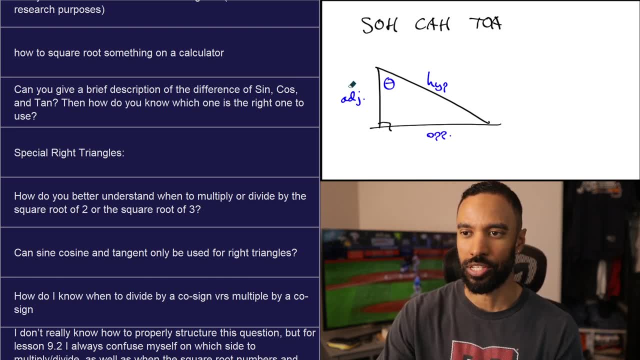 I think is the first thing that I said is there's no one trig function That's better than the other ones. It's not signs better than cosine and tangent. Nothing like that depends on the information that you have. If I don't have the adjacent leg, 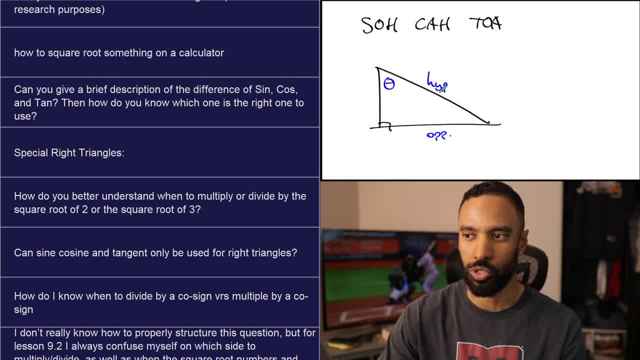 I'm going to use sine because I have the opposite and hypotenuse, or you know, when I say I have, I mean if one of them is X, you're trying to find it Okay. if it's labeled right, I'm going to use sine in this case. 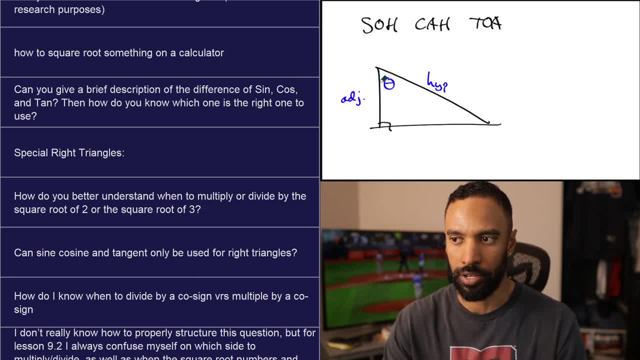 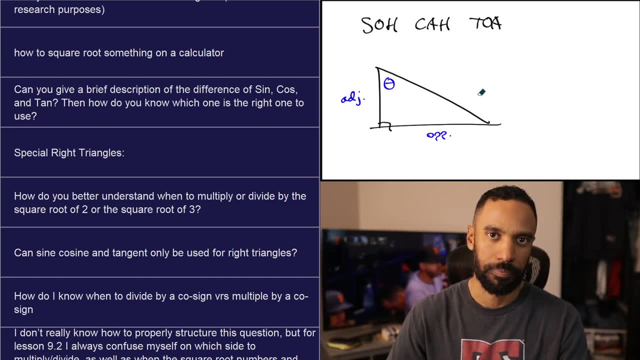 but in this case I'm going to use cosine that uses adjacent or hypotenuse, And in this case I'm going to use whoopsie. this case I'm going to use tangent, because I have opposite over adjacent. It's fine. 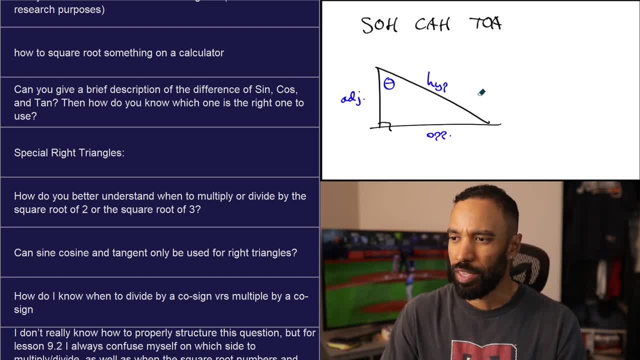 If you have all three, it's your choice. Use the one that would you think you'd most benefit from. maybe one of them has a radical and you want to avoid it. Maybe these lengths are and I need to do something that actually works. 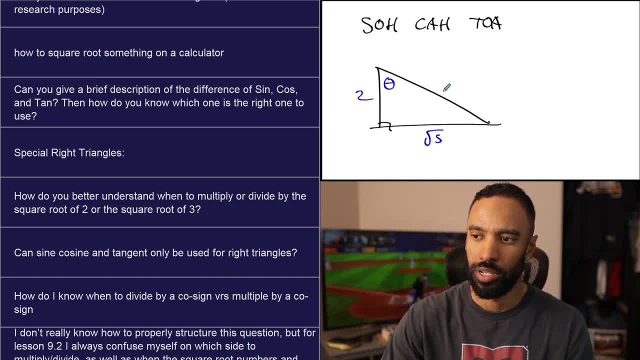 What was the one from our quiz? We had a root, five and two, two and you had to find out that this was three, whatever, but let's say it was these ones. Maybe I don't want to use Siner tangent because I don't want to use a square root. 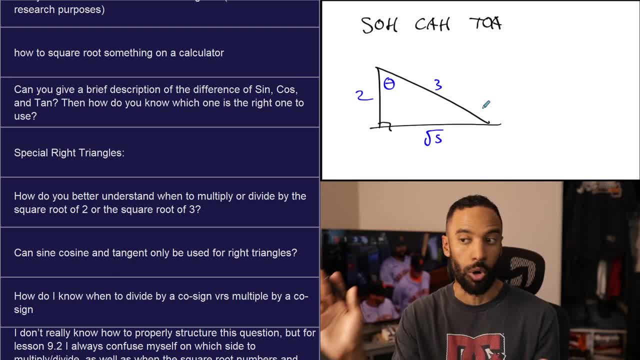 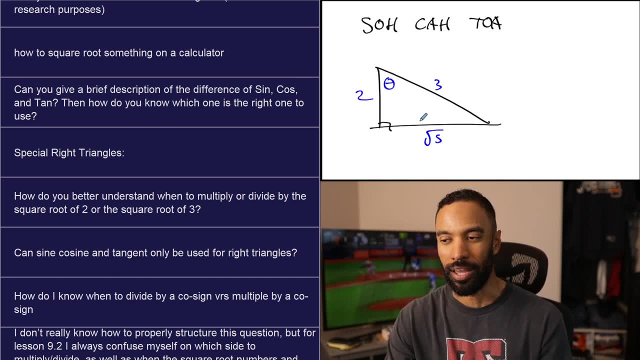 I listen to. square root doesn't make the problem harder. Oh, this is to find an angle measure Now. by the way, this is now to find an angle measure, not to find one of the sides. but yeah, it's like okay. 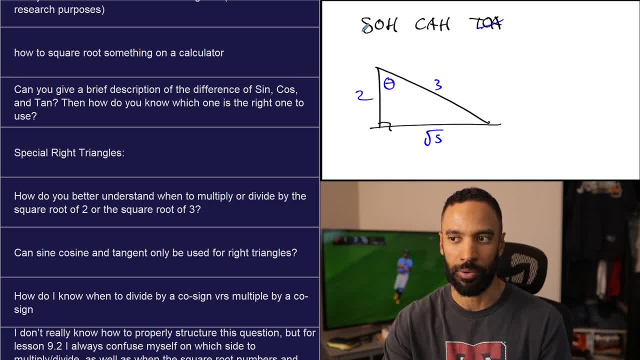 I don't want to use the square root, So I don't want to use anything with opposite. So tangents out and signs out. I'll use cosine. I'll say the cosine of my angle is two-thirds and then I'll take the inverse cosine of both sides. 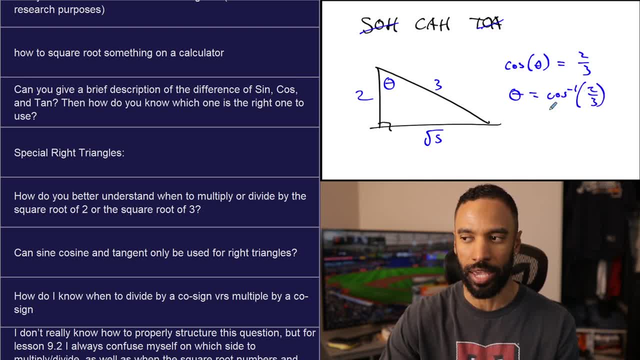 and I get inverse cosine of two-thirds. That's no different. Whatever I answer you get here is the same Same thing as the inverse sine of root 5 over 3 because and the inverse tangent, the inverse tangent of root 5 over 2.. 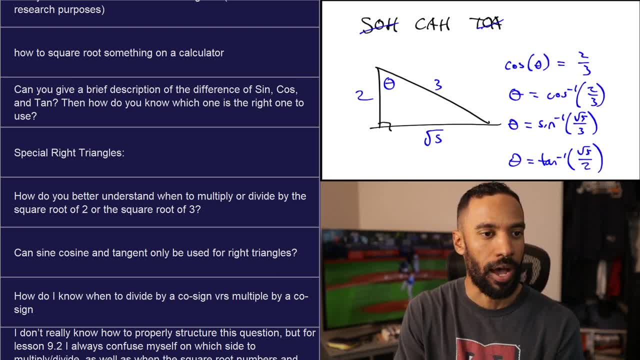 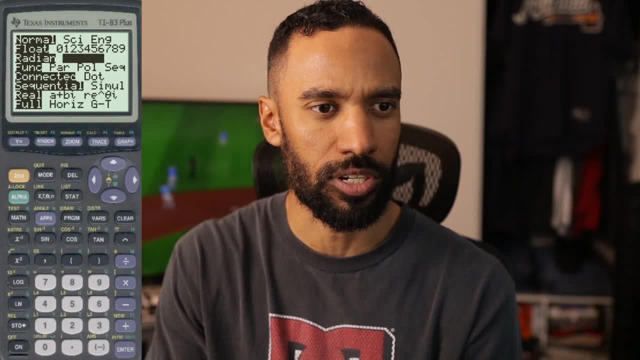 All of these are the exact same answer. Try them in your calculator. I'll go do it right now. I need to make sure my calculators in degrees when I do so, because it's probably not some radians right now. So I got to be in degrees. 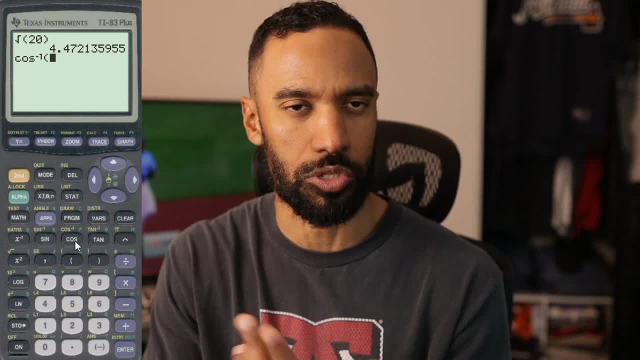 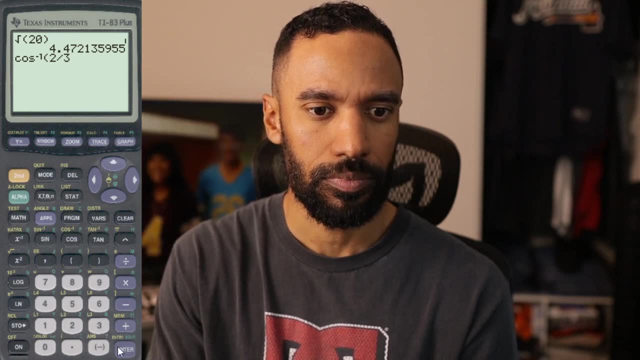 But yeah, if I take the inverse cosine- I don't know what the angle is, but I would take the- it's probably close to 45, little more than 45.. Inverse cosine of two-thirds: Yeah, 48, whatever. inverse sine of root: 5 over 2 over 3.. 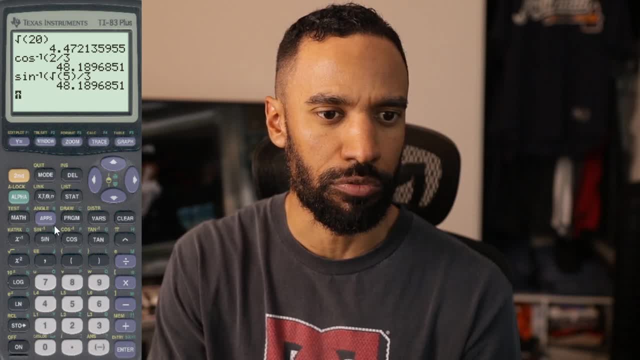 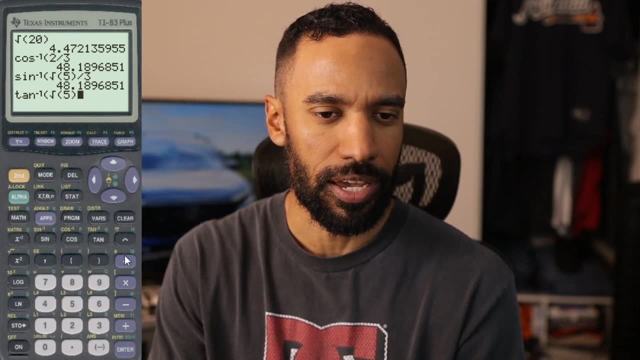 Excuse me, Is that number and inverse tangent of root 5 over 2 is the same number. So you know they're all the same, whoops, They're all the same value, And the reason is because they're all referencing the same angle in the same triangle. 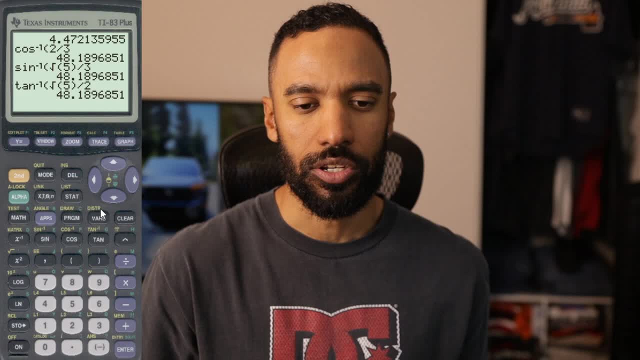 It's. it's a triangle with those ratio relationships and that's the angle measure. So there's no one versus the other. that's kind of preferred or anything like that. It's just a matter of what it is. You have what it is. 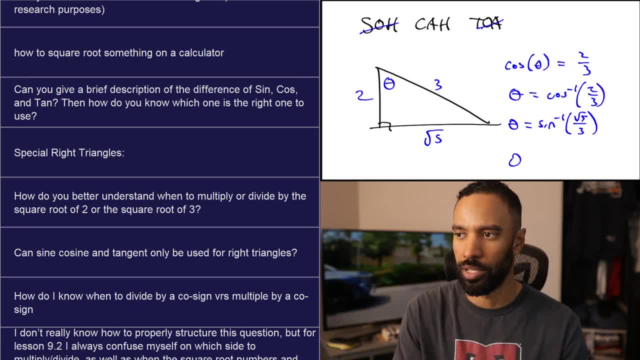 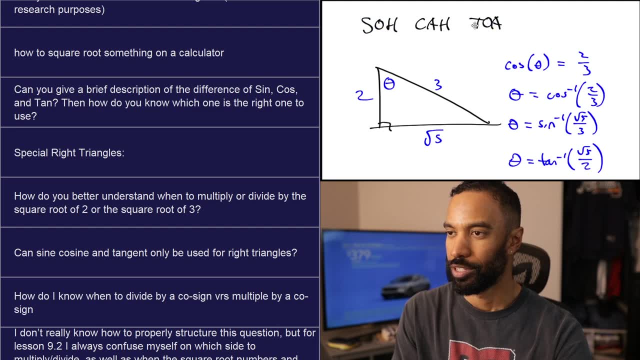 You're dealing with all based on SOH CAH TOA. It's all based on SOH CAH TOA. Keep those up there in case I need to use them again. Let me just get rid of this crossed out part. So CAH TOA. 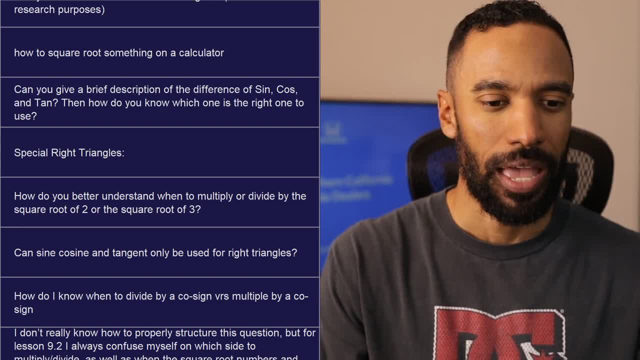 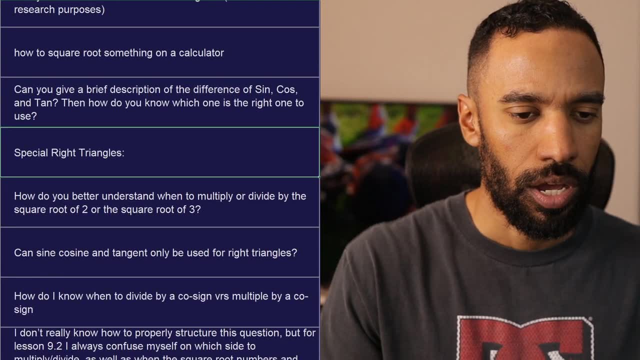 So I hope that helps answer your question. How many questions do I have left? I don't know Where am I right now. I'm here, So I have those. I don't know if this was a question, I just copied and pasted. 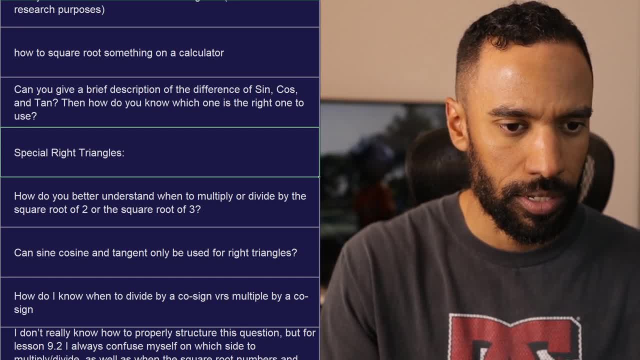 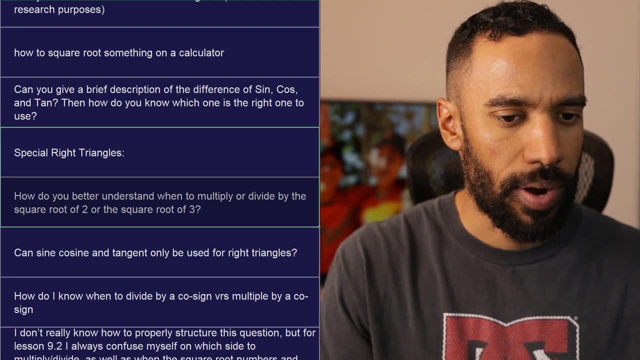 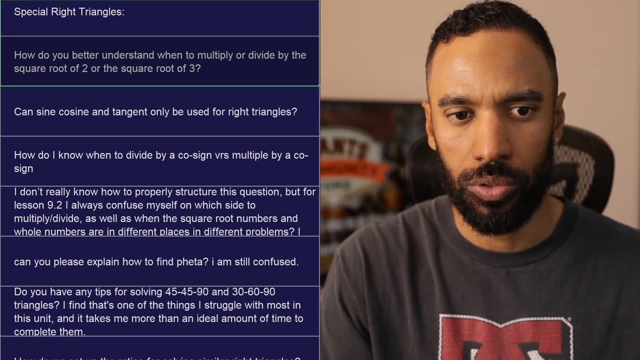 Was this the question? special right triangles? Let me find my maybe. maybe. maybe these are one question. Okay, here we go. Special right triangles: How do you better understand when to multiply or divide by the square root of 2 or the square root of 3?? 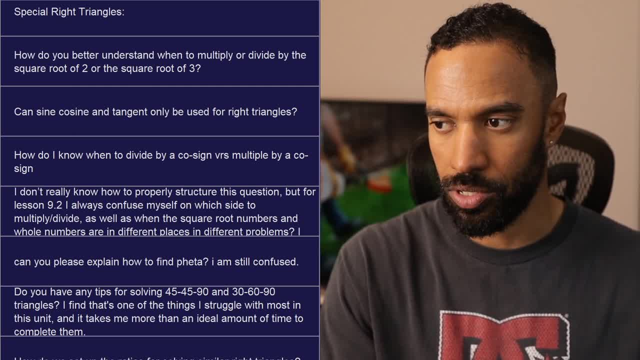 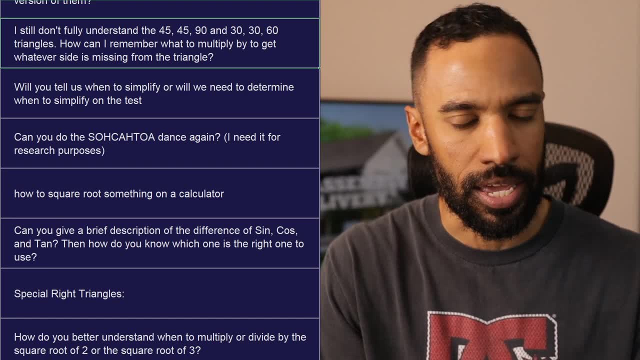 This is based off your special right triangle ratio relationships. So I have I did fill out, if you go to this question here, which this should say 30, 60, 90. I just pasted whatever was copied. You go to this question here. 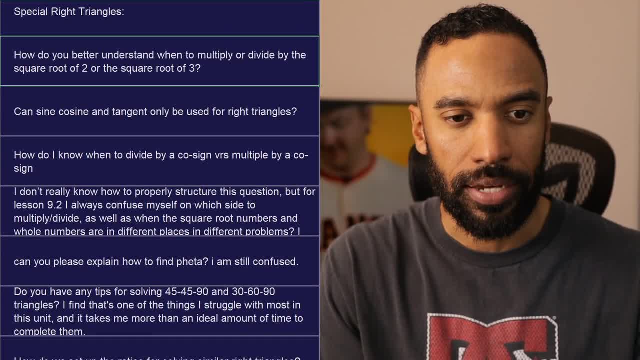 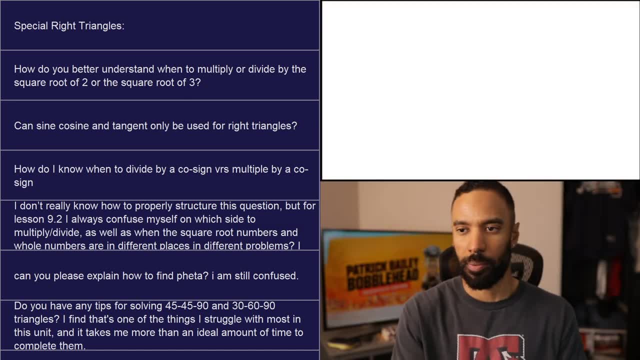 I do display them a little more, But how do you know when to use one versus the other? It's based on which right triangle you're talking about, So depends on if you're talking about the 45, 45, 90 or the 30, 60, 90.. 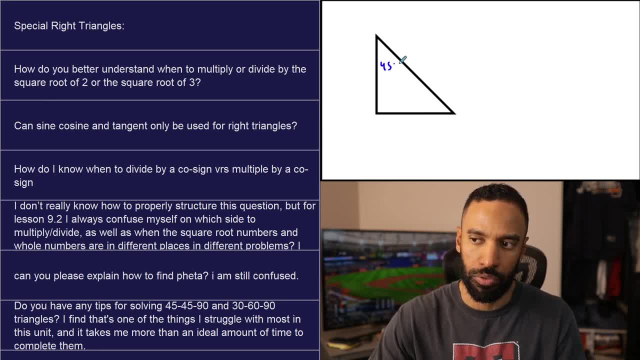 The 45, 45- 90 has a root 2 in it and the 30- 60- 90 has a root 3 in it. So this one has the root 2. I multiply by root 2 when I know the leg of my 45,. 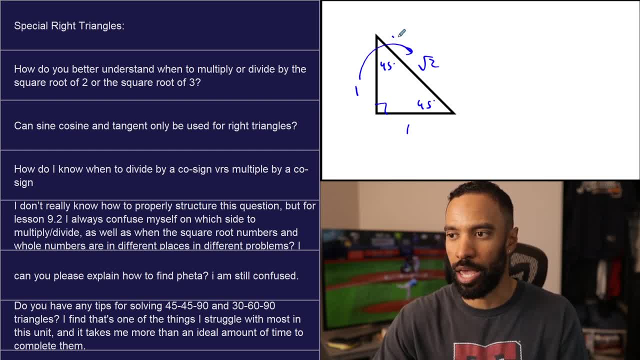 90 triangle and I'm trying to find its hypotenuse. This is a multiply by root 2 scenario. I want to multiply by root 3 when I wow. I want to multiply by root 3 when I know the short leg of my 30, 60, 90 triangle here. 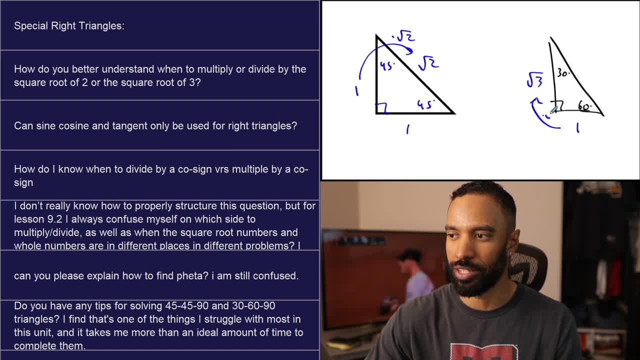 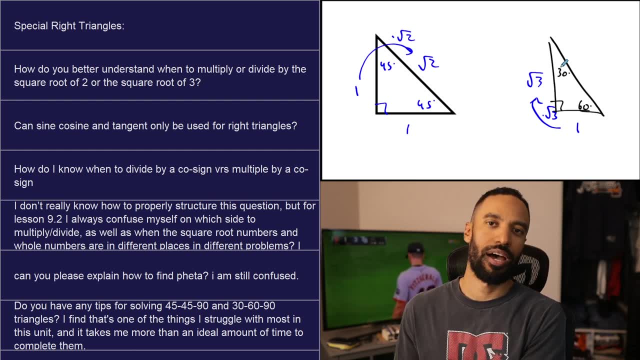 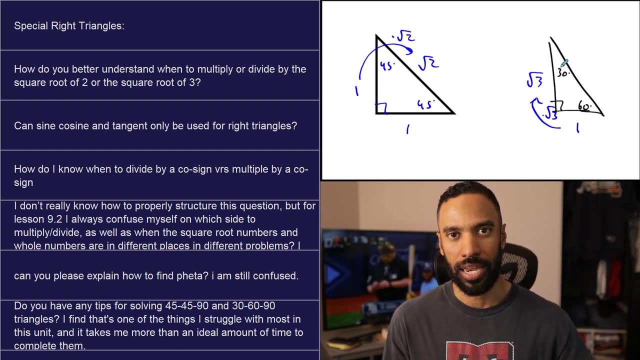 and I need to find the long leg of it because it's root 3 times larger than it. That's, that's when I do which one. I do What you want to understand, not not just you who asked the question. What students want to understand here is these right triangles are special. 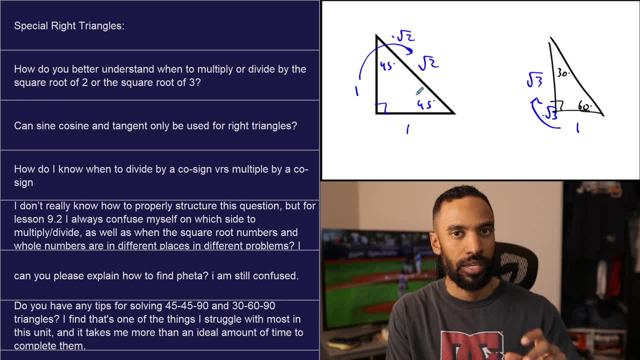 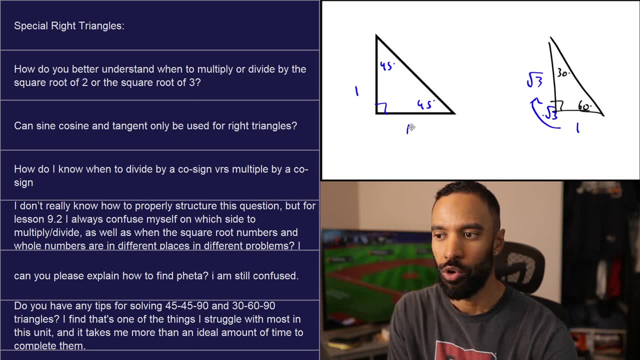 because these ratio relationships are so clean together. but any 45- 45- 90 triangle has this ratio relationship. It doesn't matter how big or small it is. Remember a 45, 45- 90, no matter how much I grow or shrink, it maintains that ratio relationship. 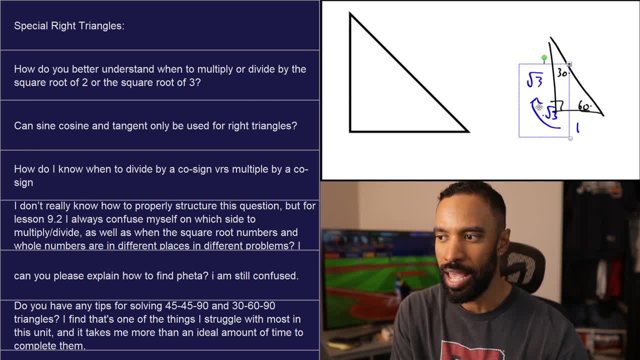 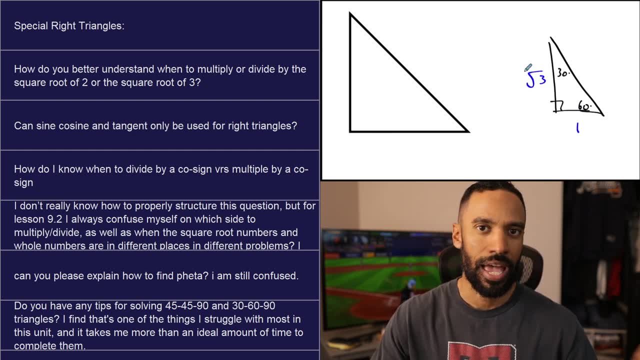 This one to one to root 2 and same with the 30- 60- 90. in any 30- 60- 90 triangle The long leg is always root 3 times larger than the short leg and I know hearing root 3 sounds weird. 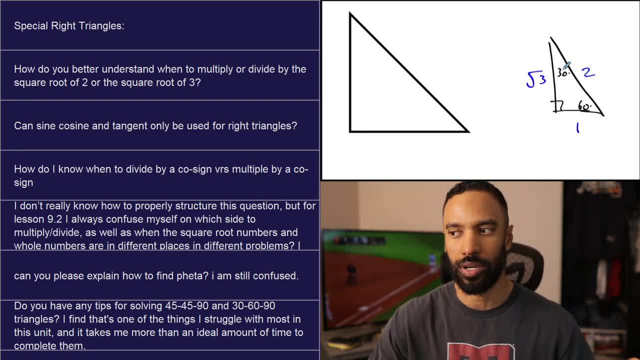 So let's go with the hypotenuse. Hypotenuse is always twice as long as the shortest leg in the 36 90 triangle. It doesn't matter how big or small that triangle is, because of similarity. Similar triangles have proportional side lengths. 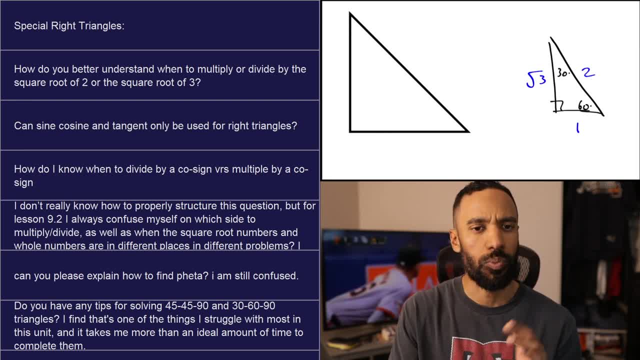 and this is the proportionality of a 30, 60, 90 triangle. Anyway, that's when we multiply by the root 2 versus the root 3. depends on which triangle you're talking about. 45, 45, 90 triangle is a root 2 in it. 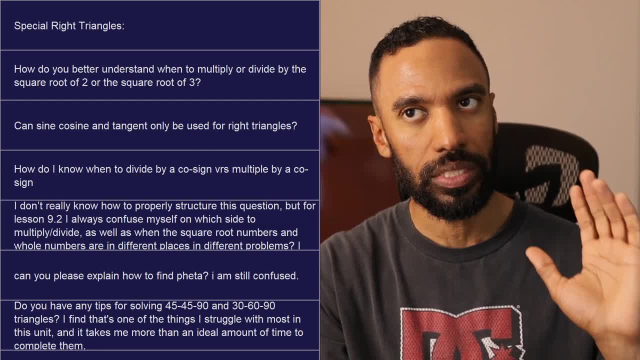 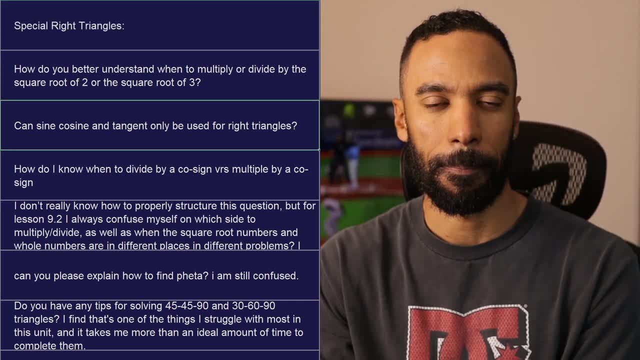 For the hypotenuse compared to the leg length, either leg length and the 30- 60, 90 triangle is a root 3 in it which represents the long leg. in comparison to the short leg, It's root 3 times larger. 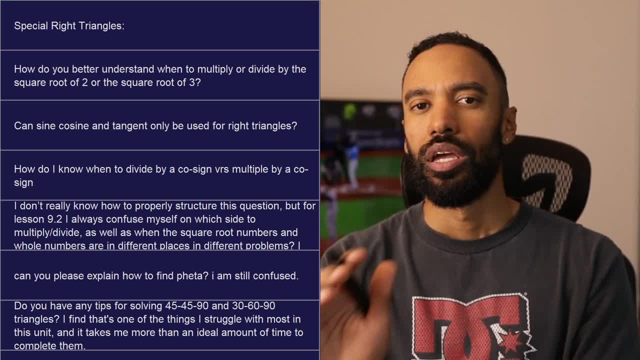 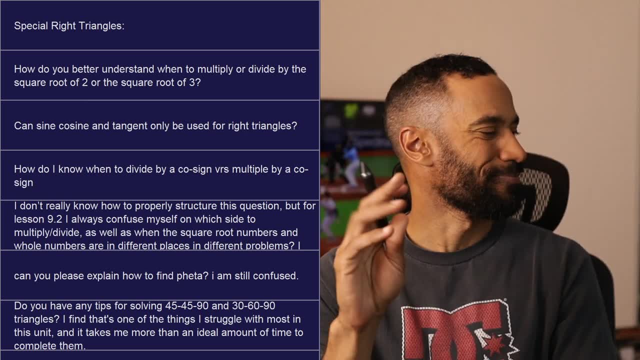 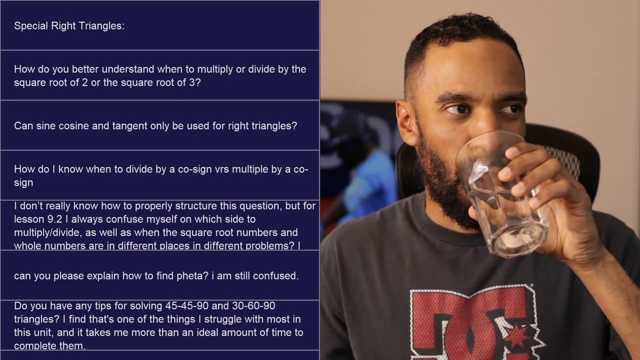 All right. The next question is: can sine cosine and tangent only be used for right triangles? No, But the ratio relationship? Well, I don't know how to answer that for you, and I am too. You can use it in other triangles. 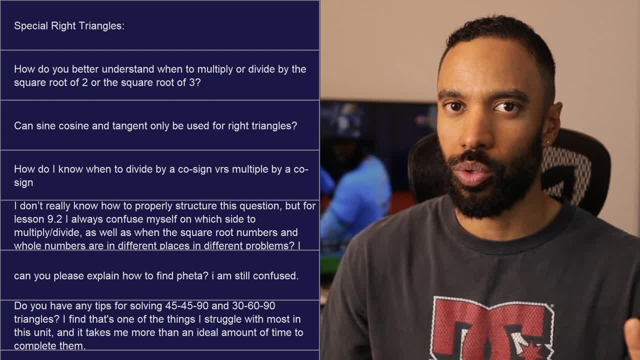 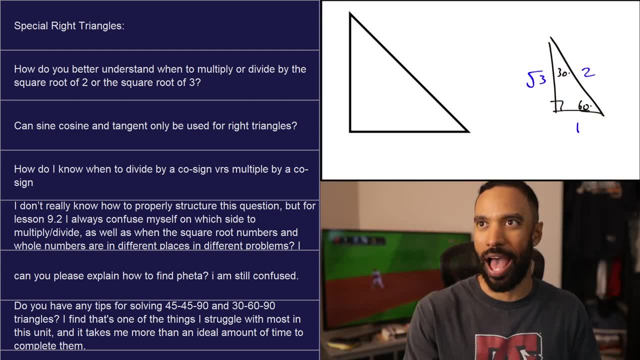 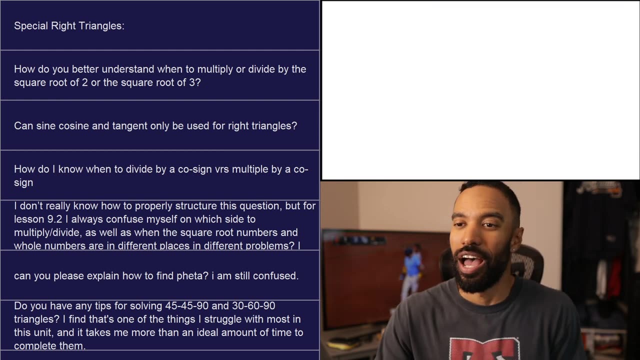 but its function served is based on a right triangle premise, Best I can say. I feel like I know who asked this question, Because just based on the more enriching thing- I don't know for sure. I do have a video. well, I have many videos. 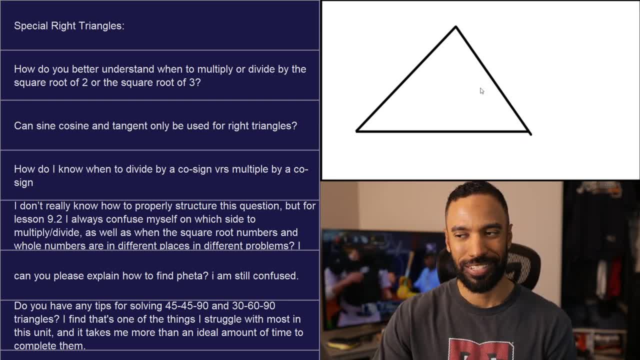 but in one of my recent videos I actually ran into a question. I'm like this isn't and I am two questions- is law of cosines? Let's say that actually almost looks like a right angle right here. But let's say this is like 80 degrees and this was a 50 degree. 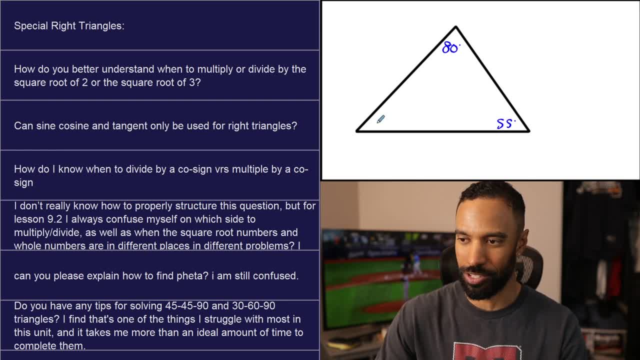 Well, this was a say: 55 degrees and 45 degrees later. Can can trig be used in here? Not in the way that you'd expect, and, by the way, I'm not coming up with more lengths, and whatever the bottom line is, though, 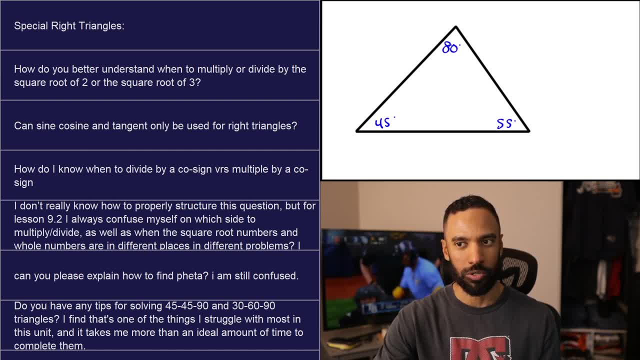 If there is some sort of thing that's used in terms of sine, cosine and tangent- because I could use if this length was, you know, five- I could find this X by using something called the law of signs. There's another formula involved with it. 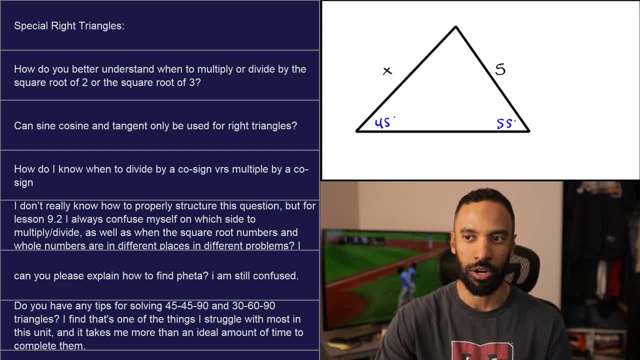 But you know what It's entirely based on it. Just ignore that 80 for a second. I don't really need the 80 for this problem. It's entirely based on the fact that an altitude can be drawn in this part, right here. 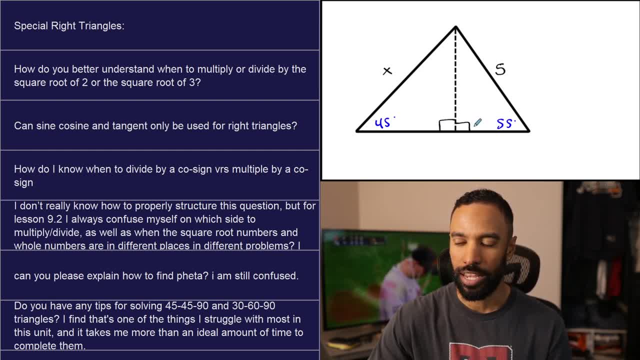 That Divi's up this into a right triangle here and a right triangle there, And therefore sign is used in some way to get gather some H, which is equivalent in both of these things. here Bottom line is: you can use trig and non right triangles. 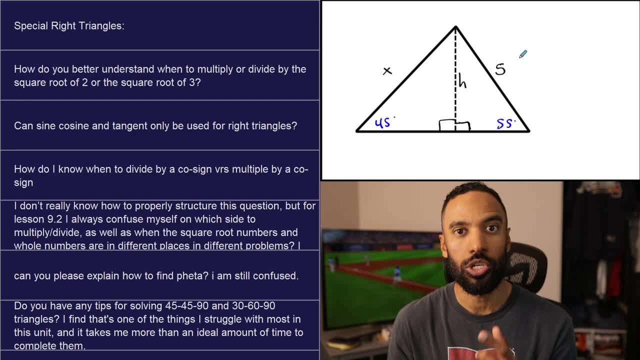 but it's based off a right triangle premise. Even still, even the unit circle- which is something you wouldn't know anything about it, but I am three people will- even the unit circle has a right triangle premise to it, Even though it's a circle. 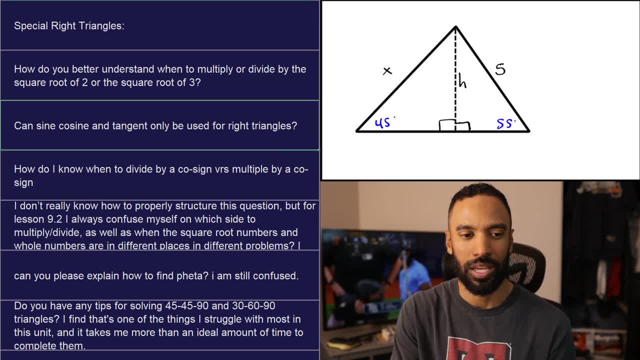 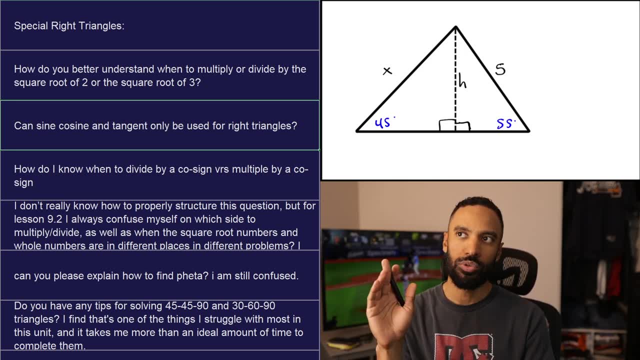 There's still a basis of right triangles that build into it, So can it be only used for right triangles In your sense of the realm? Yes, don't start using. sign is opposite over hypotenuse When I say opposite over hypotenuse for sign. 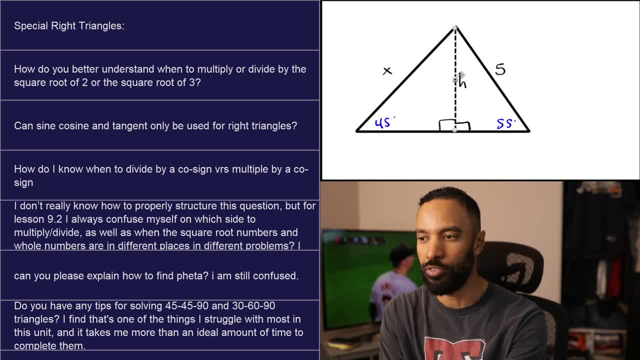 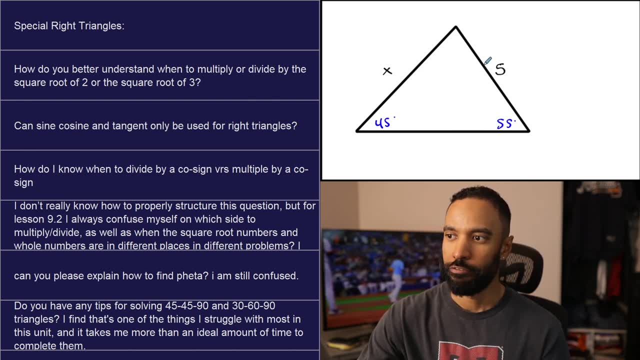 even for this problem. here I'm using it specifically with that altitude. But if you get rid of this altitude you don't start to say sine of 45 is opposite over hypotenuse, Like it's 5 over X. 5 is not an opposite in the way that it's from a right angle. 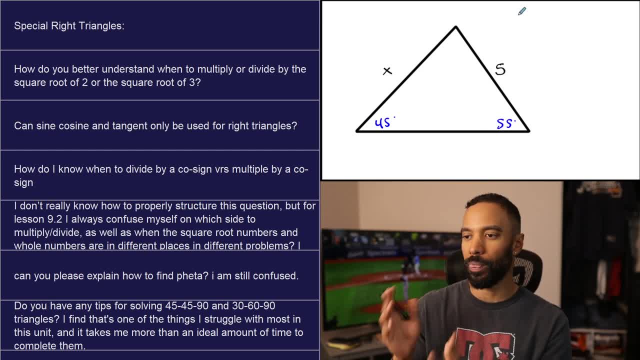 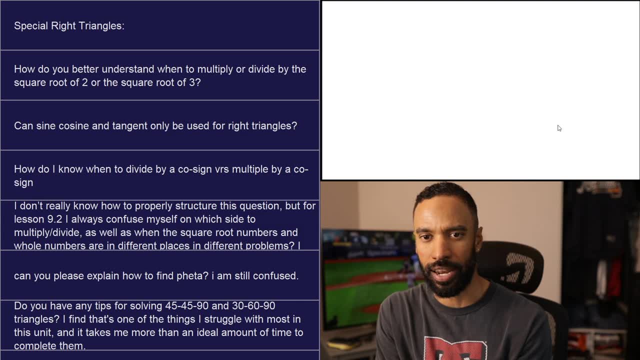 This is not a hypotenuse. It's not a right triangle, So unless you build the altitude, so it's not in the way that you'd think of it when we talk about it, And I don't know if that answers the question fully. 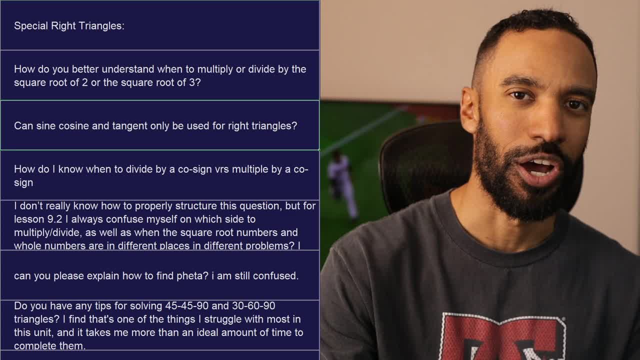 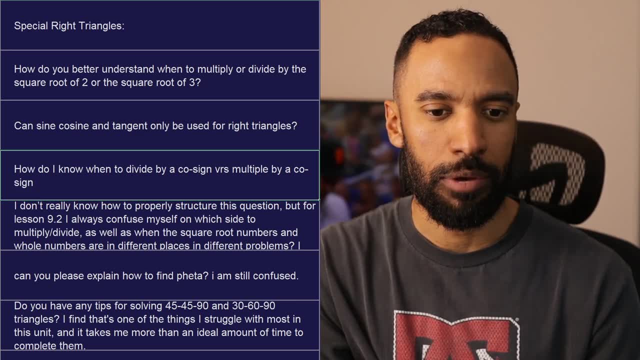 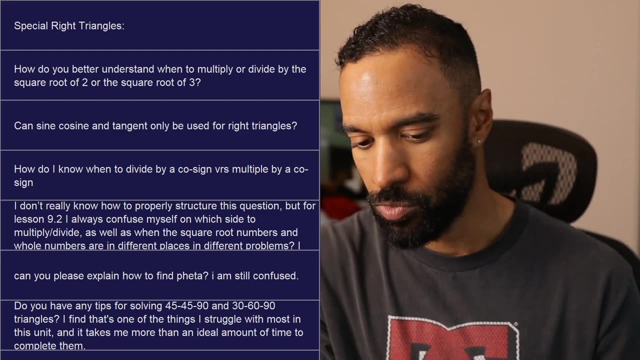 but it should, in a way for you- and I am to know- and I'm three, wouldn't ask the question, because you'd understand that there are other forms that you can. Yes, use it. All right. How do I know when to divide by a cosine versus multiply by a cosine? cosine spelled differently. 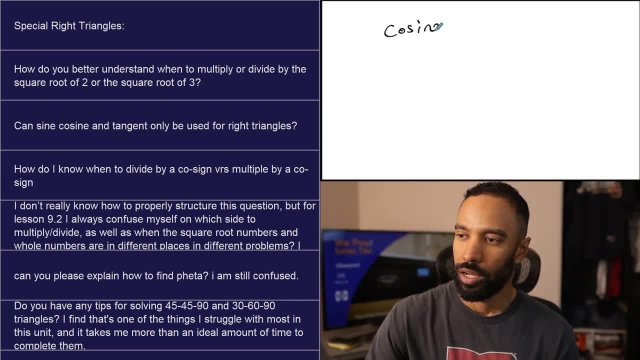 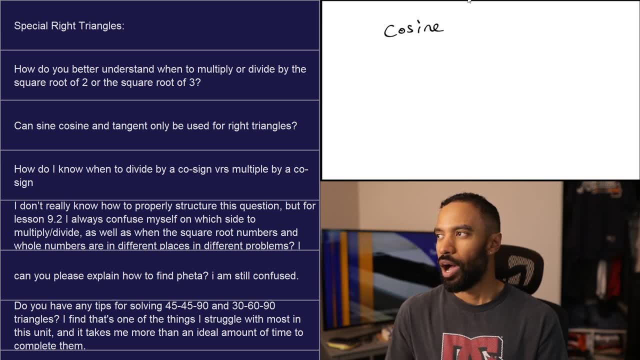 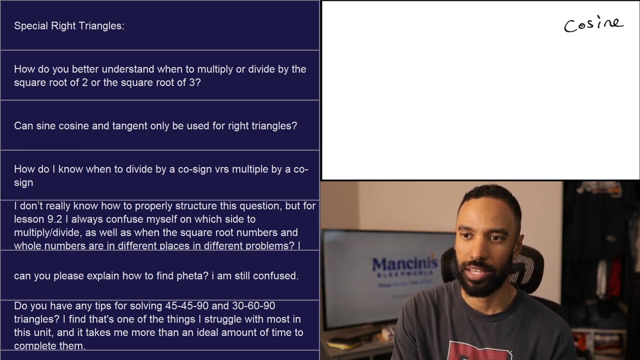 Let's go ahead and spell that one So cosine. Well, cosine instead of sine or tangent. I assume you just mean trig functions. I guess what you're asking is this, Not Okay? I guess what you're asking is this: when you win, in what scenarios? 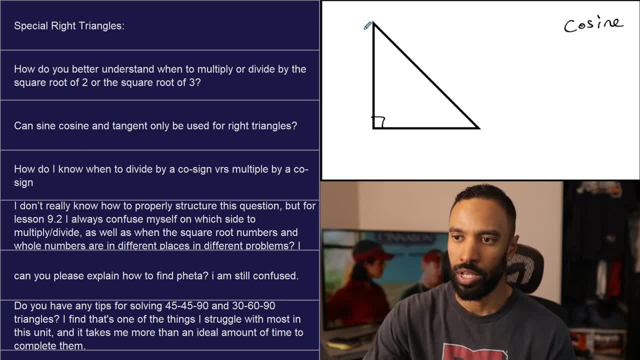 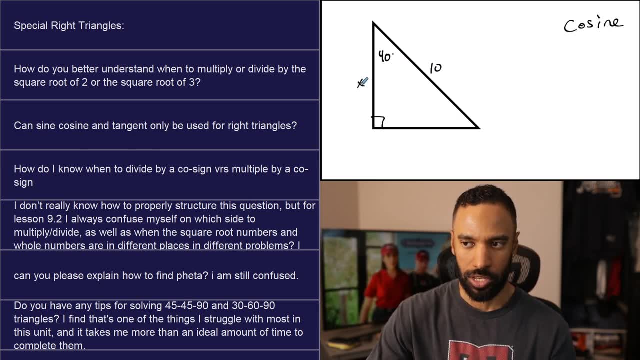 and, and I'll use cosine as the example, I'll use an adjacent and hypotenuse. So let's say this is a 40 degree angle right here, And this is your unknown. and this side length is 10. and they say: solve for X. 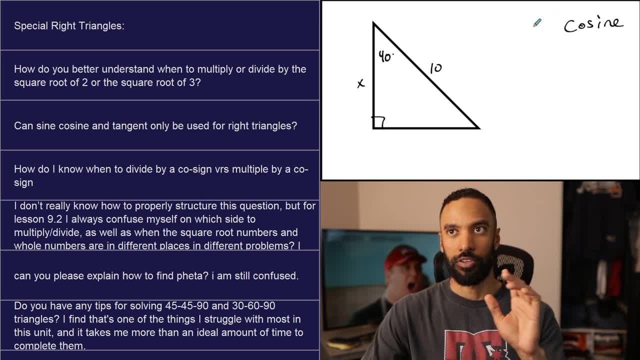 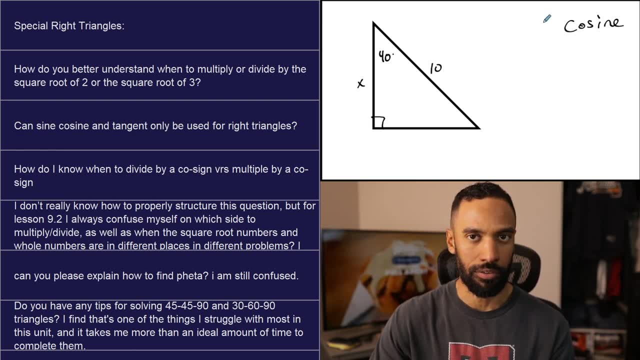 To answer your question, I'm going to say, you know, based off of your setup, your, your trig setup, your trig equation and then what you choose to do algebraically to solve for your variable. So my trig setup for this equation will be this: relative to my 40 degree angle. 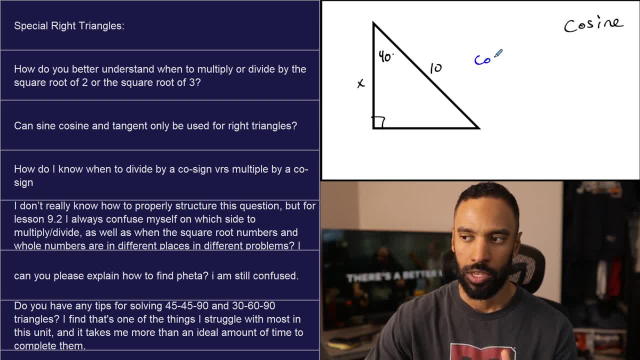 I'm looking for the adjacent. I know the hypotenuse, So I'm going to use cosine. So my setup is cosine of my angle. This isn't cosine times, By the way, if this is what you're asking. I'm just going to say this is not multiplication. 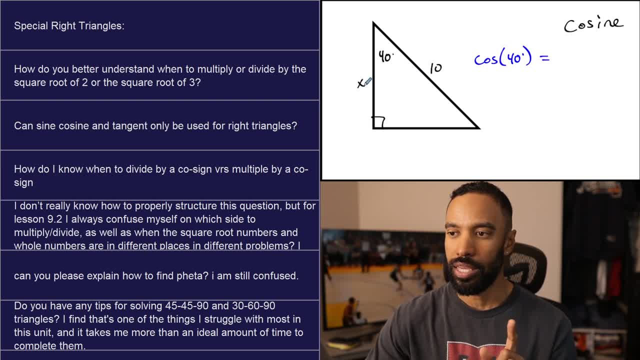 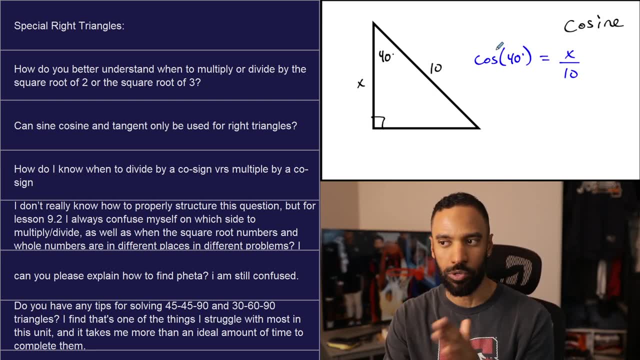 This is applying a function, but I don't think you're asking that equals adjacent over hypotenuse, X over 10.. So your question might be: how do I know that I multiply 10 by cosine of 40 instead of divide it with cosine of what you know? 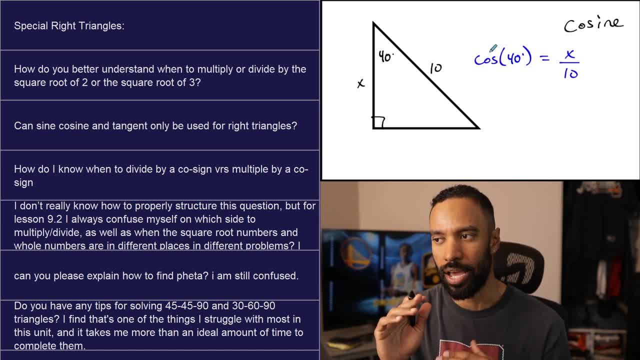 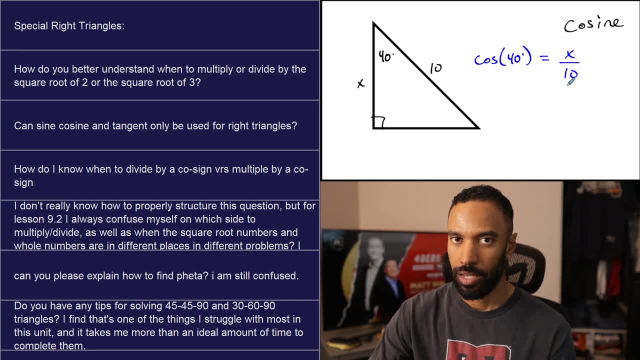 something like that. That's what I think you're asking, And my answer is: you got to know your algebra based things. X is what I'm solving for. X is being divided by 10.. In order to solve for X, I got to multiply both sides by 10.. 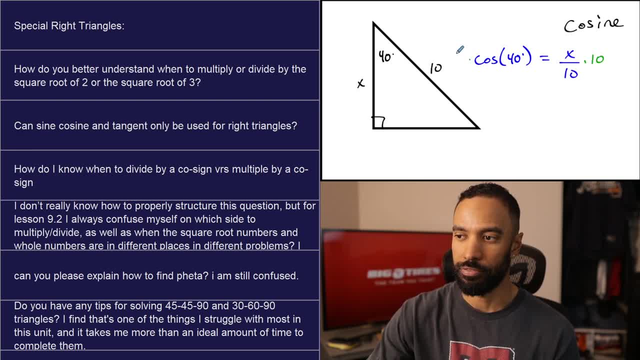 That's. that's the setup. to get X by itself, 10 has got to be multiplied, So 10 is multiplying with the cosine of 40 in this case. right, Here's the exact answer for X. I'm just going to leave it like that. 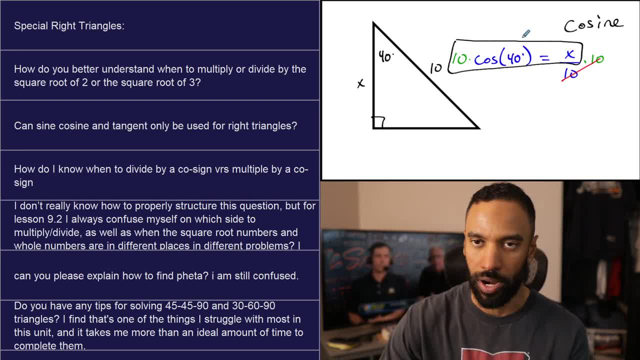 X is 10 times the cosine of 40. Whatever that calculates to is whatever right. Let's flip the script on that one, though, And let's go to. let's put 10 here and X here. completely different question Now, by the way. 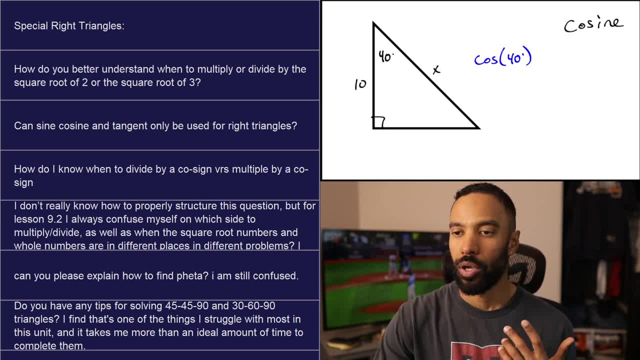 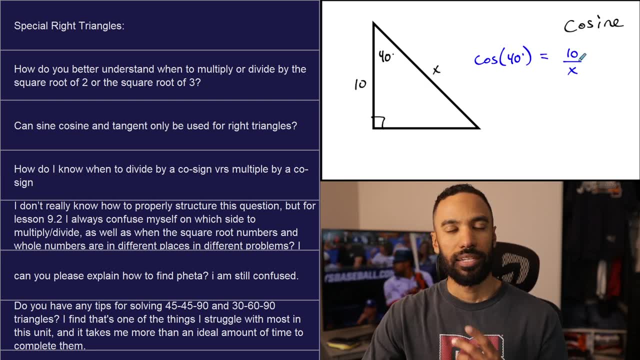 it's not like: whatever was X before, is X now Cosine of 40? in this case, now equals 10 over X, adjacent over hypotenuse. But now the X is here. Technically, it takes two steps to solve for X, to get X by itself. 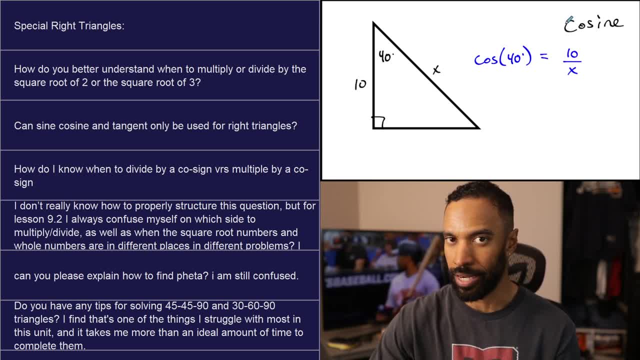 The first step doesn't actually get X by itself, But in order to solve for X, you got to get it in the numerator of its own question. You got to multiply both sides by X, same way as we multiply both sides by 10 differences. 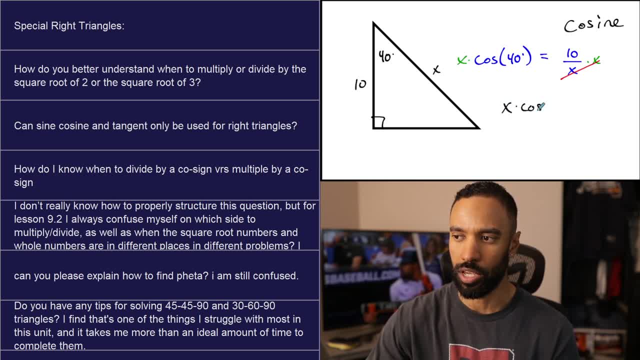 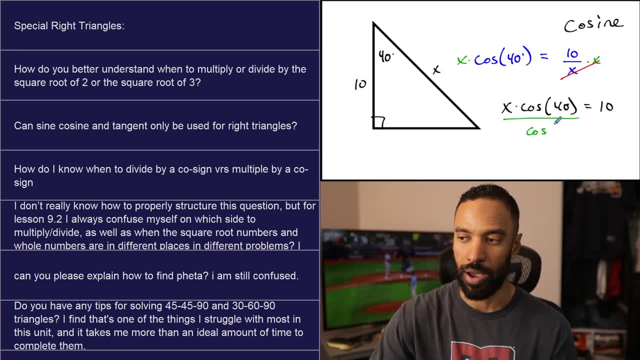 X is not yet by itself. Now this equation says: X times the cosine of 40 equals 10.. And you might say: well, or multiply my cosine of 40 again. Well, not so fast. Now we're going to divide both sides by the cosine of 40 to get X by itself. 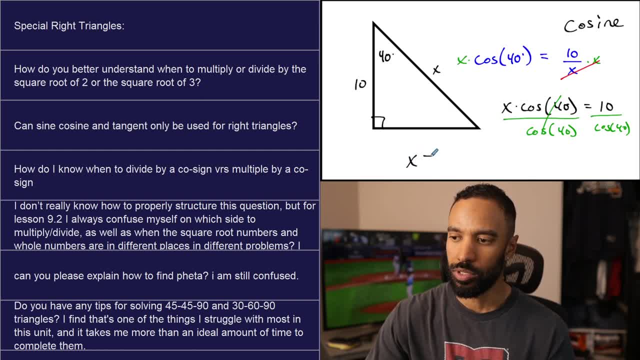 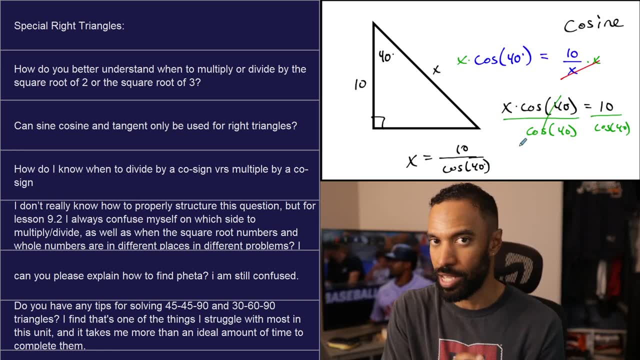 So in this case, X equals. X equals 10 over the cosine of 40. And whatever that answer is is what it is now: 10 times the cosine of 40 is going to be a number less than 10. 10 divided by the cosine of 40 is going to be a number greater than 10.. 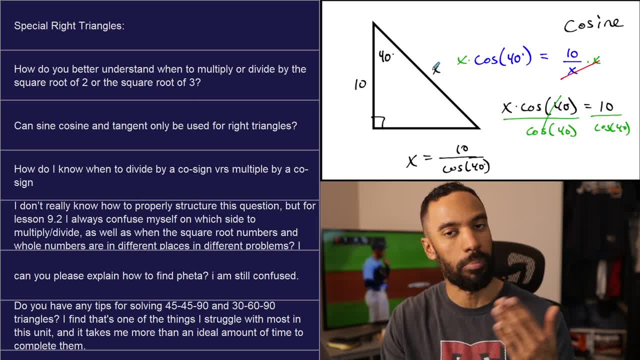 The reason. I know that is because in this case X is the hypotenuse. hypotenuse should be greater than a leg. So when you ask- and last time X was the leg and 10 was the hypotenuse- So when you ask, 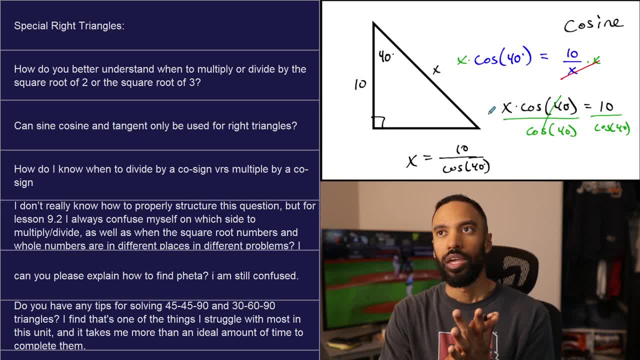 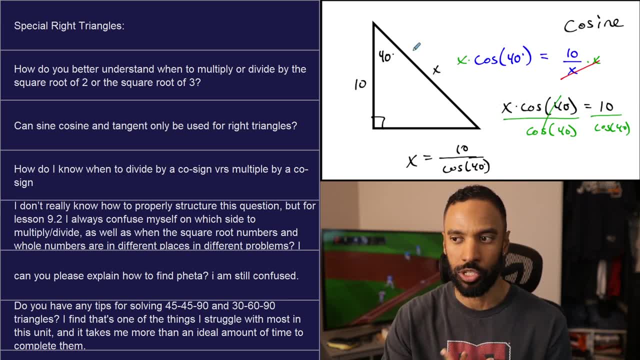 how do I know when to divide by cosine and multiply by cosine and things like that You part? part of the answer is: whatever value you get in your calculator. Ask yourself whether it's a red flag answer If I end up getting an X value of 7.6,. 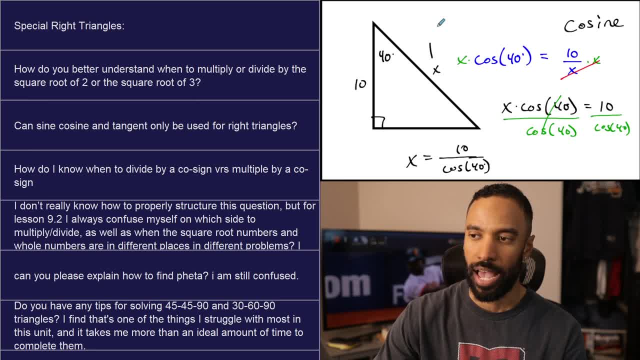 something went wrong because I should get a hypotenuse. It's bigger, So you got to ask yourself: did I do the right algebra to get there? In this case, this will be bigger than seven points. I don't know, I don't care what it's going to be. 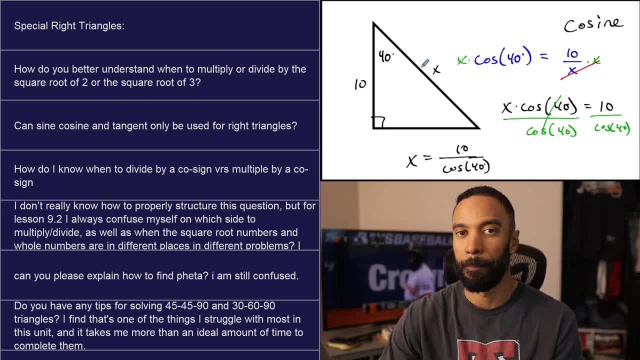 but it's going to be something bigger than 7.6, is going to be bigger than 10. And it should be. And if it was less than 10, something went wrong. So that can help answer it as well. How do you know when? 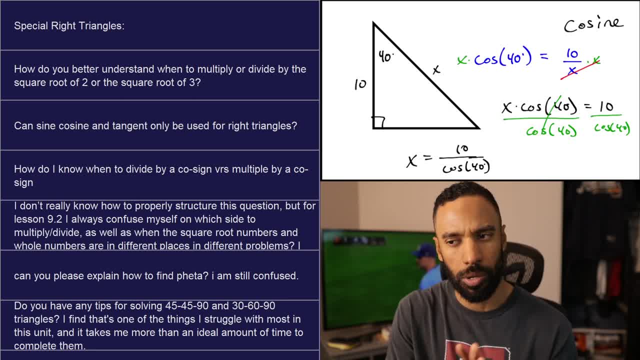 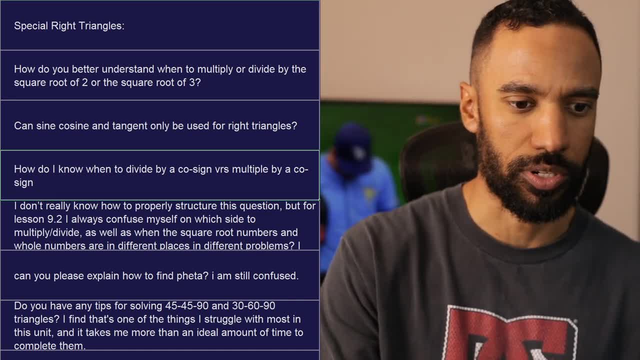 Well, you should also know the size of your numbers in comparison, and hopefully that somewhat addresses it. Okay, I don't know how many questions I have left here. I never did check, but these questions are kind of big. I don't really know how to properly structure this question. 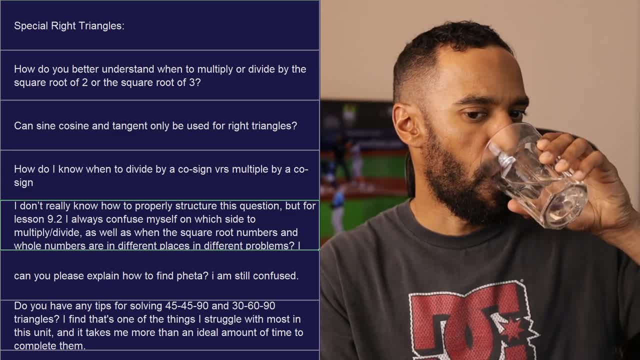 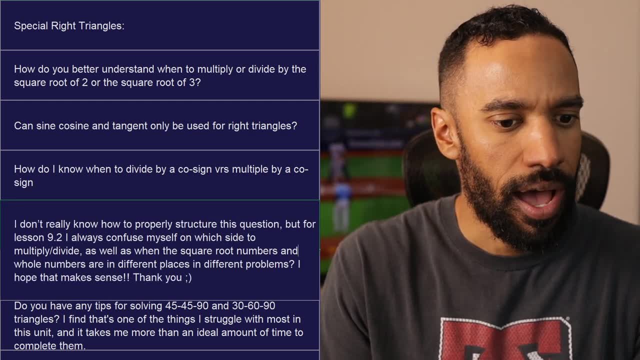 but for less than 9.2,. I was confused myself in which side to multiply, divide, as well as when the square root numbers and whole numbers are in different places in different problems. I oh, was there more? I hope that makes sense. 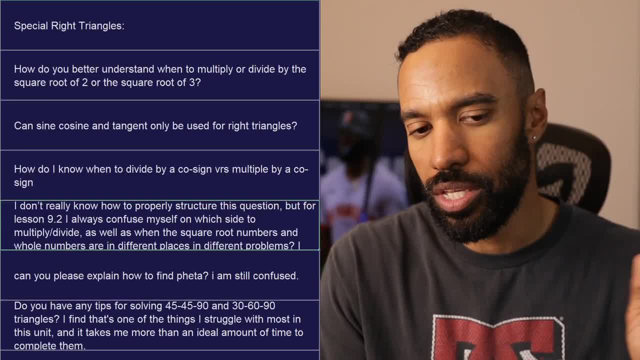 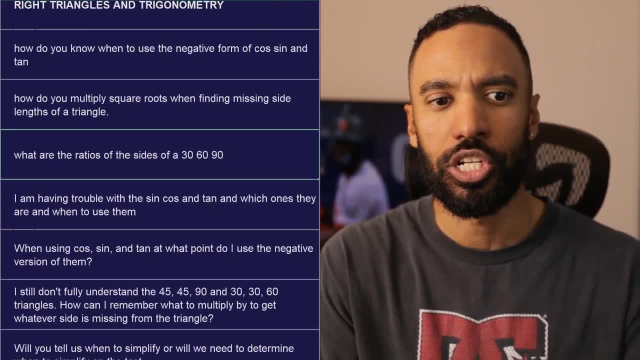 Thank you. Yeah, mostly what I'll say is- I did answer it several times- just by setting up ratio relationships, I might have even done a problem. Check out these questions here. This one: the ratios sides of a 30,, 60,. 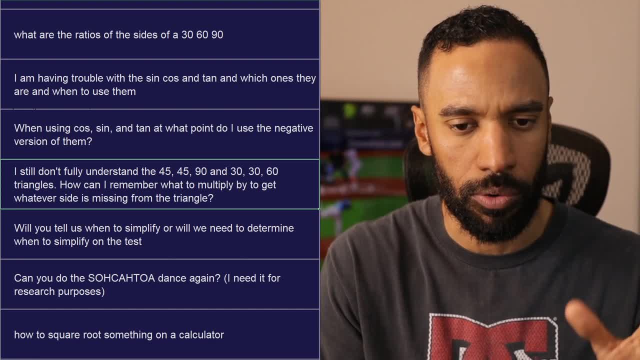 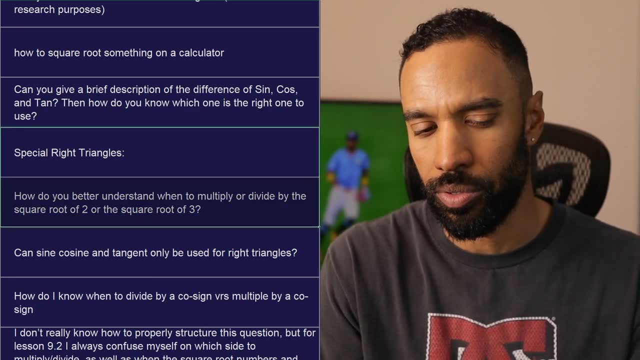 90.. This one on the 45,, 45, 90,, 30,, 60, 90.. They said it wrong, but 30,, 60, 90.. And then this question here on how to understand when a multiplier divide by the square root of two or square root of three. 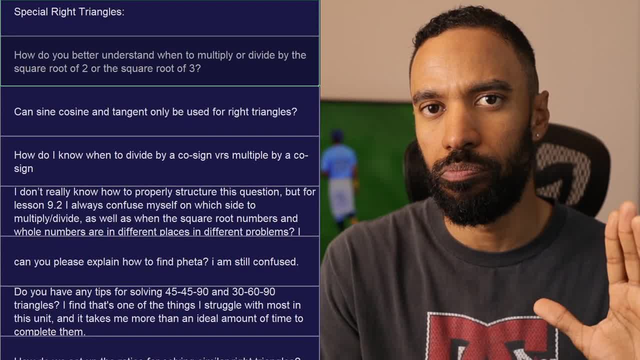 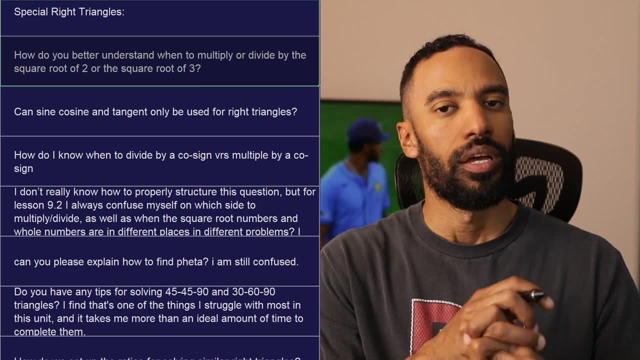 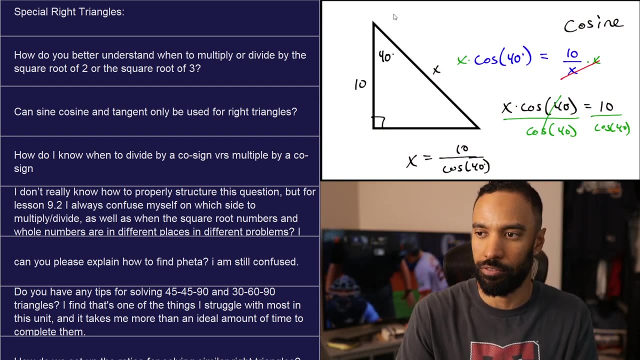 But once you you've built what, once you've drawn that triangle ratio relationship, it's hard to get it wrong because, well, well, here, here I'll answer it in a different way. You can still take those answers, because this is going to be a different way for the. 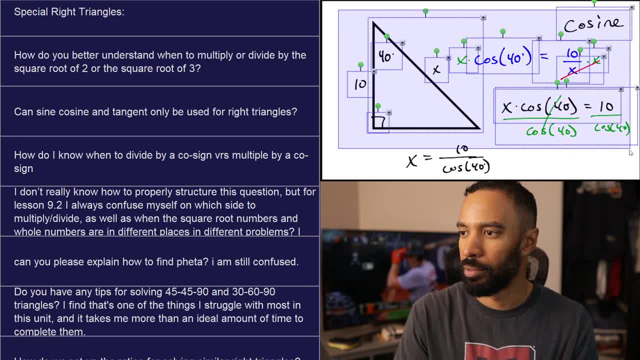 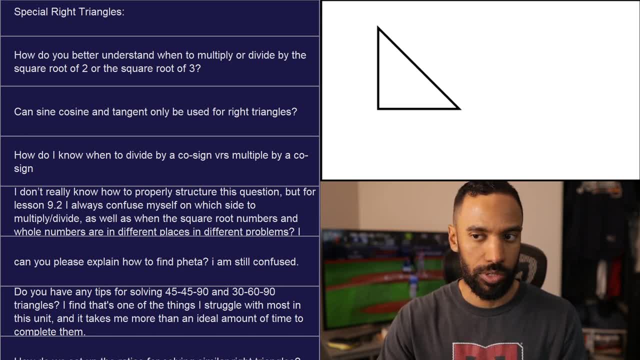 for me to answer it. What did I just do? Um, remember, this is all about similarity, is all about similarity. I'll do it with just one example, and then I'm going to cut it. Um, so 45,, 45,. 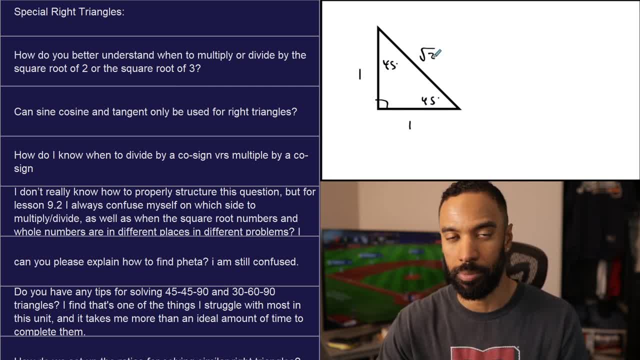 90, this ratio relationships one to one to root two. Why? Because it is Pythagorean theorem, isosceles, right triangle, all this kind of stuff we can get there Now in your that's. that's just the ratio relationship. 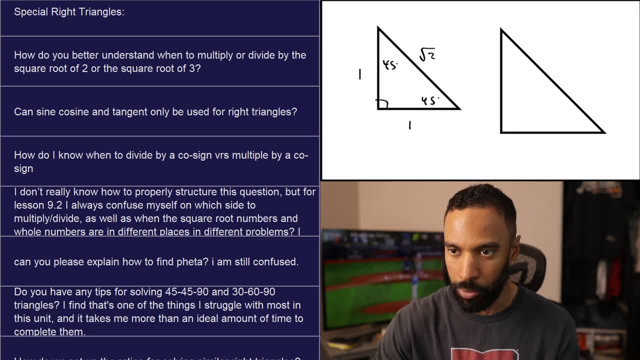 This applies to any right triangle. So when you get a right triangle as an example, when your example says a 45 degree angle here, it shows a right angle there and it shows a length right here, of, because I want to rationalize denominators. 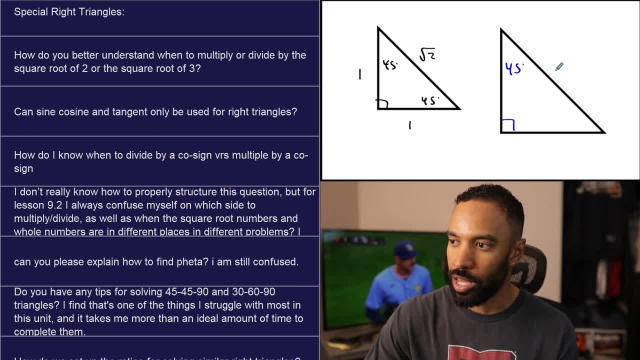 I don't know if anyone's going to ask me about it later. Our uh length of two. uh, I want to get something good. Uh, nine root six, Actually, that's not. that's not good enough Um. 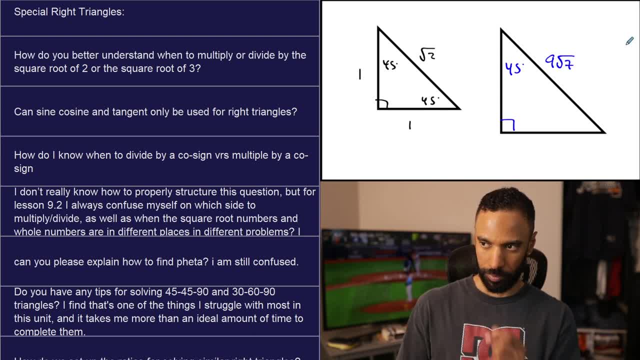 nine root. I'll just do nine root seven. Excuse me, Let's do eight root seven. This is what happens when I come up with something on the fly and it says solve for the length of a. solve for the length of a. 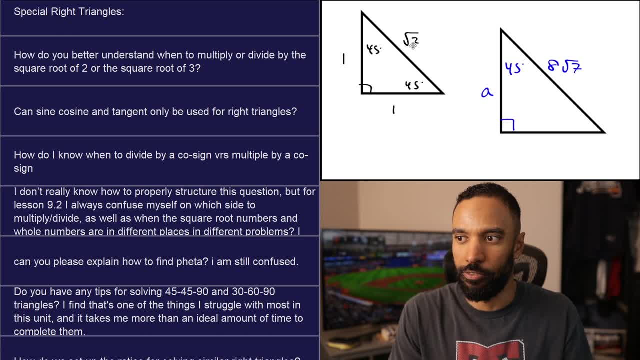 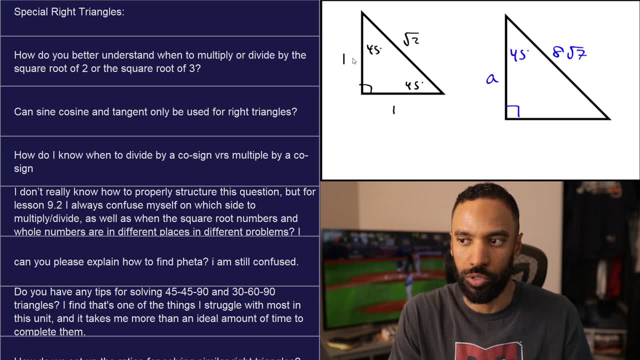 Well, the way I would say this before is straight up, as, as I would generally say, it is root two, is root two times larger than one. So to go from root two to one, you divide by root two. So you would divide this number by root two and you'd get a. 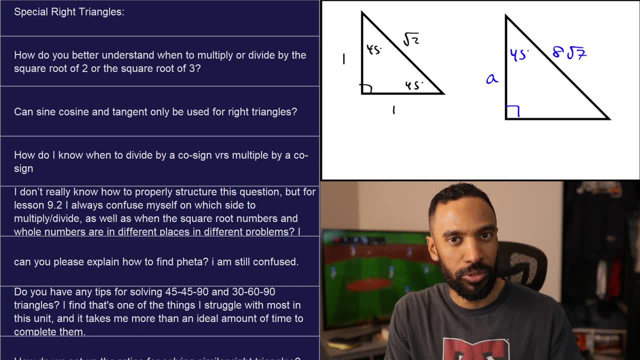 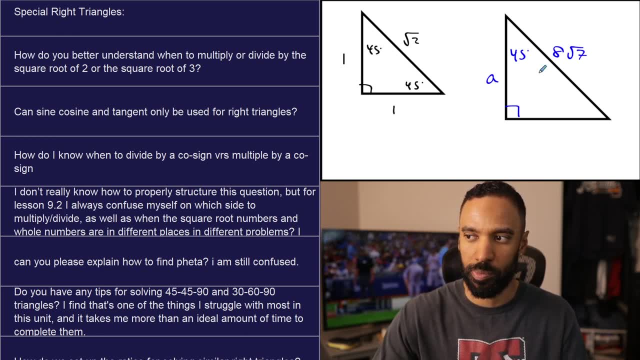 but you don't have to go about it that way. What we know about similar triangles is: corresponding sides are proportional, So we should know that this leg corresponds to this leg, This hypotenuse corresponds to this hypotenuse. You can make a proportion out of it. 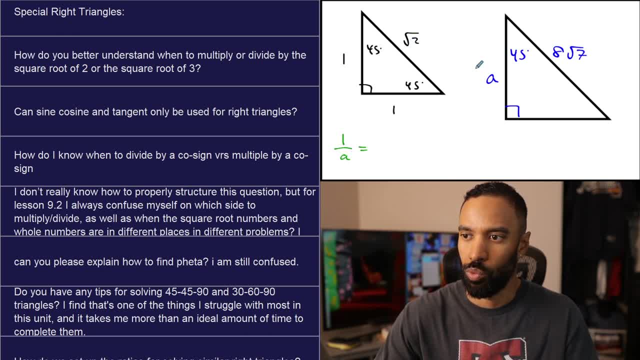 I can say something like one over a equals one over a equals root, two over eight root seven. I mean, this is just another way to go about the problem. Cross multiply all that kind of stuff, You get eight root seven equals a root two. 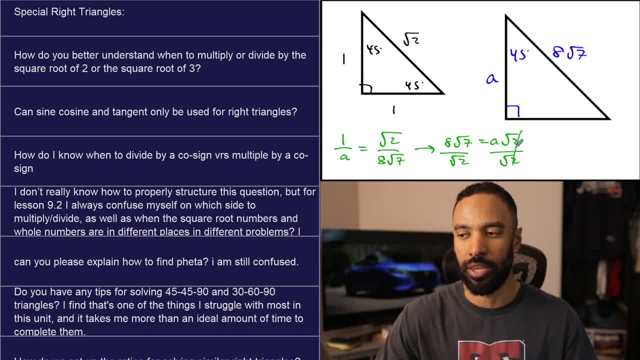 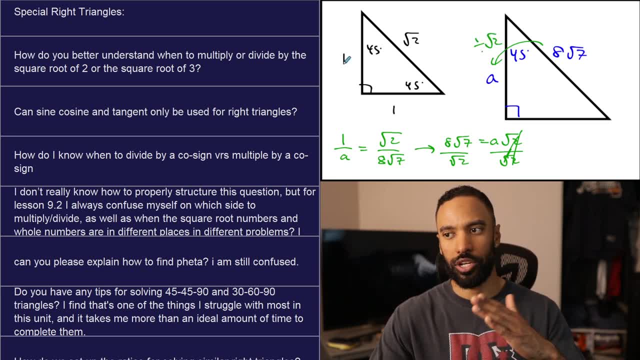 divide both sides by root two, but that's the ultimate thing that happens. You divide by the square root of two. This is the square root of two times smaller than that guy. So once you know these ratio relationships, use them with the parts that correspond and say: 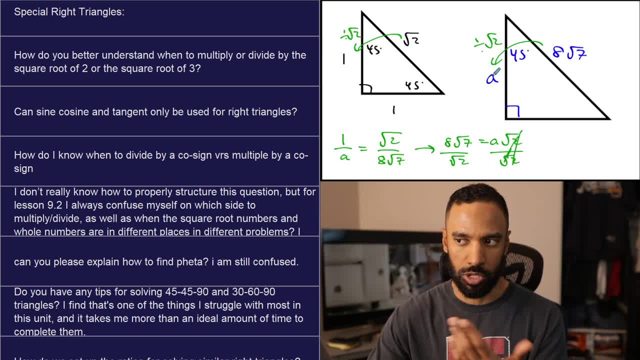 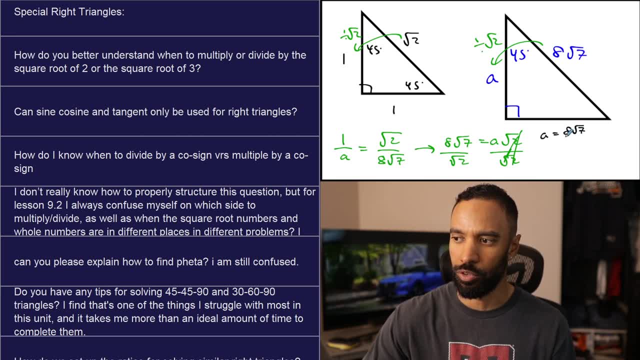 I'd have to divide this by root two to get that number. So I should divide this by root two to get that number. It's that kind of thing. Anyway, I'll just continue on the problem. A is eight root two or eight root seven over root two. 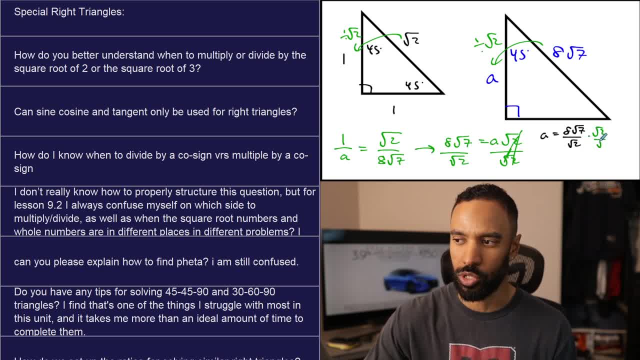 And I got to rationalize this denominator. Multiply top and bottom by the square root of two, And then you get eight root fourteen, Eight root fourteen over two, And eight over two is four. So you get four root fourteen and root fourteen. can't simplify. 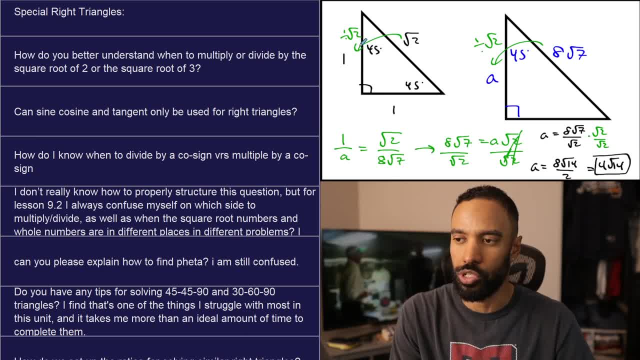 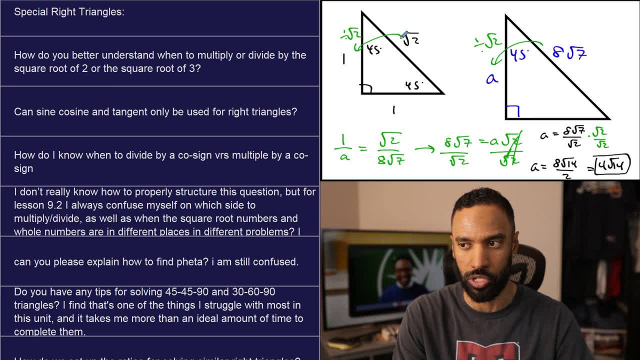 And that would be the value of a. I don't know, but that's, yeah, you, just you. the reason why we do the one to something is because one is the smallest Integer, and then I know that one times anything is just that number one times. 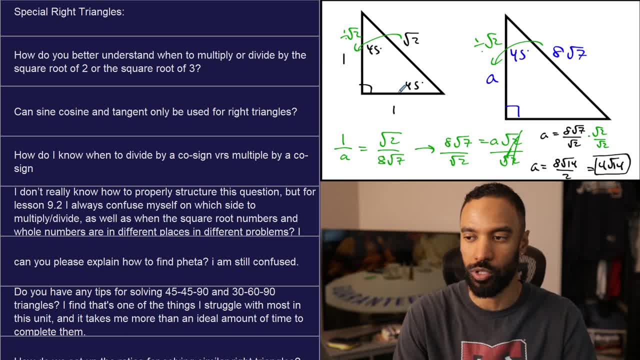 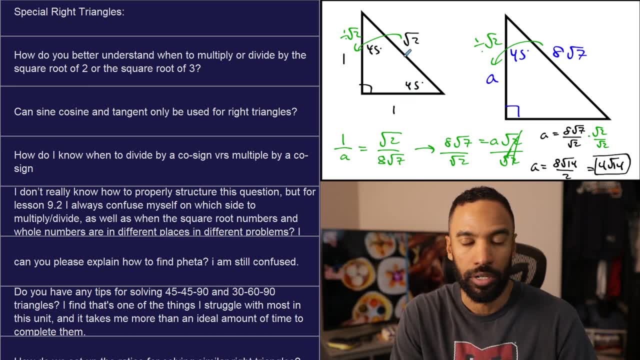 What is root two? root two, one times. What is two to one times? What is root three? root three. So it's easy to come up with. based on that value, What do I do, Or what do I divide by, to get one, that number? 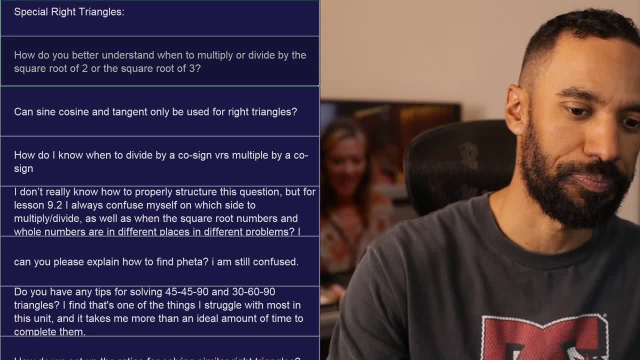 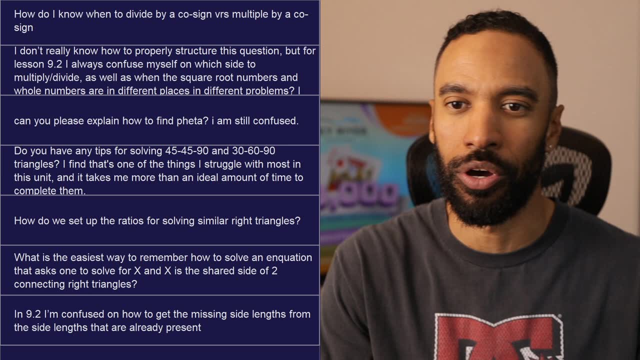 Yeah, And that goes based off all the other questions before. Where was that question? Okay, it was there. Can you please explain how to find theta? I'm so confused. was theta, Although sorry if I ever speak with a lisp of any. 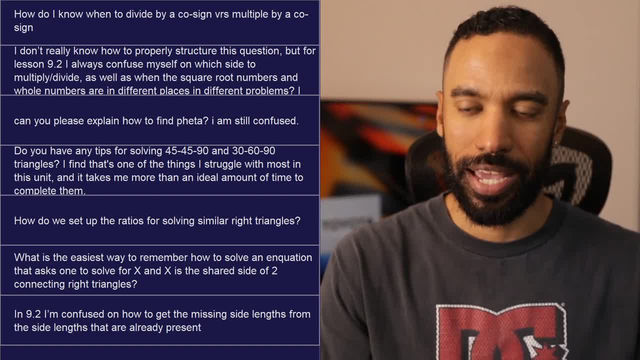 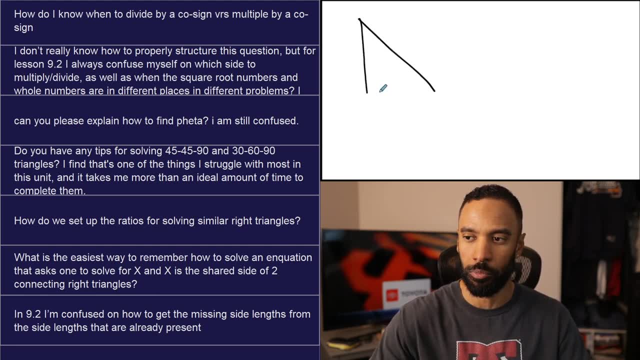 Or that makes you not sure what I was saying. Theta is just a variable, but we use that variable for angle measures, So you're probably going to see it on more quizzes and tests. So how do I find theta- theta, by the way, theta. 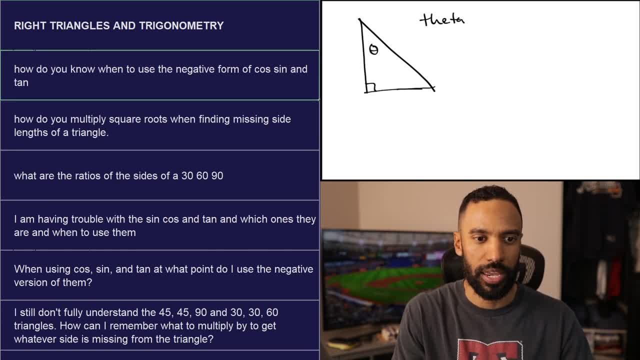 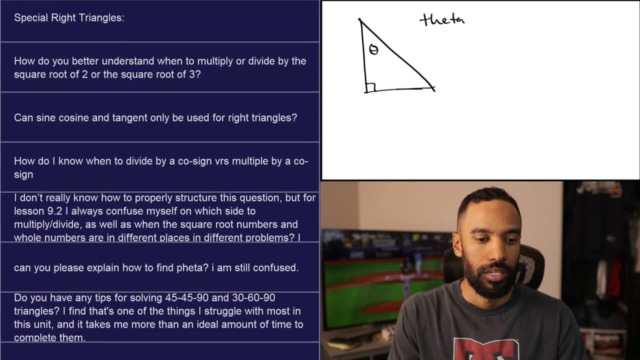 It's a Greek letter. I answered it on the top question right here. How do you know when to use negative form of cosine, sine and tangent? It should say inverse sine, cosine and tangent. but that's to do. Where is it? How to find it? 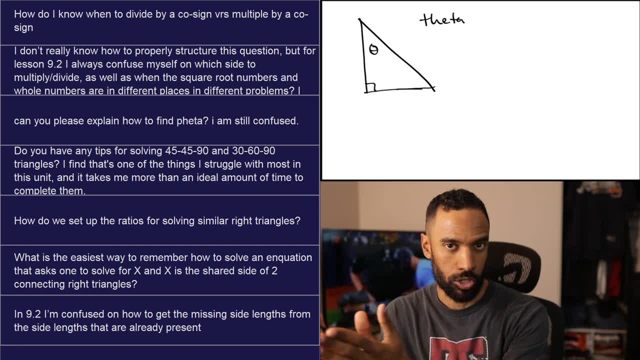 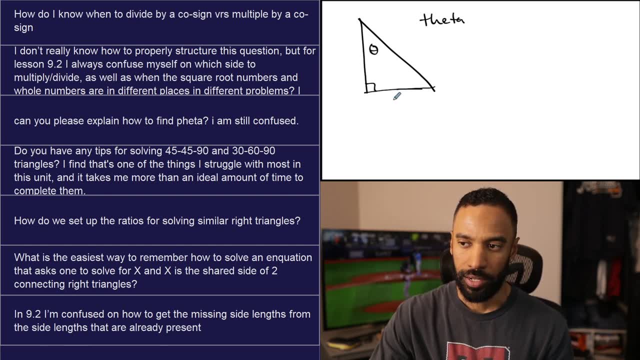 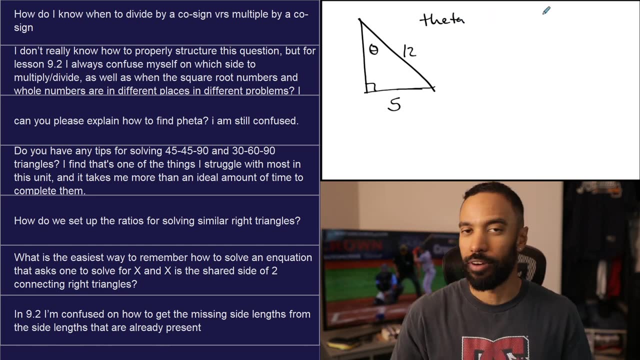 The idea of finding theta in angle measure is going to be in one of your trig based questions when you already have certain side lengths of your triangle. So let's say I had 5 and 12 right. here I want to set up a trig function. 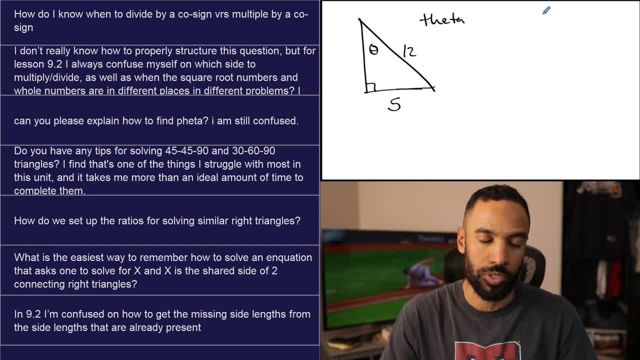 I want to set up a trig equation, the same way I would have if I knew what theta was and I was trying to find one of my side lengths. Since you didn't ask about the finding the side lengths thing, I assume you know something about that. 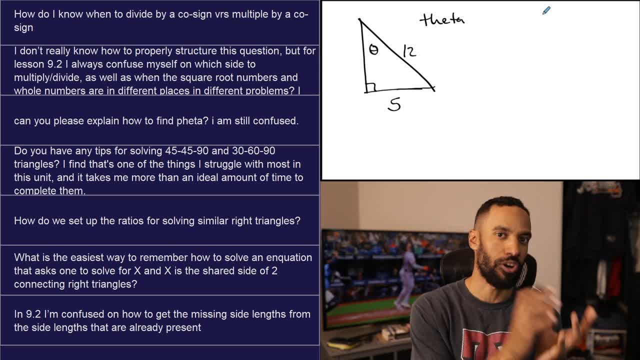 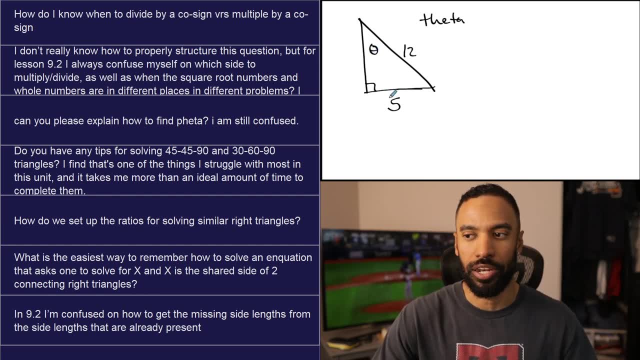 but here's the thing: You take sine, cosine or tangent of an angle measure and the result is ratio. So let's set that up. What do I do Sine, cosine or tangent with here? I know the opposite. I know the hypotenuse. 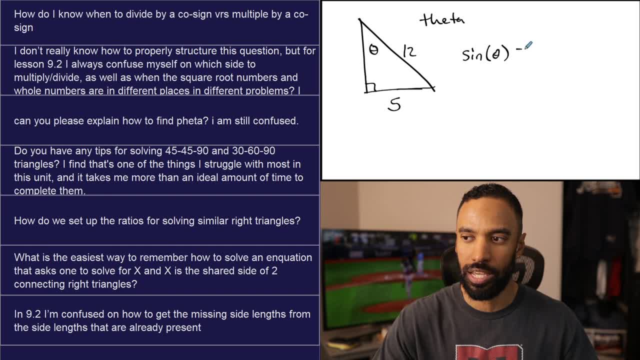 I want to use sine. So I say the sine of my angle equals 5 over 12.. Whatever angle I'm taking the sine of, I get the same as whatever 5 over 12 is. See 5 over 12 is some random number. 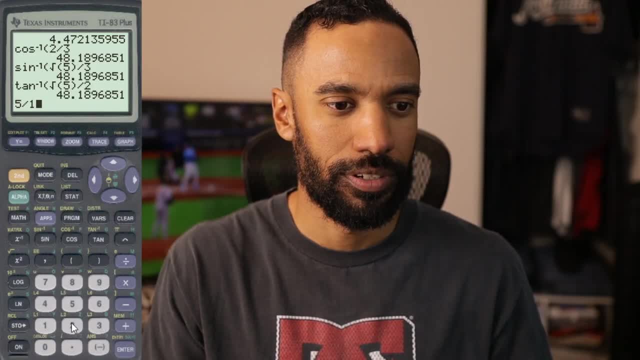 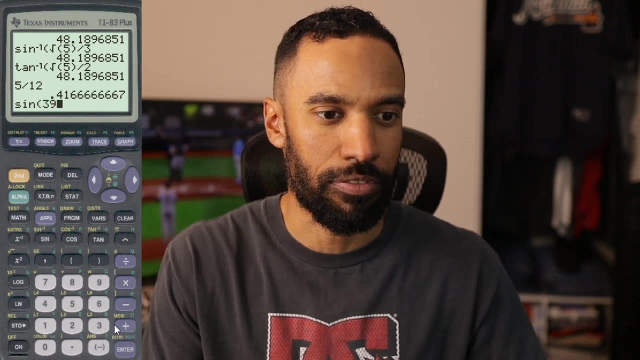 It really is to us. 5 divided by 12 is that crazy number. There's an angle that I can take the sine of to get that same number. I don't know what it is. Let's try the sine of 39.. 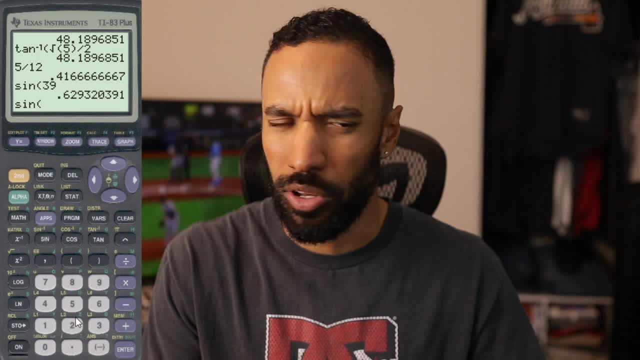 Let's see what that gets us. Not even close. Let's do the sine of: would it be a smaller number, 20, 25.. That was actually pretty close. So it's close to a 25 degree angle, right. 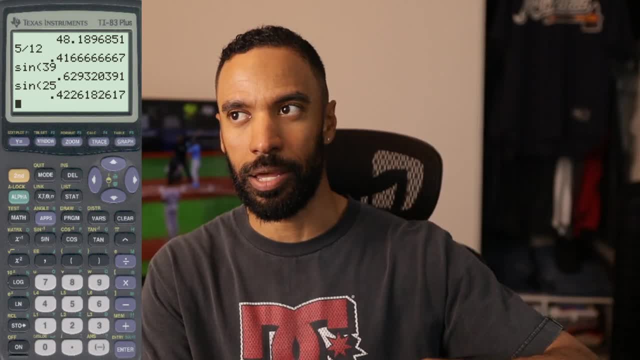 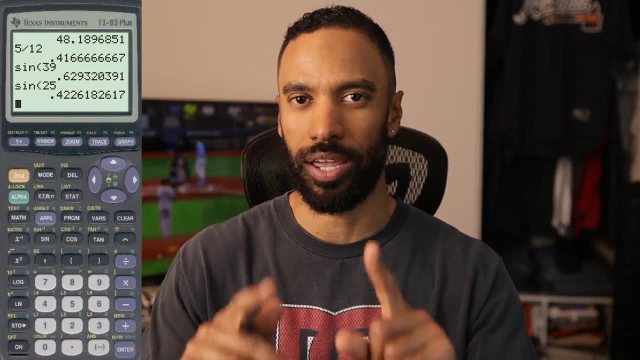 That's not what I do to find it. I'm just saying that that's the idea. You're taking the sine of an angle. You get some sort of decimal value. The decimal value is equal to the ratio of the two values That we're using in our triangle. 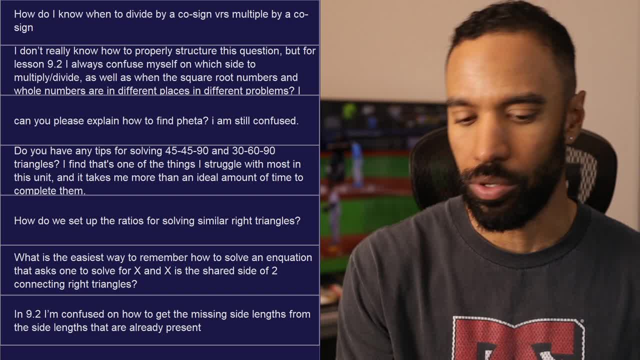 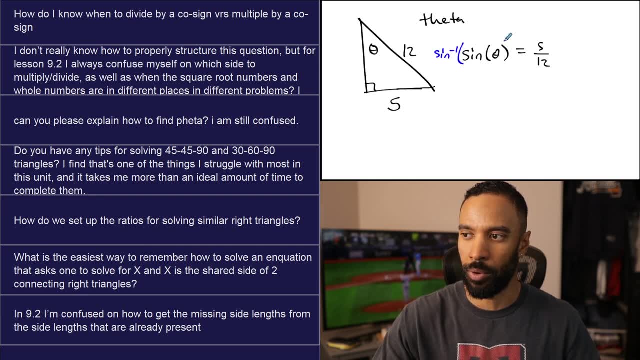 So how do you find that angle? How do you find that angle? We whoops? we have to take the inverse sine of both sides, The inverse sine. That's why I wanted to point to that negative thing. Inverse sine cancels out that thing right there. 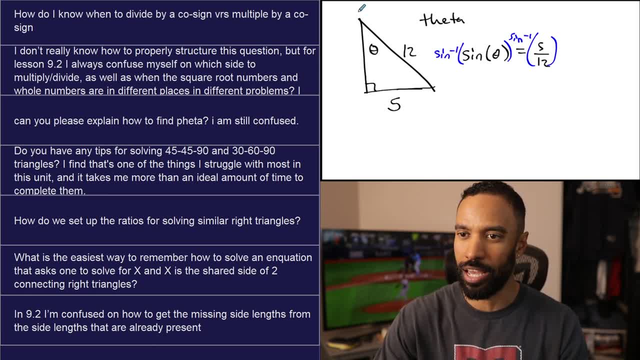 So theta, the angle measure, is now going to be alone, because the inverse sine of the sine of an angle is just the angle itself. So now we get, theta equals the inverse sine of 5 over 12. And your calculator will find the angle measure that you got to take. 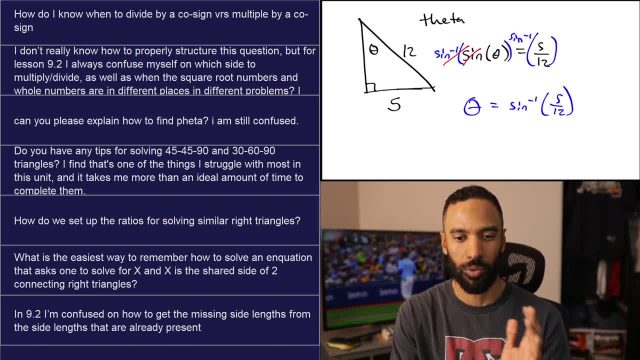 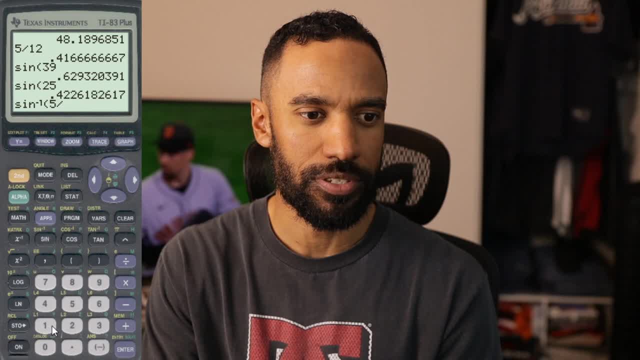 Take the sine of to get you that same 5 twelfths ratio or that decimal equivalent of it. So the inverse sine, and it'll be something close, It'll be a little bit less than 25.. Inverse sine of 5 twelfths is 24.. 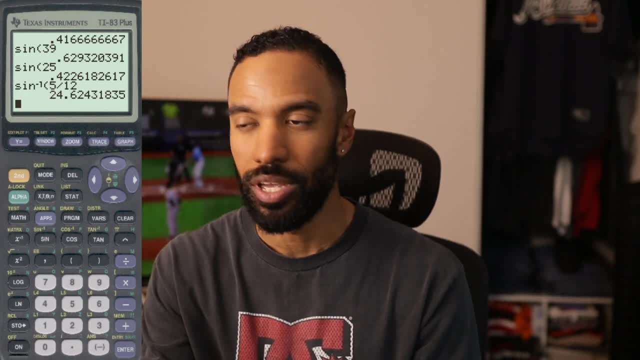 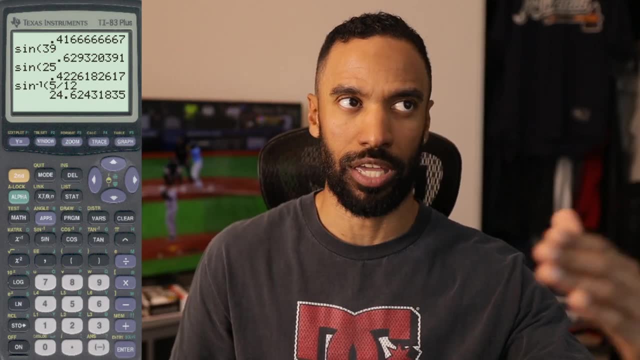 That was very close, Like yeah, pretty much 24.6 degrees. That's how you find it. Inverse trig functions: That's the whole point of them. So go back to your notes, Find the part where it says you take the sine of an angle to get a ratio. 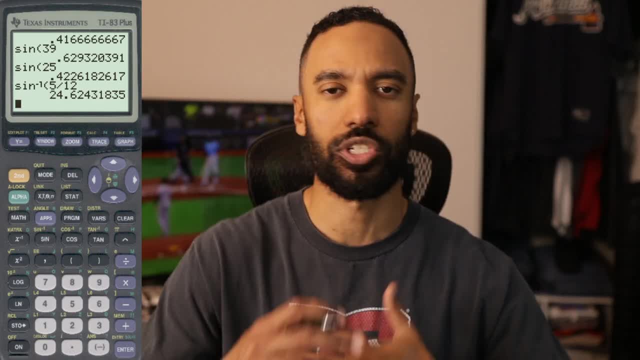 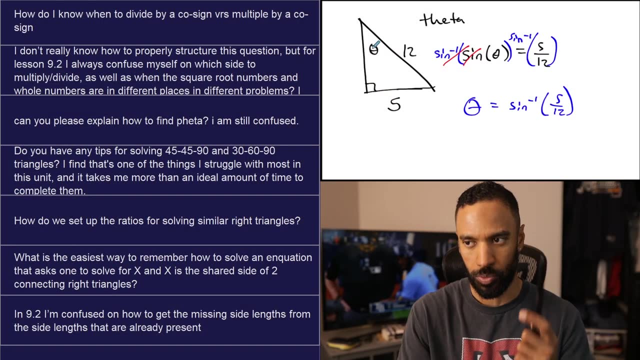 Take the inverse sine of a ratio to get an angle, Or inverse cosine or inverse tangent. But it depends on which setup you have. This I would use sine because with this angle it's the opposite, in hypotenuse, Like that Tangent would be opposite over adjacent and all that. 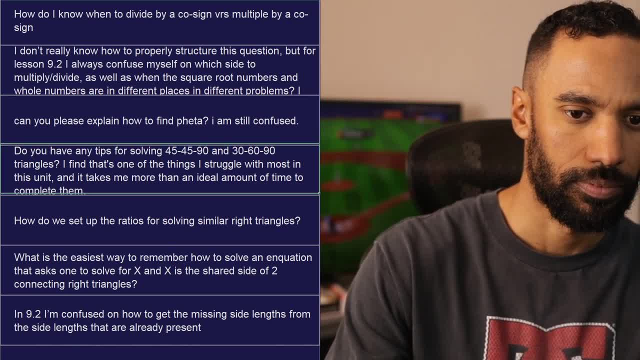 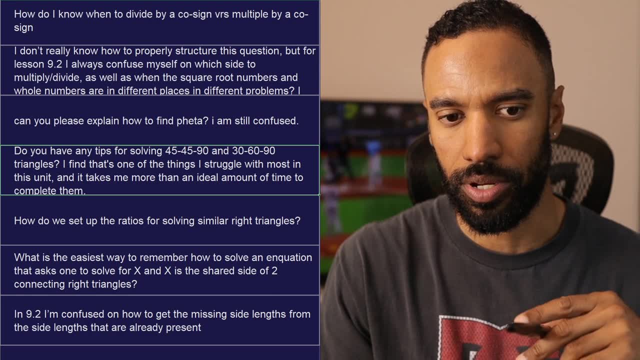 Okay, The next question: Do you have any tips for solving 45,, 45,, 90,, 30,, 60, 90 triangles? I find that's one of the things I struggle with most in this unit. It takes me more than an ideal amount of time to complete them. 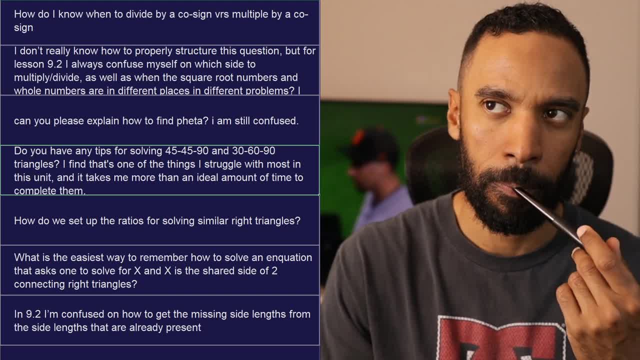 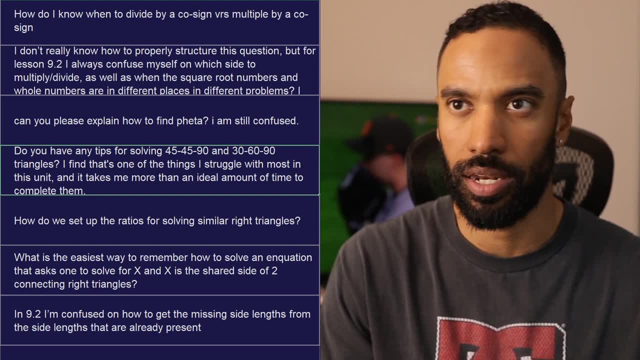 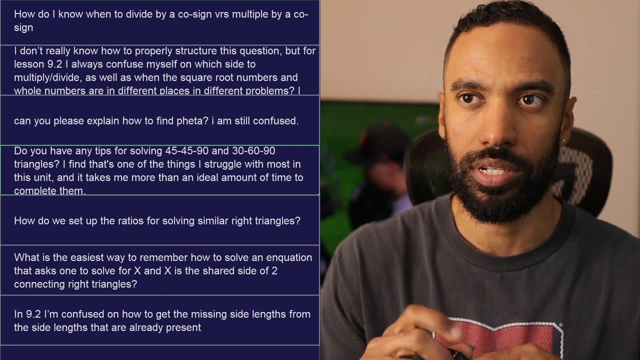 All I will say is I have answered it several times here. If you haven't tried the assignment- because I think the assignment I gave you was a worksheet And look it might have had a video on it. It might not have, But if you want to just see more examples of them, I would say go to the textbook version. 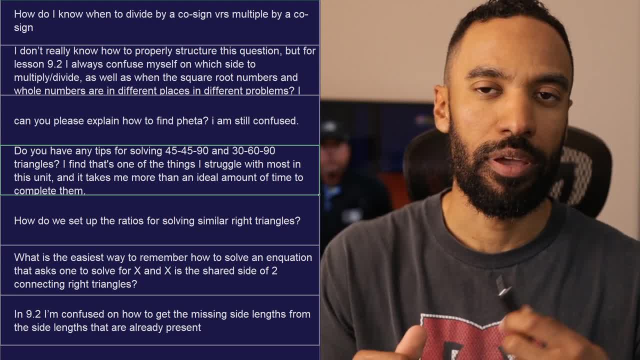 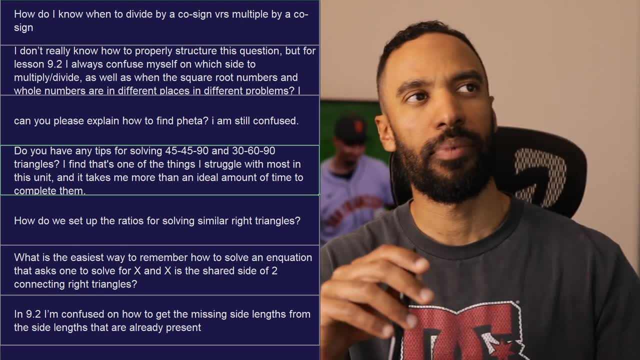 Like: go to 9.2 in the textbook, Find my video. Find my video in my IM2 playlist of the 9.2 textbook video stuff. You'll see that I do them really quickly. If you're talking about the simple, if you're talking about the using the ratios, that's what I'd recommend. 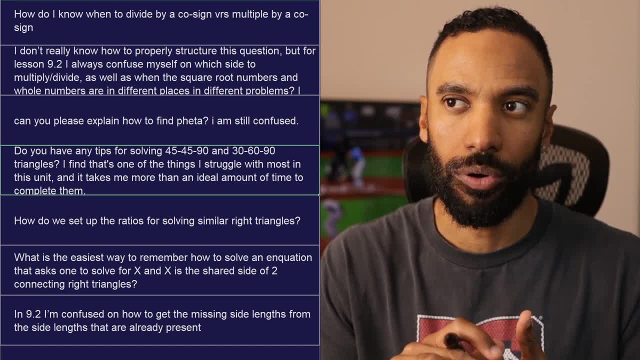 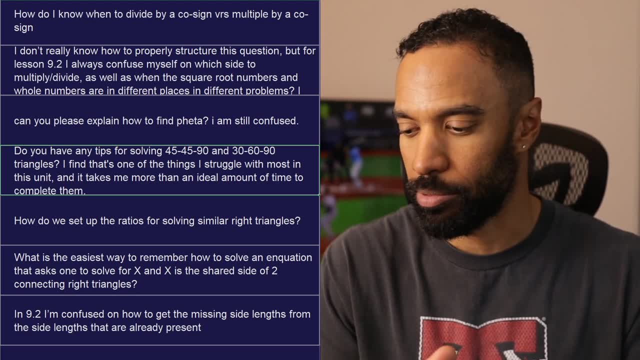 If you're talking about simplifying radicals. I don't know if I teach that stuff there. I just do it Because I taught that back in, I think, chapter 4.. I think I brought up It's back in chapter 4.. 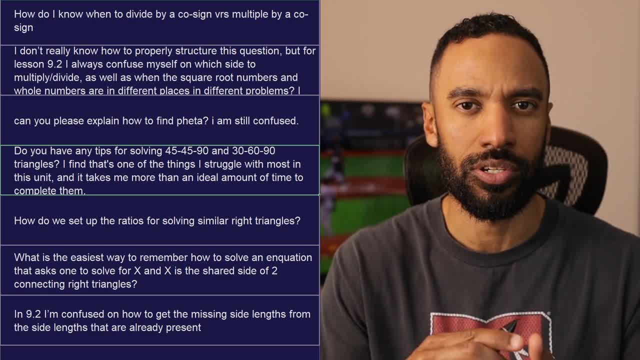 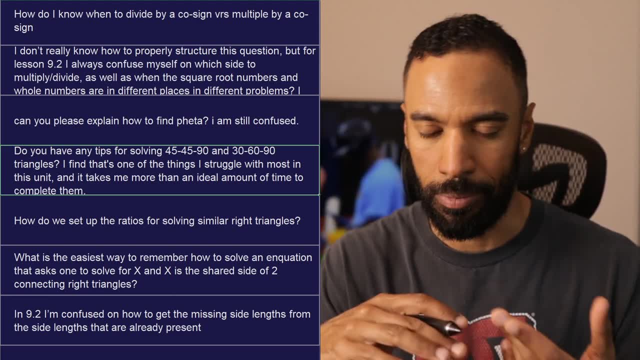 So if you're asking more about simplifying, radicals, rationalizing denominators- we got to look back a little bit on that. But it's very quick. You multiply by 2 or divide by 2.. You multiply by root 2 or divide by root 2.. 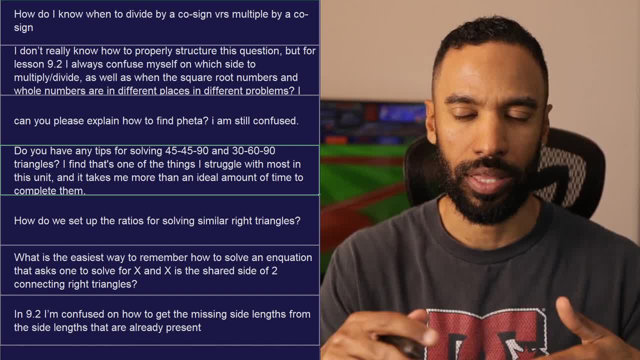 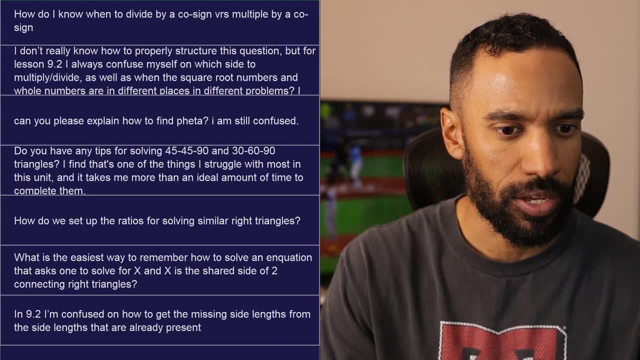 Multiply by root 3 or divide by root 3.. All depending on which triangle you're in and what the buildup is. So go to the other questions that I have here. Anything else that talks about 30,, 60,, 90,, 45,, 45, 90, special right triangles. 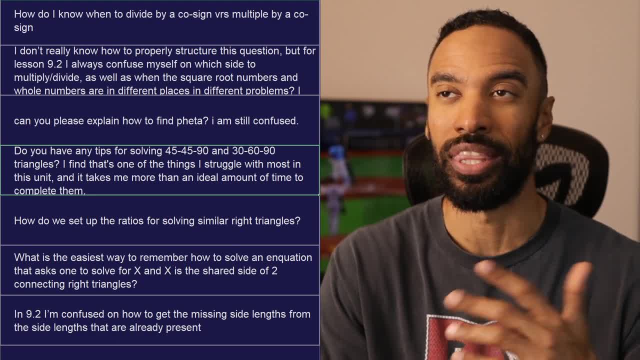 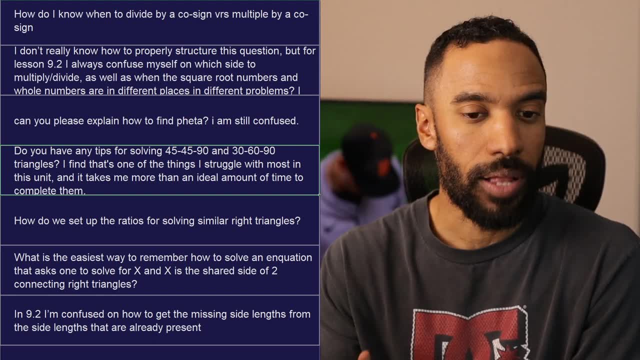 There are several questions there And I'm actually surprised there are more questions on that. Not that I'm surprised that people don't get it. I just feel like people often have a recency bias and would only focus on the trig questions. So I'm glad people are asking it and I hope I'm answering it pretty well. 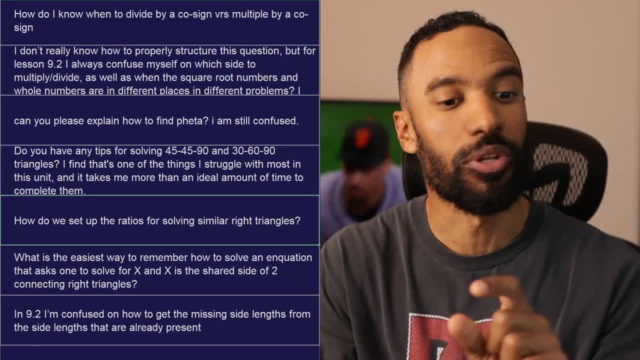 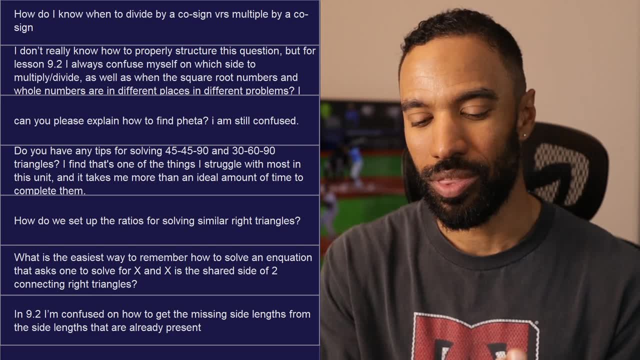 Okay, the next question is: how do we set up the ratios for solving? oh, similar right triangles. I thought this was special right triangles. again, I was going to say, and here's another question, We have a similar right triangles question, So this was out of 9.3.. 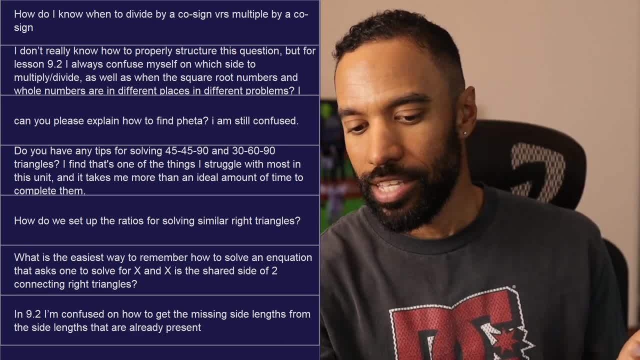 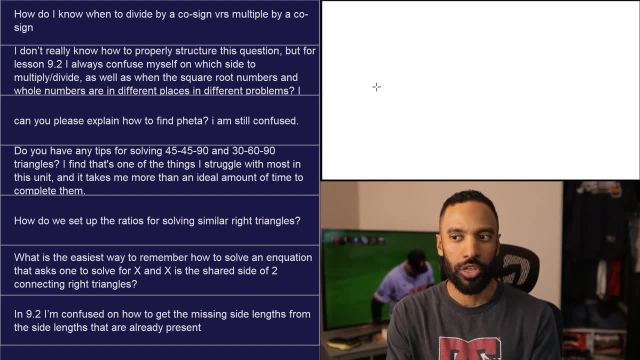 Yeah, it's something that you know. we spent one day on the notes of it And, although I only read the room in a nutshell of whoever's saying things out loud, I felt like we had a pretty good gist of it. That doesn't mean we still do. 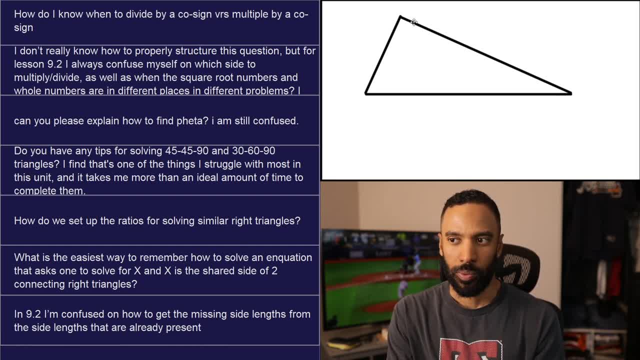 And that doesn't mean that everybody did, And that doesn't mean it's always the easiest thing, unless you're hearing it from the teacher, Like I've had many times, where I'll hear something from my teacher And I'll fully understand what they're saying when they say it. 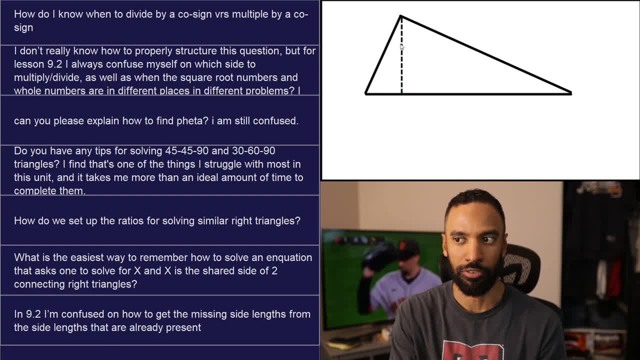 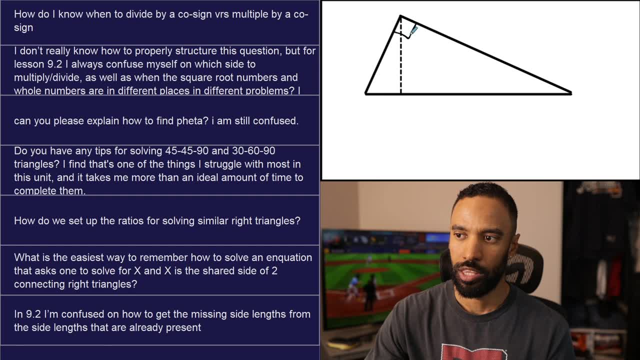 It's just that when it's time for me to do it for myself, I can kind of freeze up right, Like I can understand them doesn't mean I can do it for myself. Anyway, let's say: you have a right triangle right here. 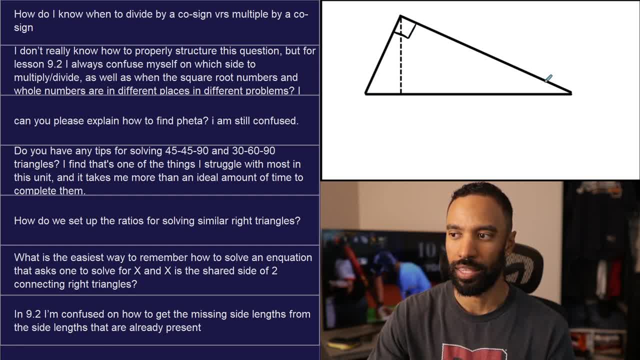 The big one right, Big right triangle right there. I now will draw an altitude to this hypotenuse. and then I construct another right triangle right there called the medium right triangle, And this guy here is the small right triangle. Clearly that means there's also a right angle right there. 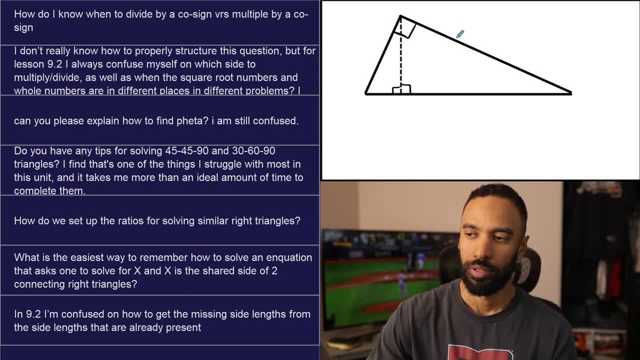 Right, They have their own. So there's big, medium, small. All of these triangles are similar in that they all grow proportionately with one another. I will give you letters with these things here, like that, And let's redraw them so they all face the same direction. 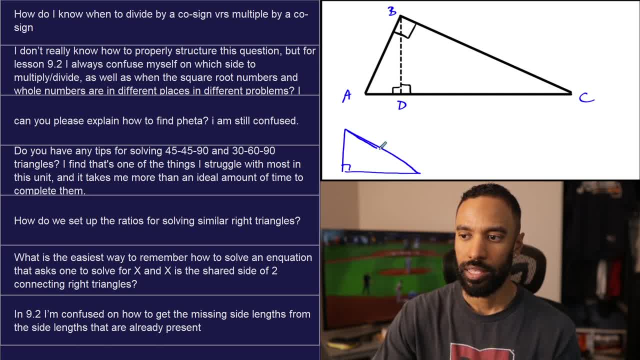 Let's start with the big one. Let's start with the big one. Here's what it's all about: Short leg, long leg, hypotenuse- Which ones are which? Where's the right angle as well? B is the right angle in the big right triangle. 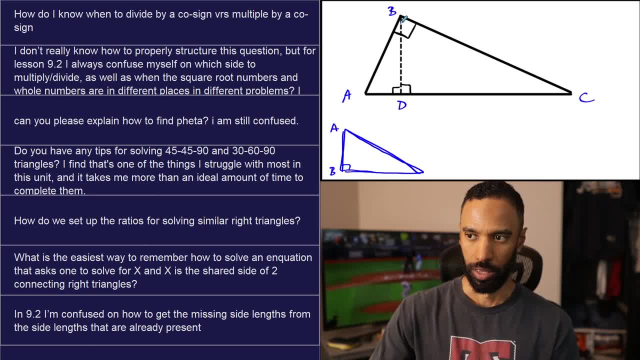 The short leg goes to A. The long leg goes from B to C. The hypotenuse is from A to C, Confirmed. Let's go to the medium triangle. The medium triangle's right angle is D. From D to C. 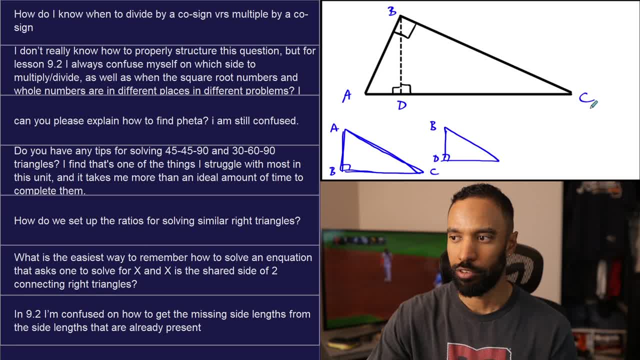 This is basically drawn the same way. From D to B is the short leg, From D to C is the long leg, From B to C is the hypotenuse, The small right triangle. imagine if you could rotate it downward. The small right triangle also has the right angle of D, in this case. 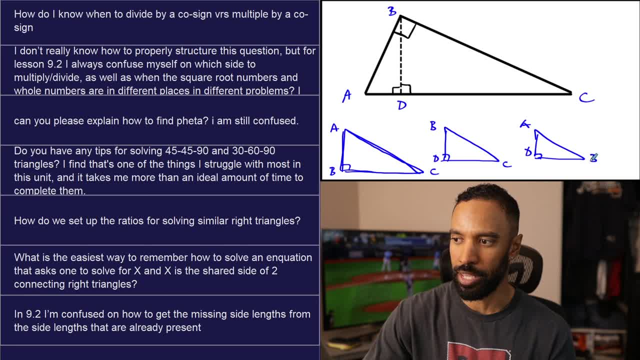 It has a short leg from D to A And the long leg from D to B And the hypotenuse is from A to B, like that. You asked: how do we set up the ratios, More so probably proportions. How do we set up proportions? 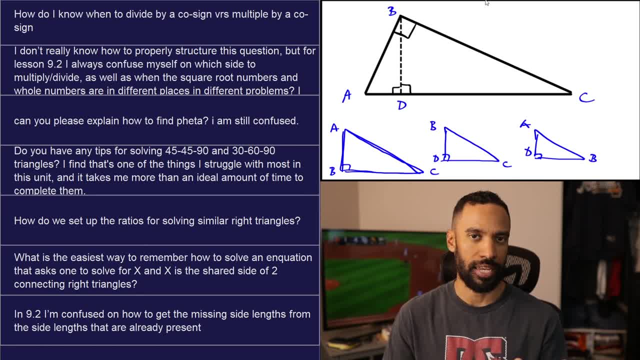 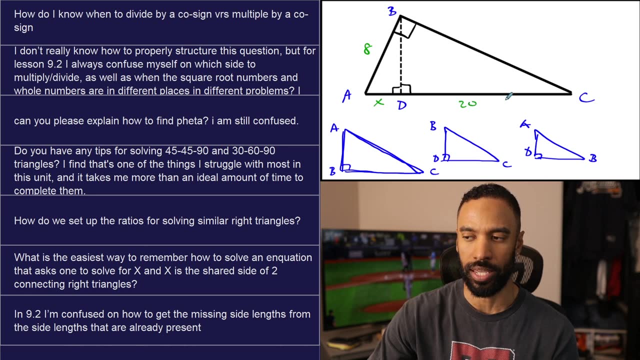 The reason I did the redraw was to reconfigure the idea that there's a short leg, long leg, hypotenuse, And the big, medium, small triangles, And that you can do this for yourself as well. So if you had information, if I knew that this was 8 and this was X and this was 20.. 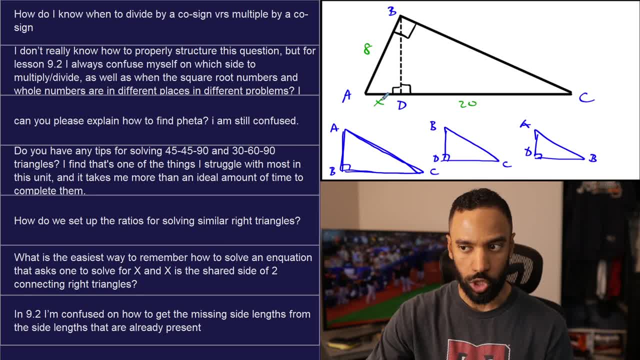 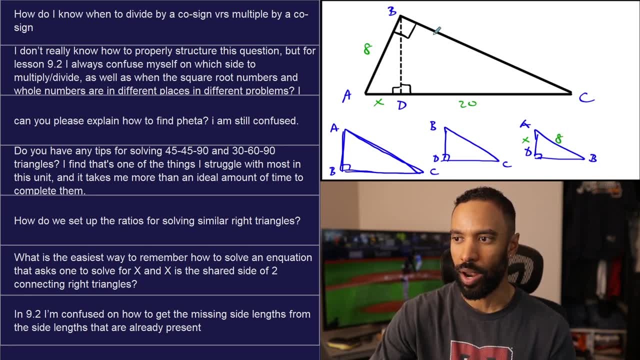 As far as my redraws go. look at the small triangle. I know that this short leg is X from A to D. Hypotenuse is 8. right there In the medium triangle, I only have this 20 as the long leg. 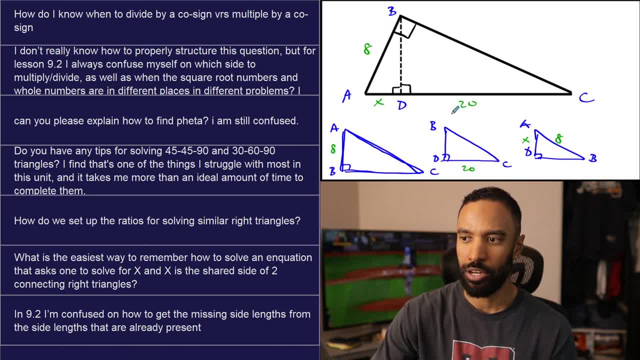 In the big triangle I have the short leg of 8. And the hypotenuse of X plus 20. Whoops, that's not the hypotenuse And the hypotenuse of X plus 20.. Why does this help me? 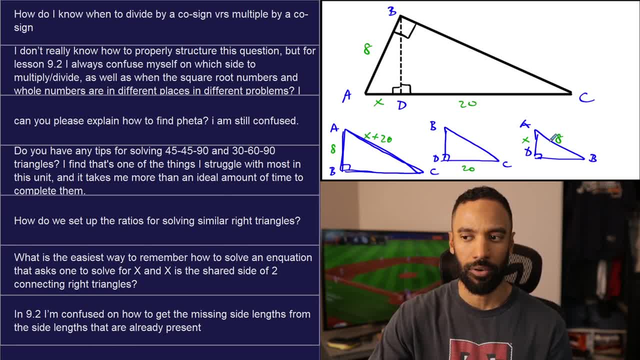 Because I can build a proportion with the big triangle and small triangle together. How come? Because they have corresponding parts And two parts known for each of them. The medium triangle not only has only one known part, But it's also a part that doesn't correspond to these guys. 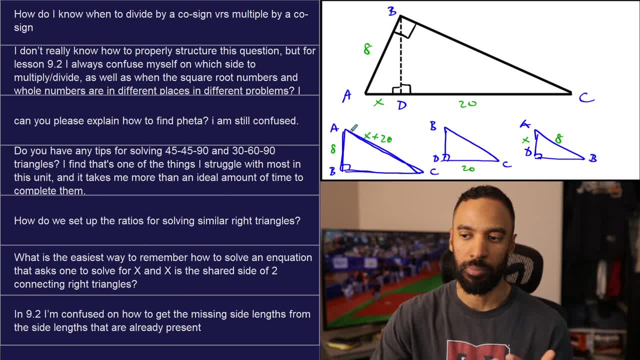 I have the long leg for it. I don't have the long leg for these, Whereas the small and big triangle, I have the short legs for each of them And the hypotenuses for each of them And I can do like: an 8 over X equals X plus 20 over 8.. 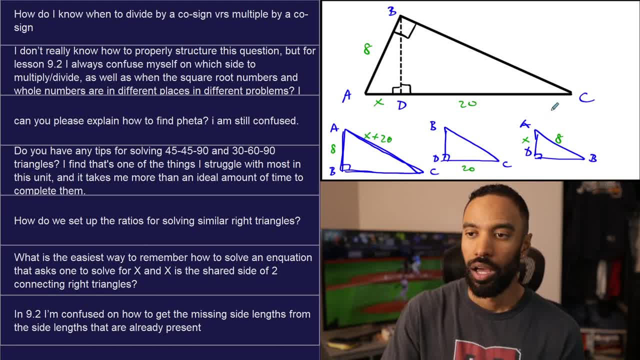 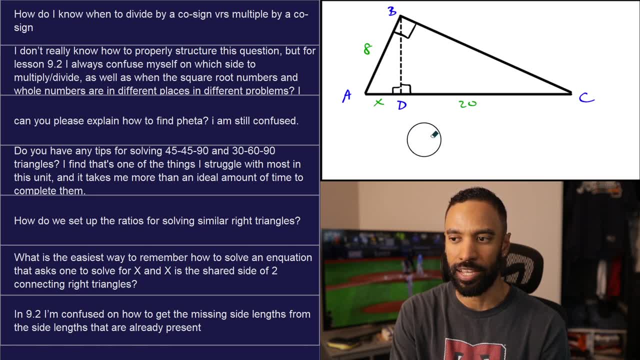 Something like that: How about we do it without a redraw? It's still the same thing, You have to ask yourself. You have to tell yourself that you do have to find X, Right? So you're like, okay, I have to find X. 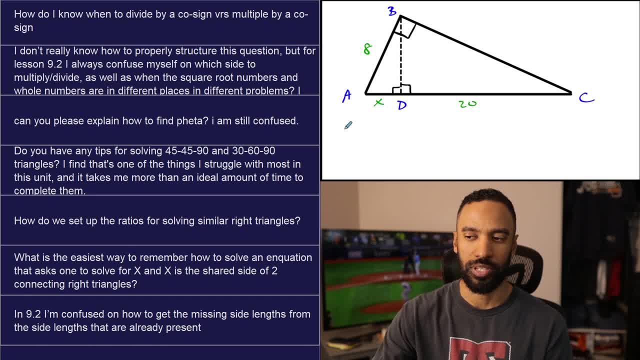 And I recognize what X represents in a part of my triangle. X represents the short leg of the small triangle, Short leg of the small triangle Right, Which means I need to also find the short leg of another triangle. Do I have one? 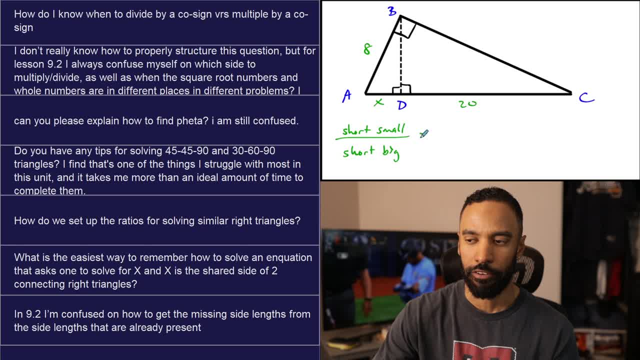 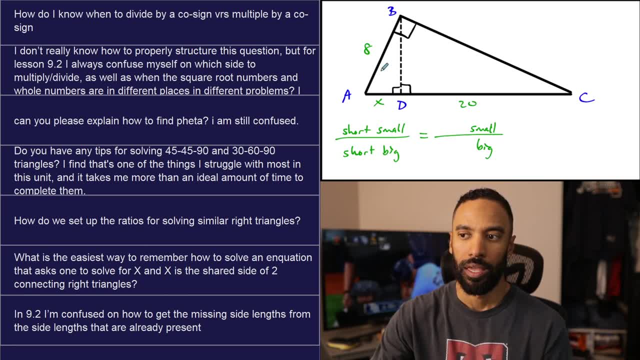 Not for the medium, I do for the big. Therefore, I need to do something else from small to big that correspond And hopefully this problem has enough information for it. The small in the small. I don't have the long leg. 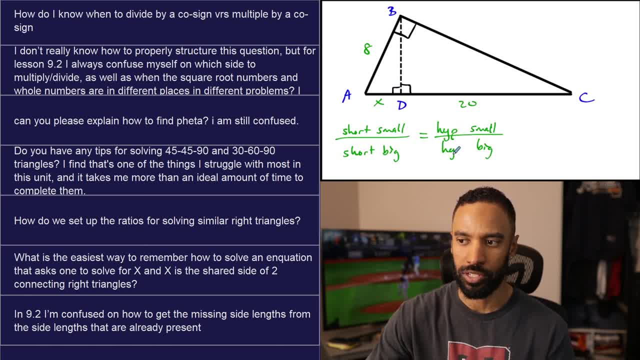 but I do have the hypotenuse. Do I have the hypotenuse of the big? I do, if you add X and 20.. Yes, So I can come up with the thing there. So short of the small is X. This is the part I don't always write. 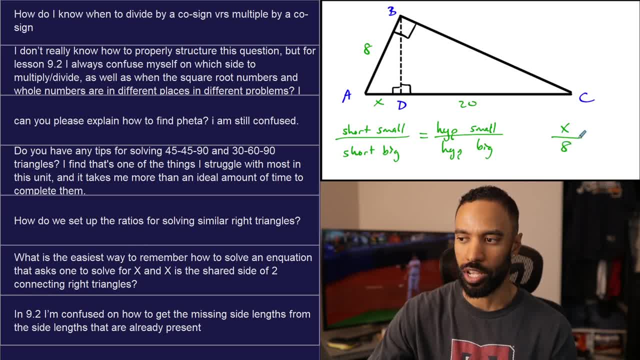 but I say it out loud: The short side of the small triangle is X. The short leg short side of the big triangle is 8.. Hypotenuse of the small triangle is 8.. And hypotenuse of the big triangle is. 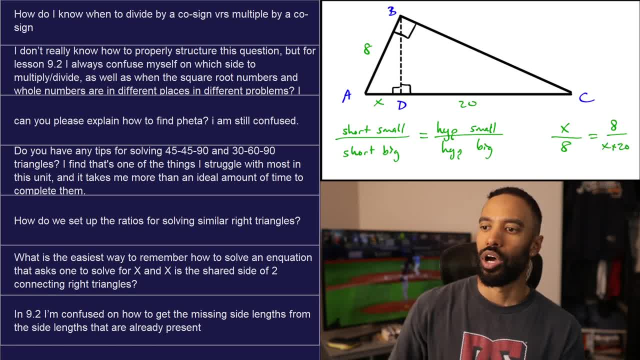 um X plus 20.. So it's that kind of thing that I do, uh, that I call out Generally: you want to identify what your variable is, what parts it represents, if more than one, because it can, as you could tell. 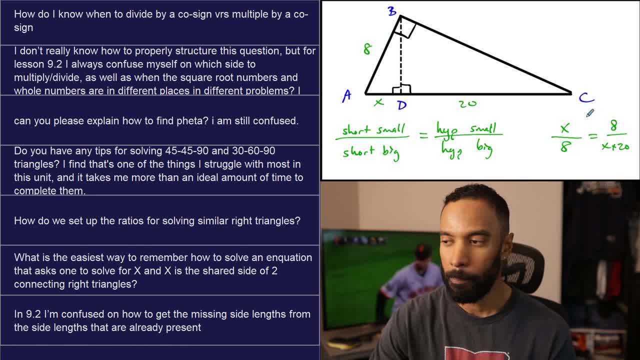 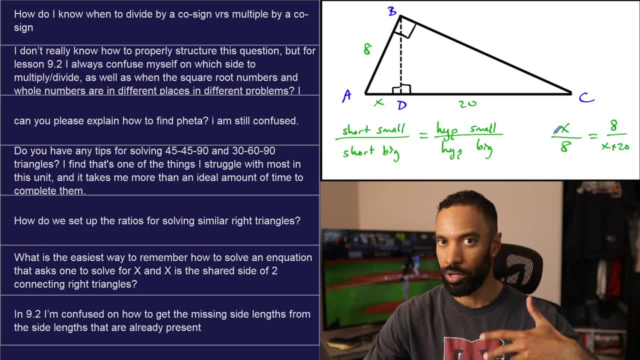 eight represented two different things: The short leg of the big triangle, the hypotenuse of the small triangle. You do have to not only correspond parts like short leg, short leg, hypotenuse, hypotenuse, but you also have to go in the same order. 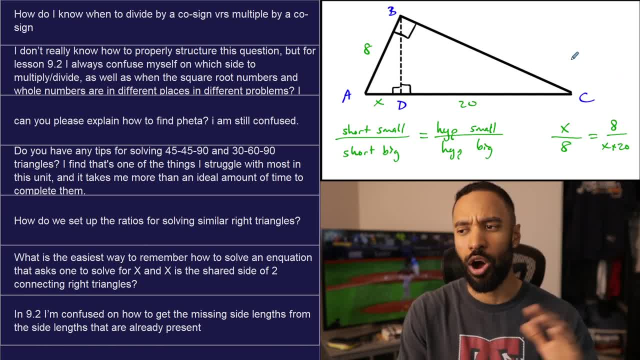 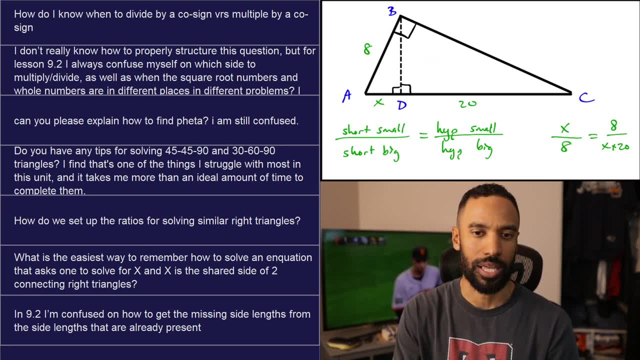 the same direction. small to big, small to big. Um, you do it. That's the idea. You have two different forms. I recommend triangle redraw if that helps you, because it's all about triangle similarity. but that's another example of that. 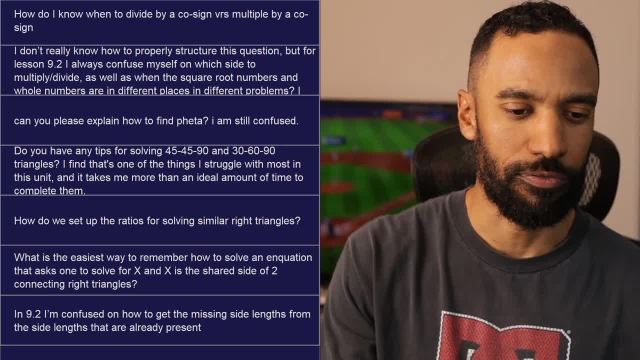 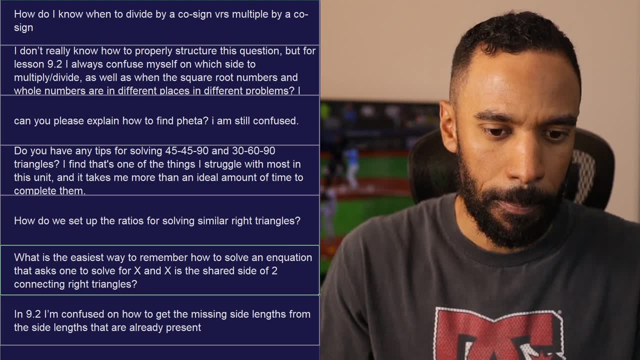 And I'm glad someone asked something in 9.3.. Awesome, All right And move forward. I think we have two more questions. What's the easiest way to remember how to solve an equation that asks one to solve for an X and X is the shared side of two connected right triangles? 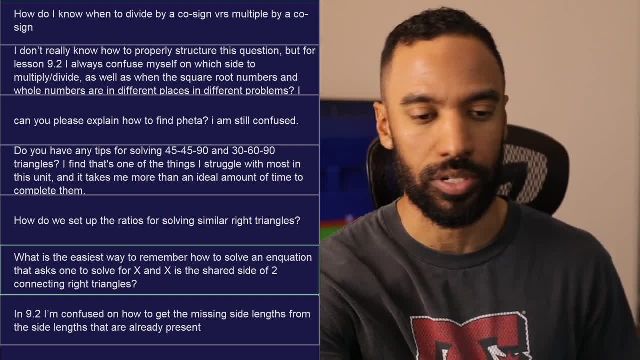 Oh, it's another. it's another uh question, Like it's another 9.3 question. So what's the easiest way to remember how to solve an equation that asks to solve for X? It's the shared side of two connected right triangles. 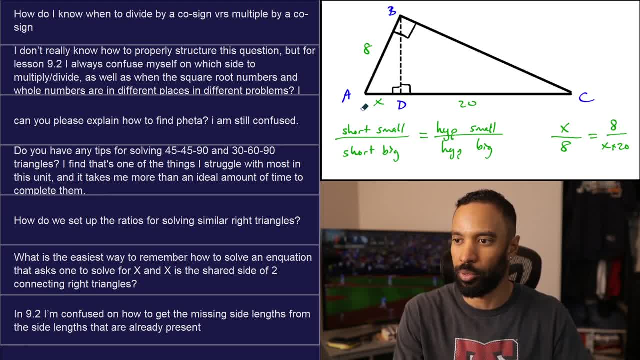 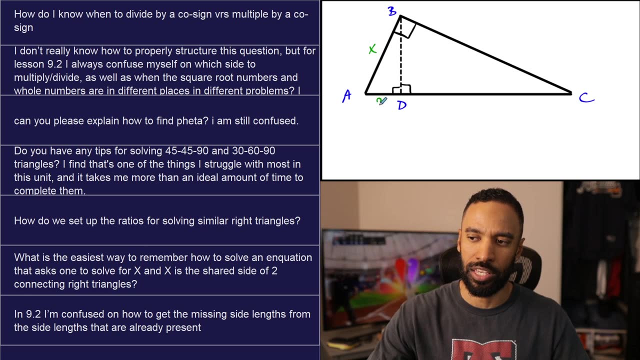 Um, so the? uh. this was not an example of that in perfectly. only because the X was not the shared side. In this case, eight was a shared. Oh wait, is this what you meant? I guess X, like if this was X and this was eight and this was 20,. 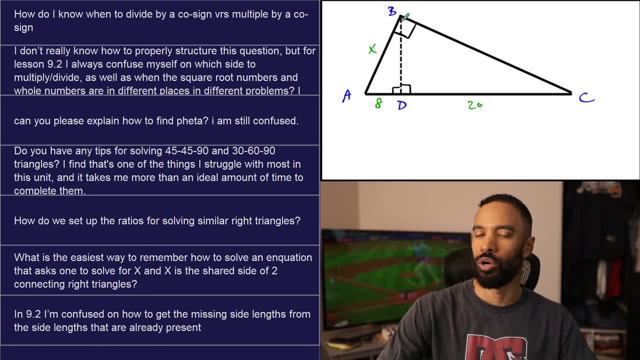 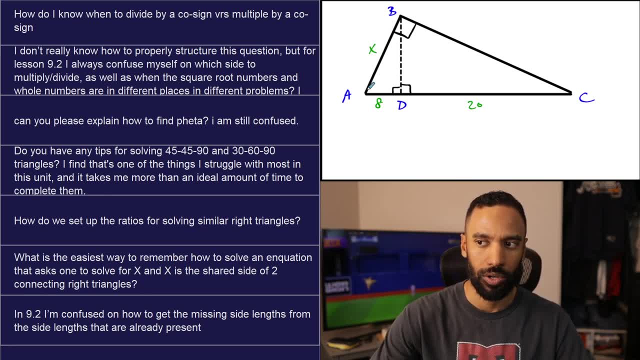 just flipping it around, whatever, Um, you know the. the thing that I generally do- and I I do this a lot before- is I first identify what where X is and what it represents. And I asked myself: do I? 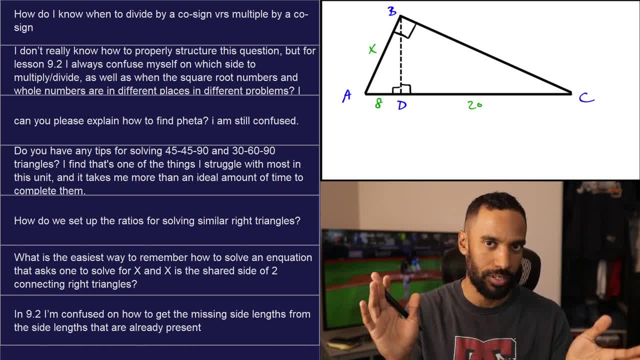 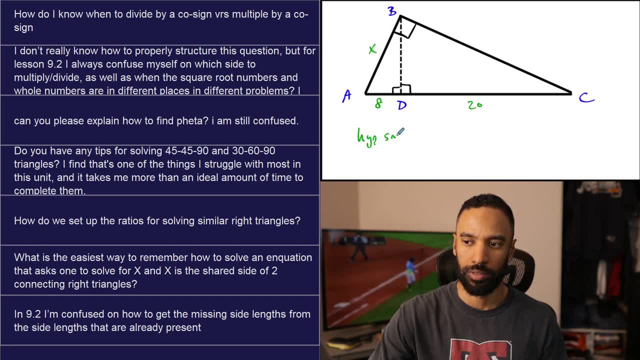 could, could I use it? or, you know, do I need to use all forms of X in this part of the problem? for it I, in this case, I will, but X represents the hypotenuse of the small triangle, which means I'd have to find the hypotenuse of another triangle. 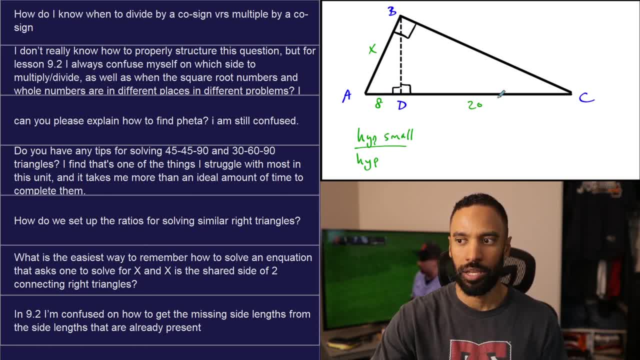 the medium or the big. I don't have enough information in the medium, The biggest, eight plus 20.. So I do have that. So I'm hoping I have something else with small and big to represent. uh, with small I have the short leg and the high pot. 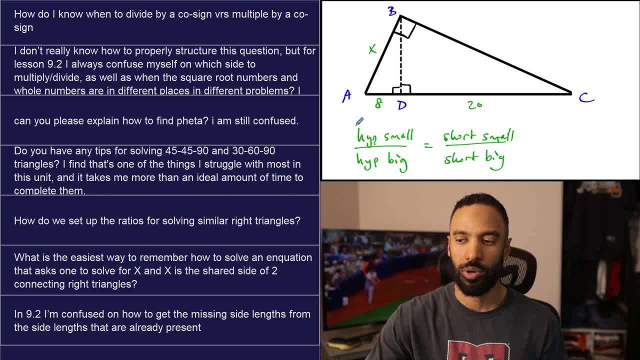 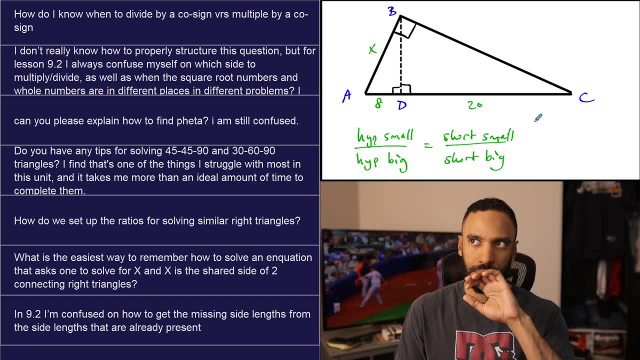 the big triangle I have the short leg as well, which happens to be X again. So X represents both the hypotenuse of the small triangle, short leg of the big triangle, neither would, which would correspond with each other, meaning they would never be divided with each other. 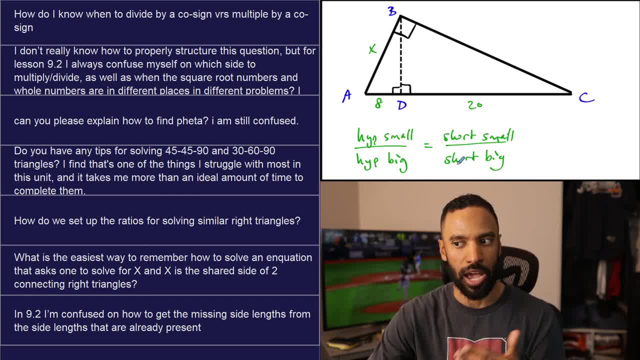 They'd never be on the same part of the fraction with each other. They'd actually be opposite each other as to cross multiply in that way. If X is going to be used like that, So I don't know if that kind of addresses that. 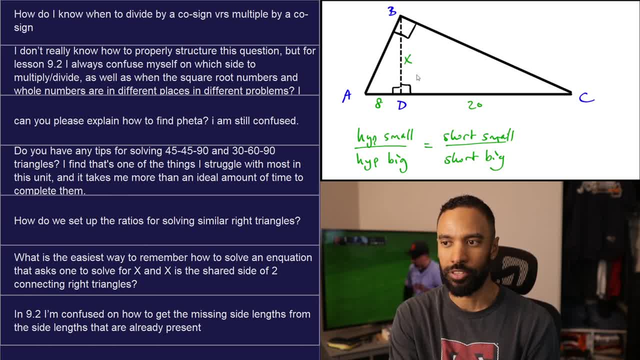 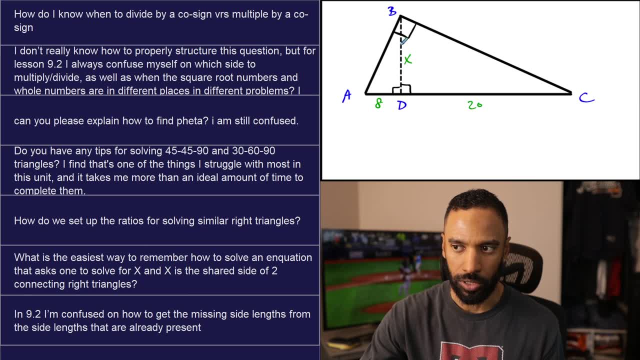 but there's an example there. Uh, the other forms that we'll have is when X is the altitude right here. Now. X represents two different things: X is the long leg of the small triangle and it's the short leg of the medium triangle. 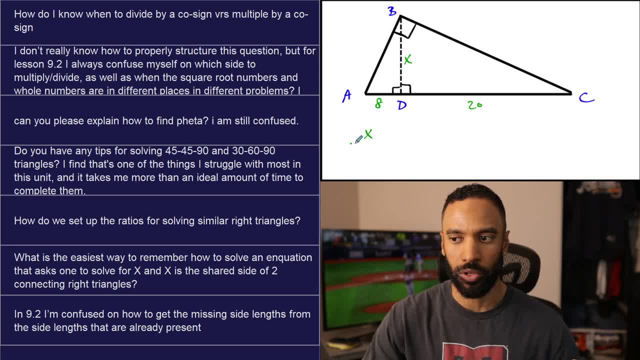 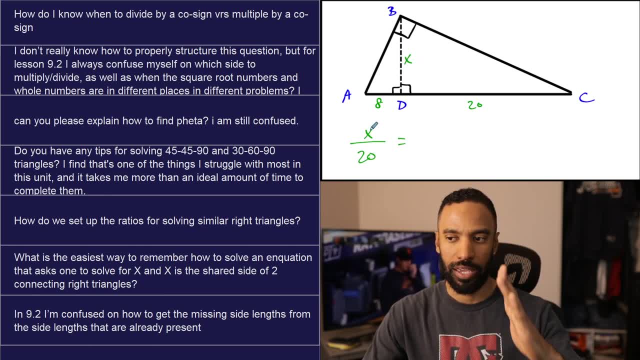 So when the long leg of the small, I also need the long leg of another, the medium triangle I have and it sounds like I can use the medium again for X. So the long leg of the small over the long leg of the medium equals. 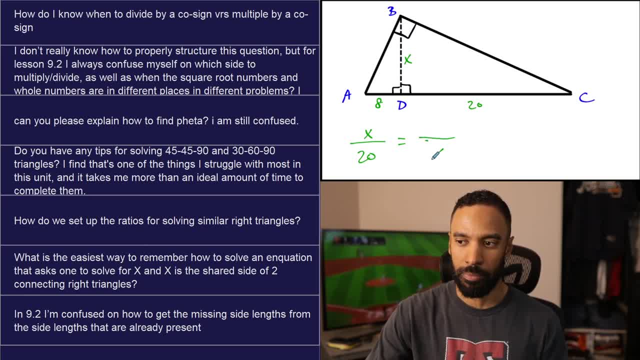 Now let's do notice how X is the short leg of the medium and I can use that in the short leg of the small, is right there And there's another setup, you know like that, And then the last one that's set up when 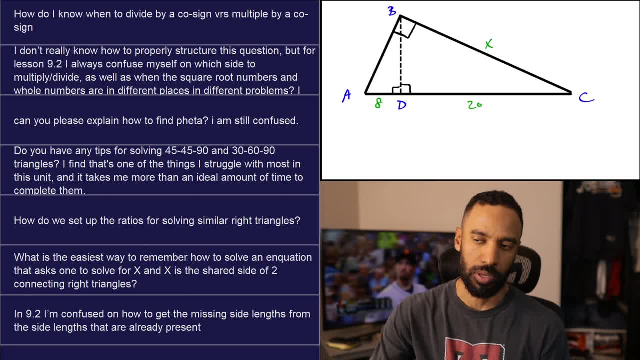 cause. you said shared side, So the last one that we could set up is something like this: Now X is in the big triangle as the long leg, And it's also the hypotenuse of the medium triangle, but it's the long leg of the big triangle. 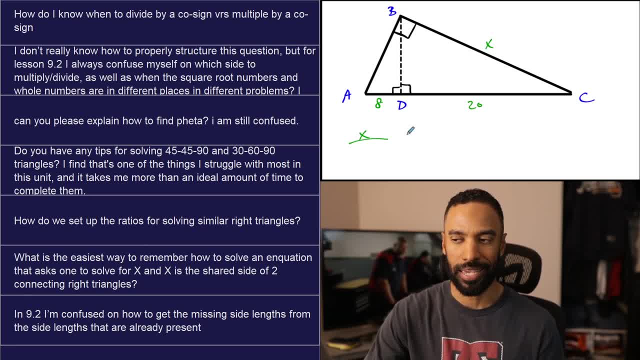 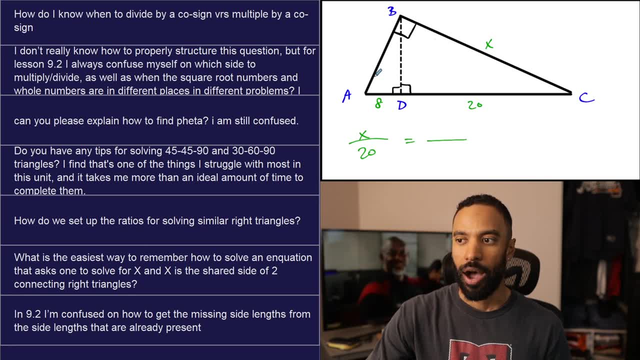 Do we have the long leg of another triangle, Not the small but yes, the medium- right there. So we have something else in the big and medium to do: Hypotenuse of the big 28, because we don't have the short side. 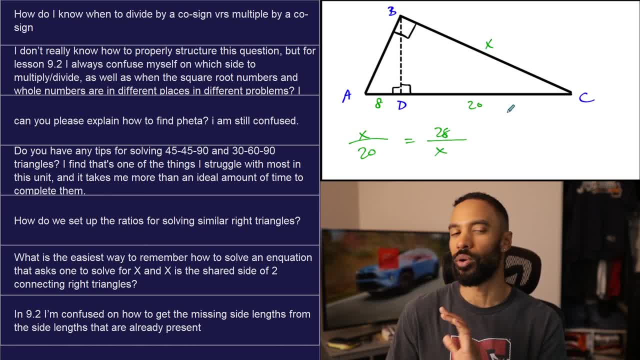 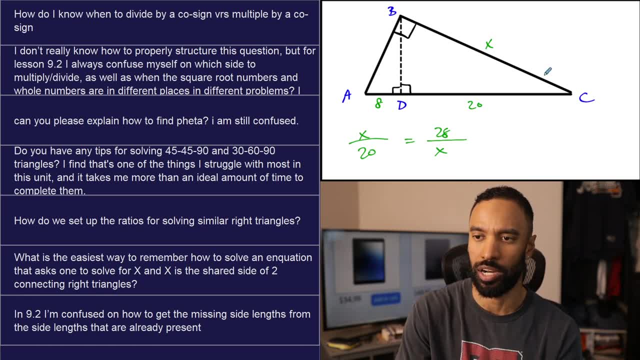 And then hypotenuse of the medium X and X, just so happens. Remember you don't have to use X multiple times in this question, You do. There are some questions where X might not have to be used multiple times and just kind of keep that in mind when it's set up. 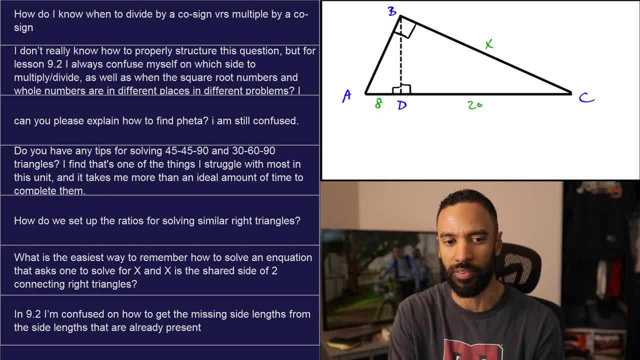 But that's how it's used. I mean, I talked about the proportion stuff a little bit more in the previous question that was asked, So maybe you can combine the two and see if you get your answer in full based on that. Okay. 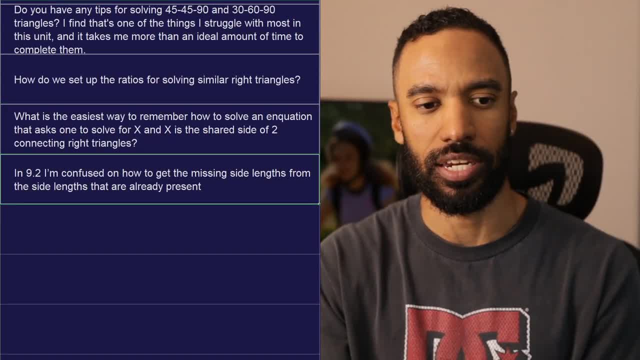 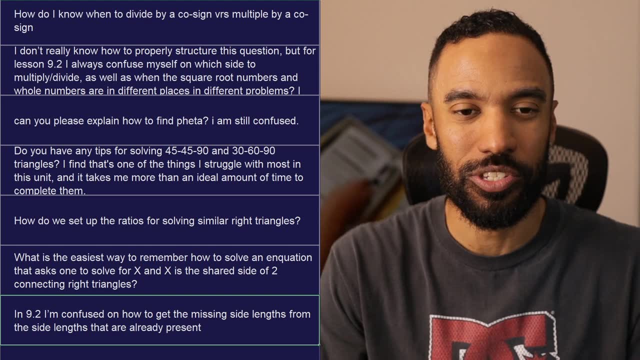 And I think yeah, the final question being asked is in 9.2.. I'm confused on how to get the missing side lengths from the side lengths that are already present. I hate to do this to you, but I did. I did answer it. 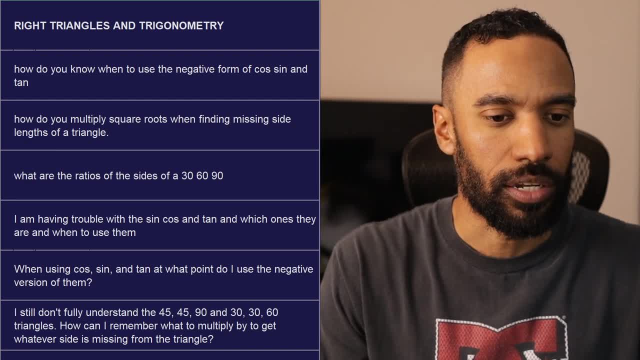 If you want to check out other questions, I'm going to point to them all. I'll be helpful. We can find this question. Find the timestamps in the description section, but find this question here. Anything on 3069,, your special right triangles.